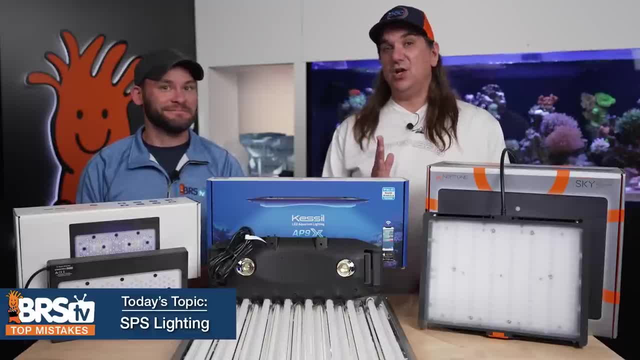 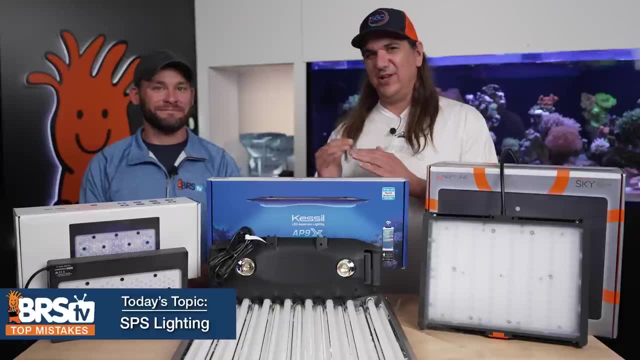 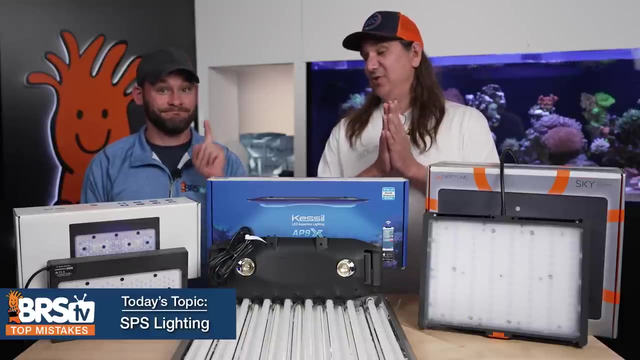 All right. today, new angle on a different topic: Top 20 mistakes on SPS lighting- Big ones. Let's refine the information down to the application rather than giving it to everything to everyone. So today, if you're an SPS nut and you want to know how to use lighting, this is made for you. 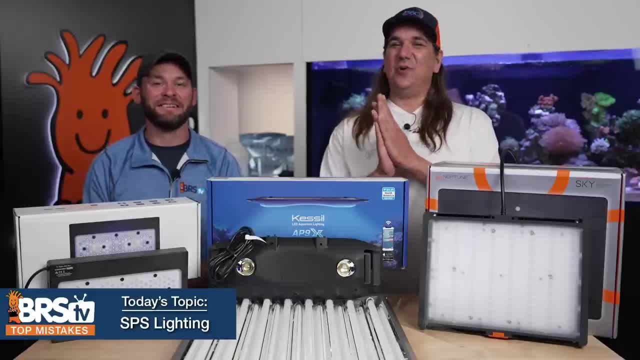 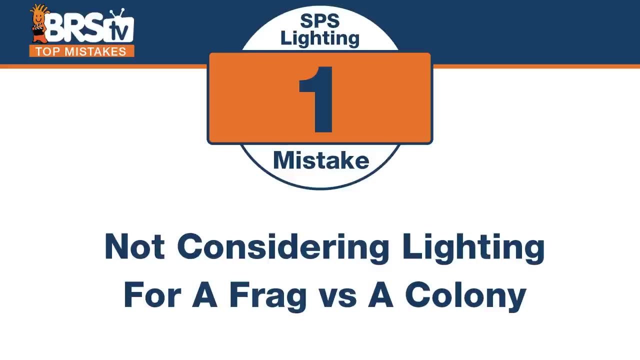 Everybody else check out, because we've got one for you later, But we're going to find out, So starting with number one. Number one is not considering the lighting, or making the mistake of considering the lighting for when your sticks are a frag versus when they're a full, giant colony. 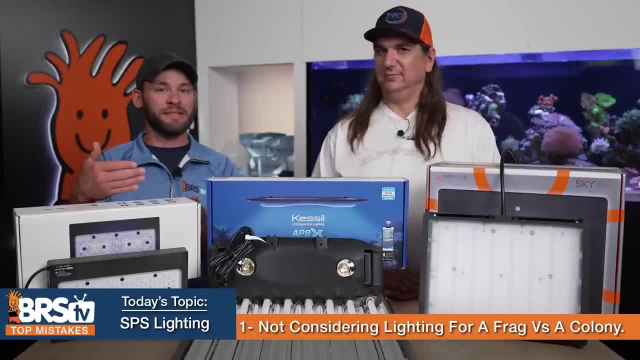 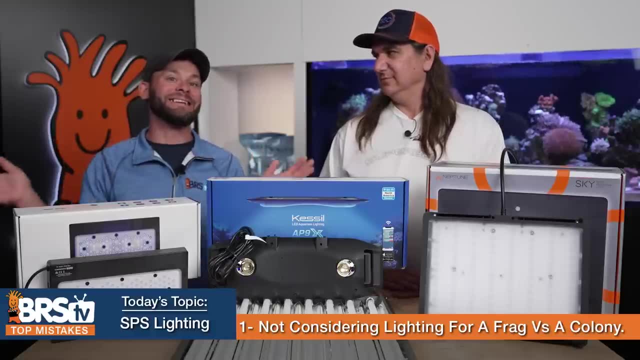 And there's ways that you know you can grow the light with those needs, as long as you recognize that those needs for lighting from a frag or mini colony to full colony completely different. I think this is like. if there's one thing you heard today, let it be this: 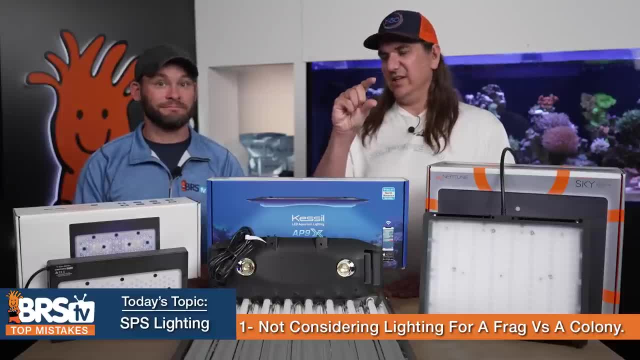 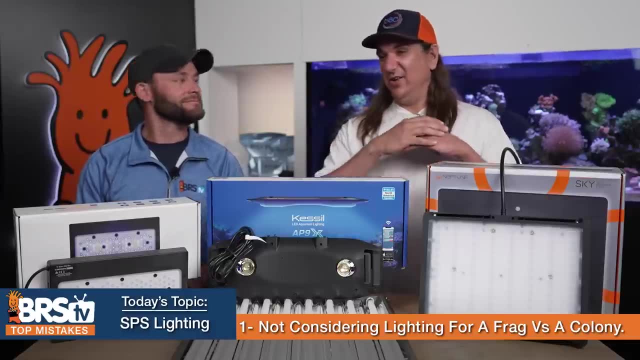 The needs of a tiny little coral this big It doesn't shadow itself and is super easy to light. doesn't shadow its neighbor, doesn't do anything. It's just an array of them, man. It's really, really easy. Almost anything could do it. 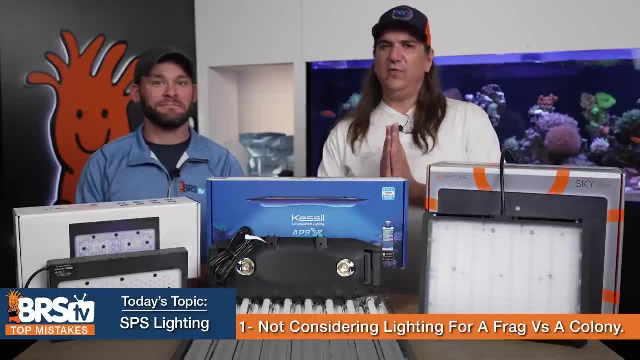 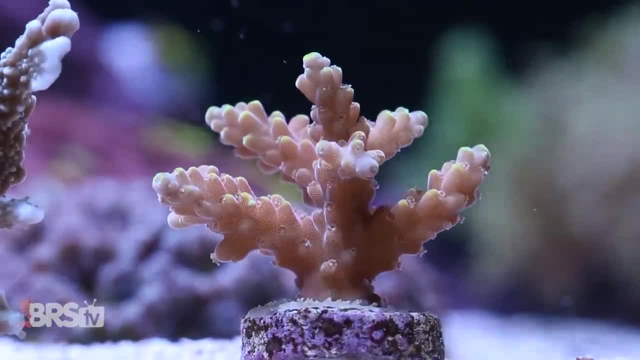 But the goal isn't really that, And the trick here is that, well, if it worked for the first 18 months, you're not going to know that it doesn't work for the following few years, until you start killing stuff. Yeah. 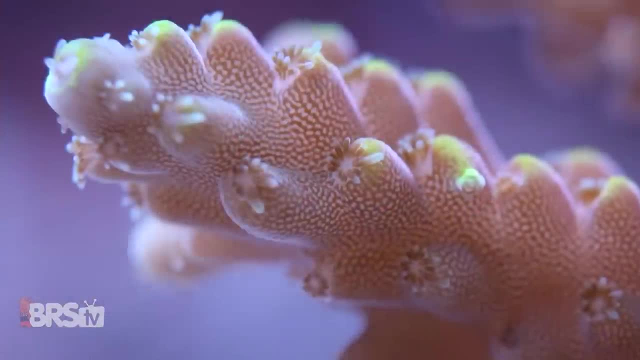 Unless somebody told you: All right, You're going to hear today exactly what that is: A bunch of tips for SPS lighting, And it's going to be a lot of fun. None of this is about I bought a one-inch frag. 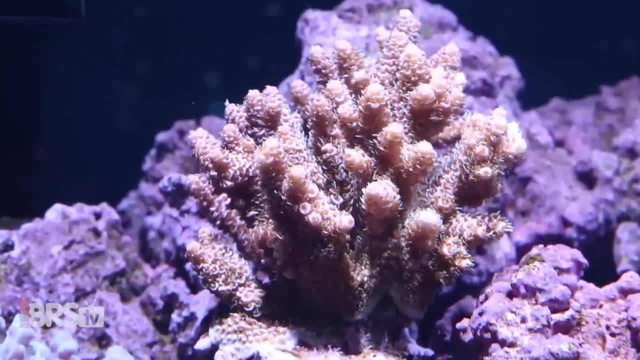 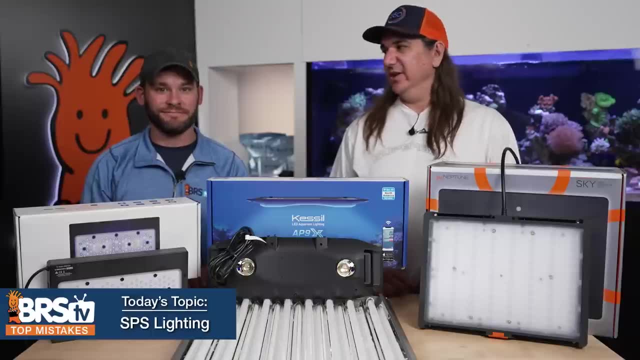 This is about how do I grow massive, healthy colonies. So in that spirit, number two, I just don't think this has been said enough, even if you've heard it. Yeah, the mistake is not understanding how a coral shadowing its neighbors really matters. 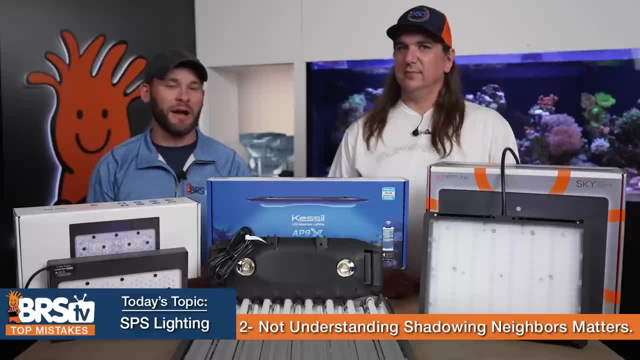 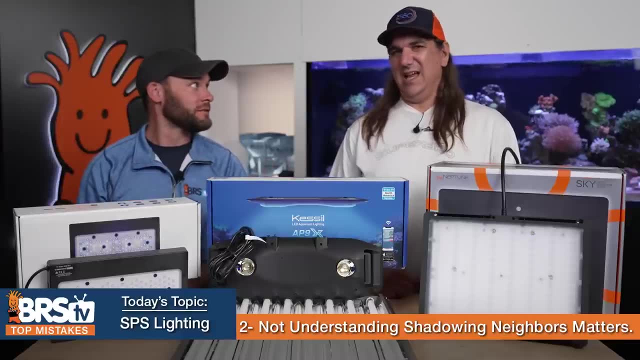 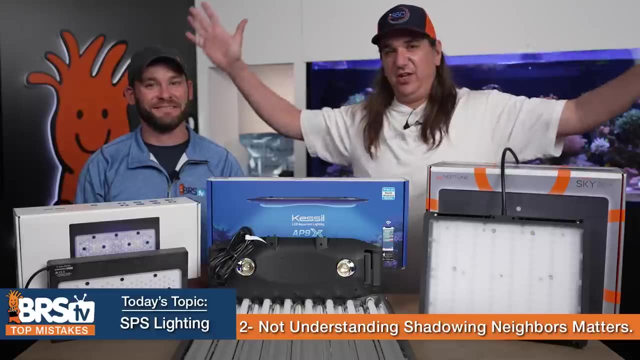 And I think you say it really well when you're talking about. you know, how much percent of energy am I getting from the light when I'm fully exposed to light versus when I'm not? I'm behind something else. Yeah, this is one of those things that was missed when we shifted from T5 lighting, which was this big and covered the whole thing, blanketed it from all possible angles. 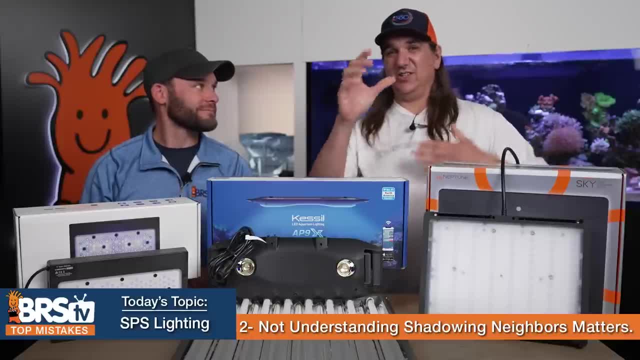 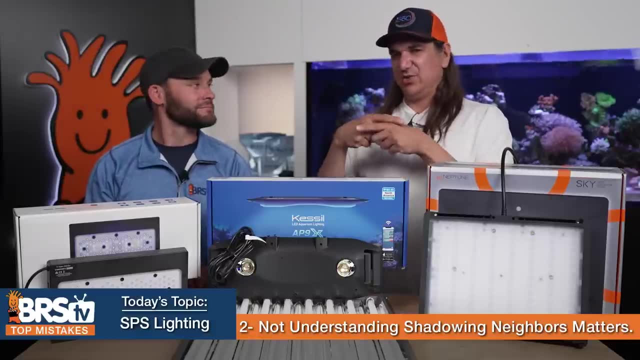 And even halides, which looks like a little bit light, but it actually is coming from a giant reflector And you know 50% of the light is coming back down this way. And then, when we shifted to tiny little, small form factor lights, what we did is, if you can imagine- you know, I got a coral over here and the light hits here- 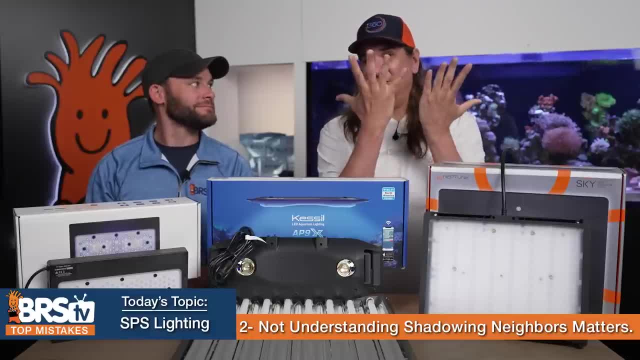 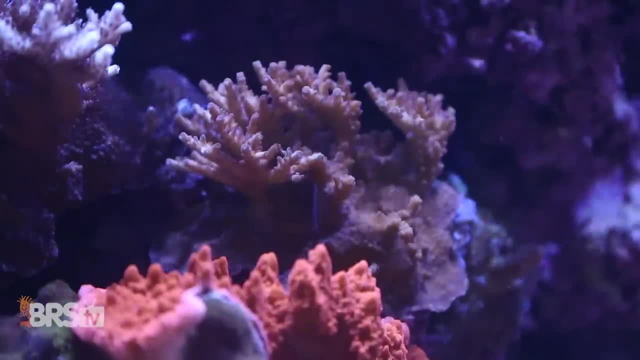 This one is now shaded. When they were this big, it didn't happen. When they're this big, it did, And so that's why a lot of people struggle And they don't really even know why. They don't know why the bases of the coral is dying. 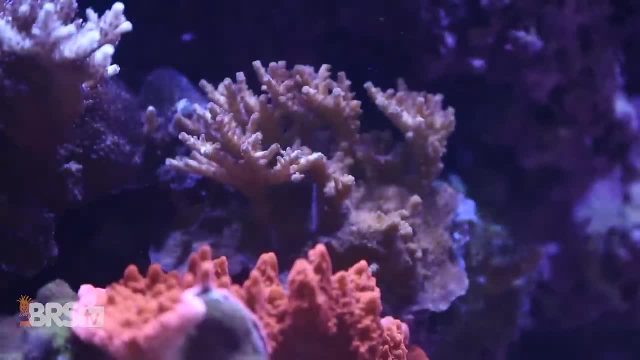 They don't know why the neighbor, like this coral, is doing so well What happened? And you don't even, like you know, there's some things, until you hear it aloud. you just don't know, But like you know what. 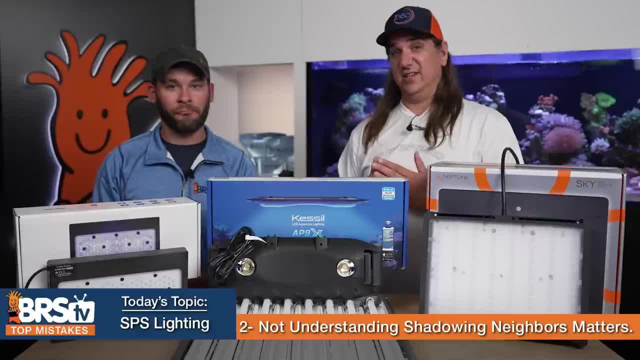 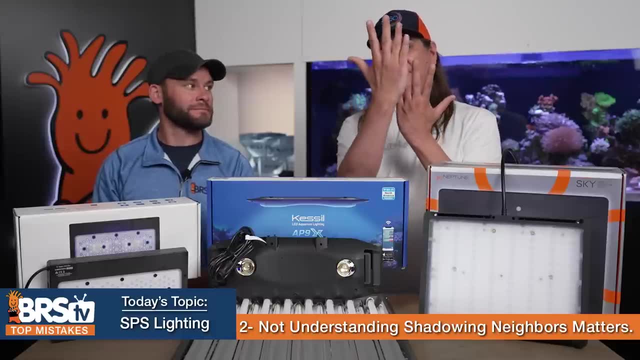 This, like organism, thrives off of light. It's 90% plus of its energy for metabolic function and growth from light. If I shade Half of it, it's getting half the energy And it's not necessarily like just going to kill off this part. 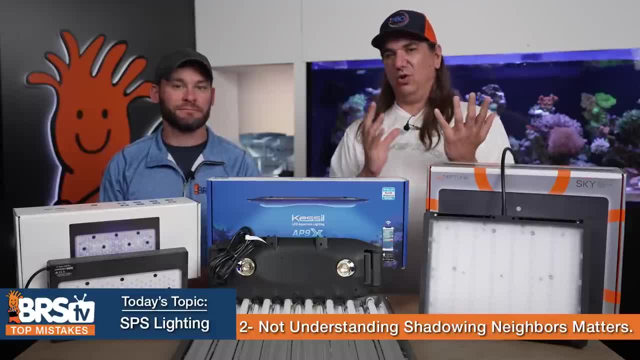 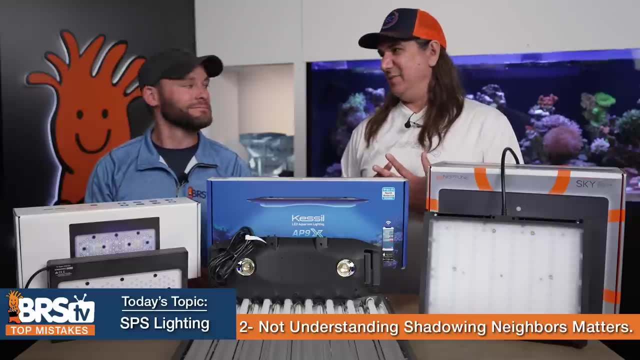 It's actually spreading that energy throughout the whole coral, And so the whole coral can be affected in its health, its ability to fight off pests, to survive stressful events. So you know, if there's one thing again, I mean this is going to probably sound redundant because all this stuff is so important. 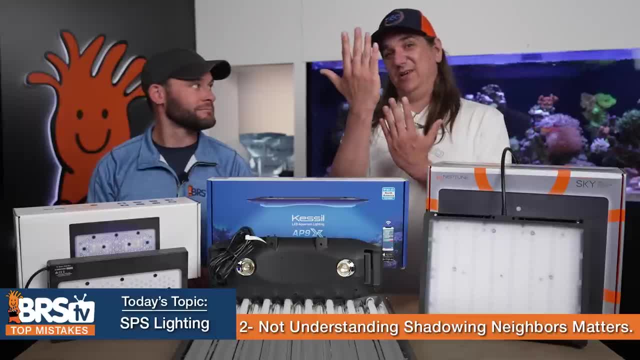 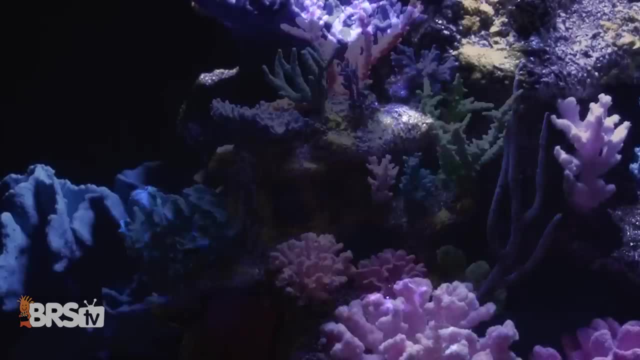 There's one thing here today, man, Let it be that shadowing is important and it comes from small form for their lights. If you only have one, if you have a bunch of small for it, So far Small form factor lights actually intersect and you can create the same thing is a big light. 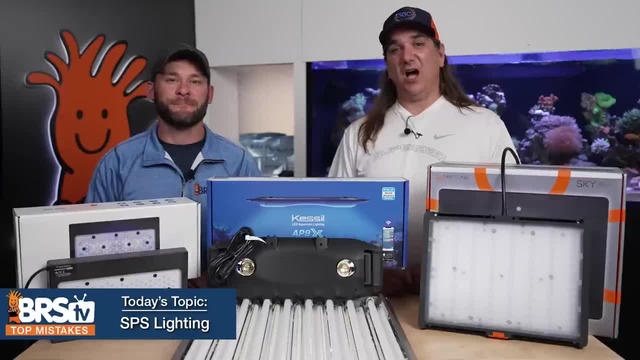 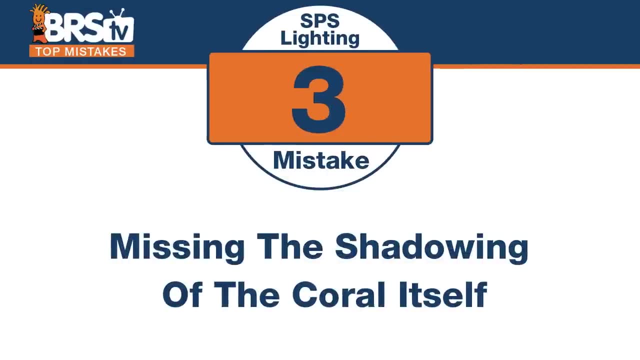 But look for those shadows because they matter. Number three: Another big difference between this little guy and these- And the mistake is missing- the shadowing of the coral itself. So you know, as it's a mini colony or whatnot, there's light getting all through the inside and there's no problem. 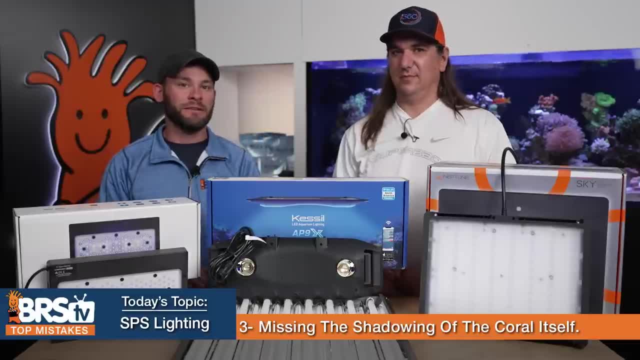 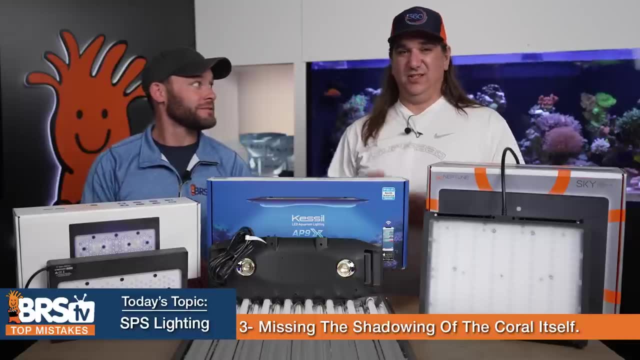 When this thing turns double, triple or what have you, and you'll start to notice there's dead spots with inside of the coral And that's something that we need to manage. also, You'll notice that it's not basing out. The base is actually shrinking. 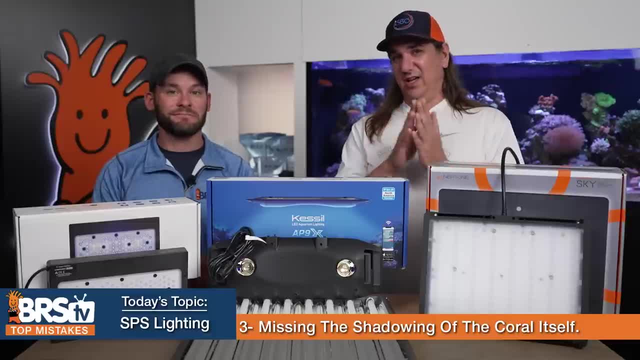 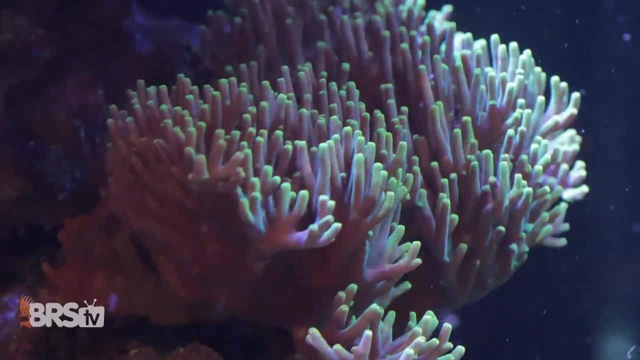 You'll notice that the inner working of your, like Piscillopora or your bird's nest, is all dying. And again, you know when we had these big giant lights, you know it wasn't dependent on a beam of light coming here. 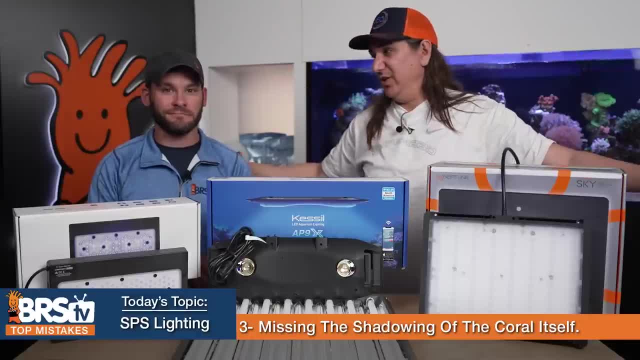 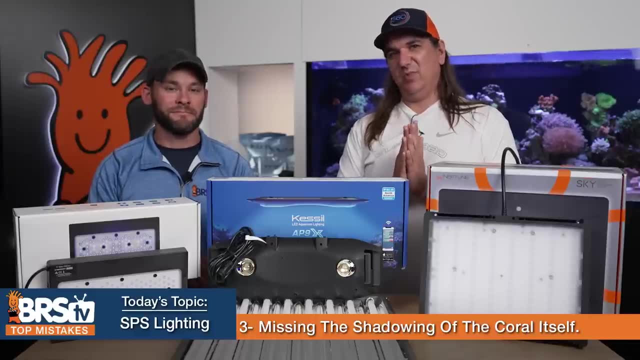 It was coming here, here, here, here. It was coming down all from you know, everywhere, And so we're trying to create that thing. Now we're talking wall to wall SPS Light's here today, Like I'm not talking about trying to grow a handful of zoanthids somewhere in the tank. 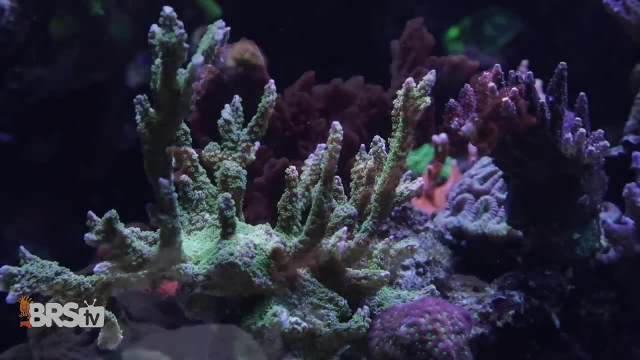 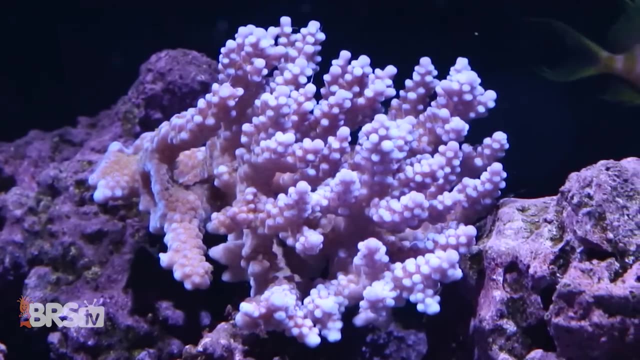 Yeah, like you're going to grow an epic tank And to do that, you really need to consider this thing: that this coral shadows itself and it does die and it will shadow those neighbors. If you solve that, you won't have that problem. 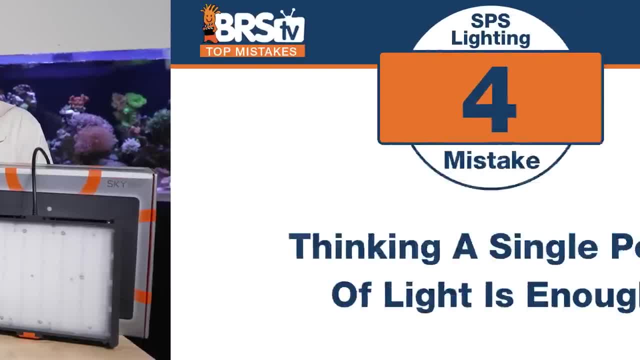 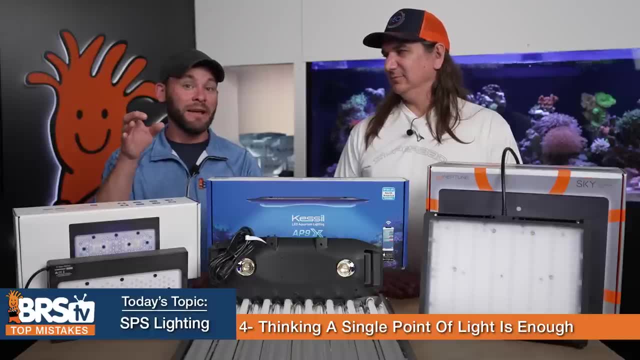 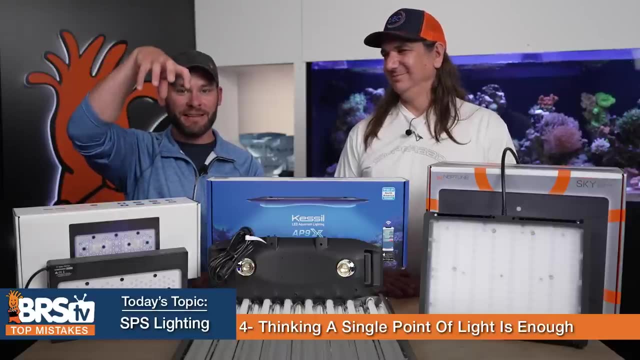 Number four: we're really going to bring this up. The mistake is thinking that a single point of light is enough for an SPS or SPS dominated system. It very well might be if you put a single SPS frag that grows into a colony directly under that light, and that light is hitting it at all sides. 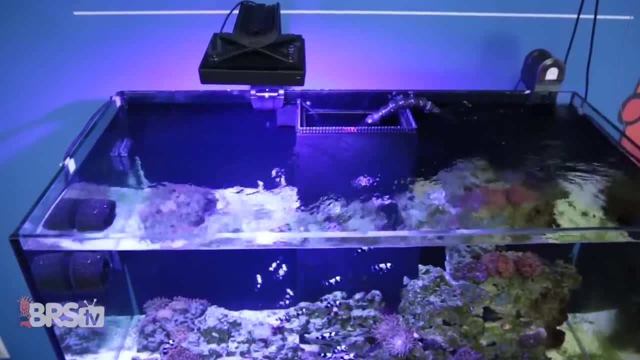 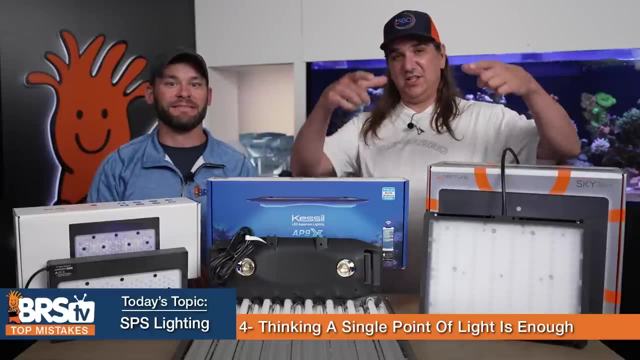 But we're talking about lighting an entire tank, whatever the dimensions. those single little points of light just aren't enough. So you can get away with a single point of light, but you're going to have lots of them, And so you just think of it as like a cone that will be blocked. 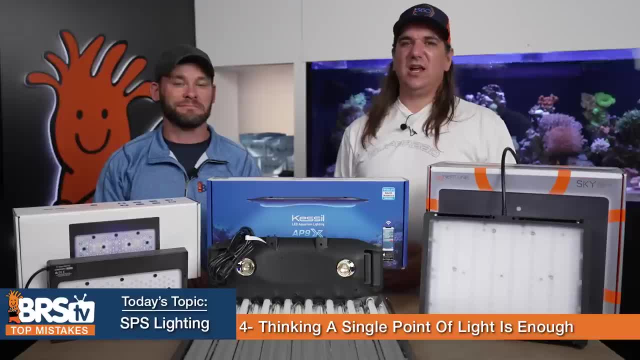 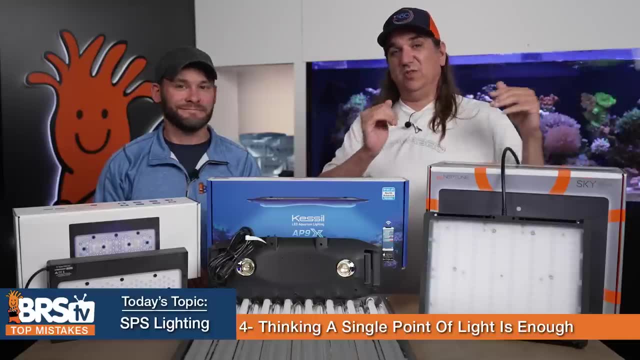 But if I have another one over here, it won't be. However, a lot of times that you know, like the manufacturer will say, covers a two foot area. Well, really, to get those intersecting cones of light, especially near the mid range and the top of the tank, they actually need to be closer together. 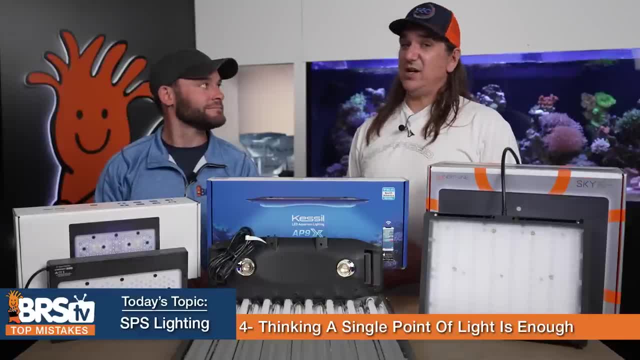 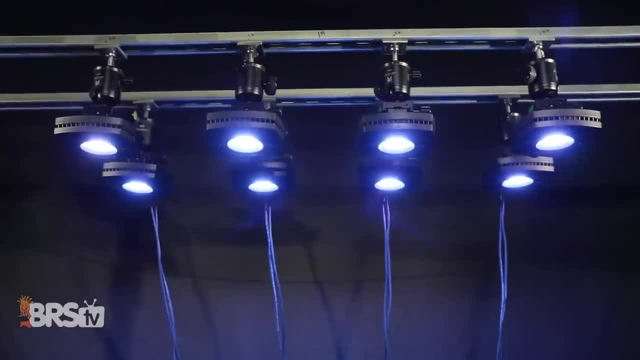 So often 12 to 18 inches, depending on the light. We saw actually a grid of AI primes which is like on a 120.. We saw a grid of six or even a grid of eight, where one single AI prime is covering a one foot area. 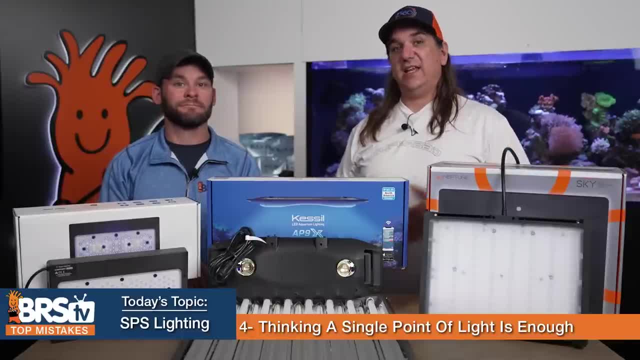 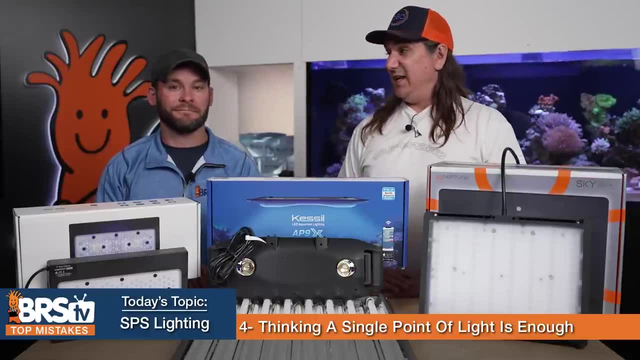 There's so many cones of light in this case that you created that big coverage And essentially you know covering it end to end with a blanket of light with all the little form factors, and then you know like oh whoa, eight lights. 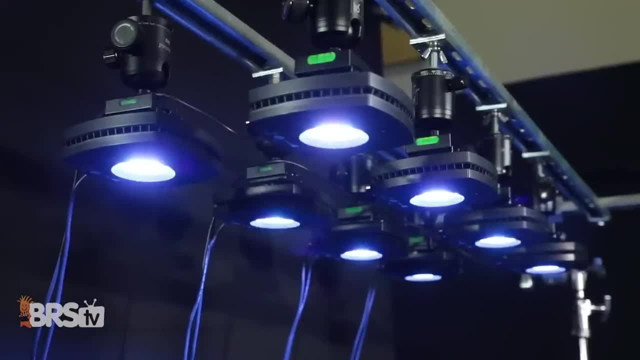 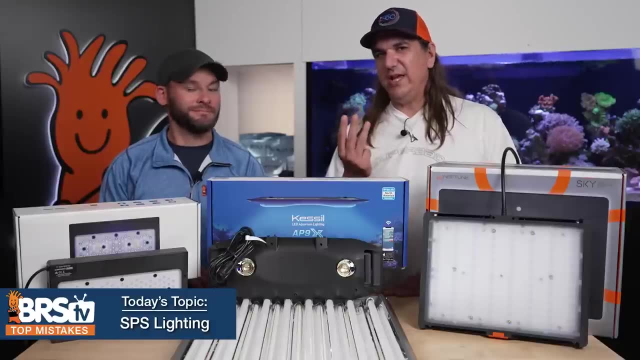 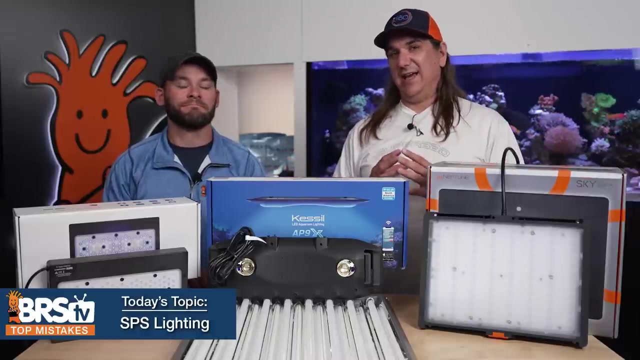 But you know what? It's actually cheaper than doing many other solutions And it does it better. Number five: there's actually three ways to get this blanket of light in the tank that's going to grow, that epic SPS tank, And I think the mistake is not understanding that there's three different ways and all of them. 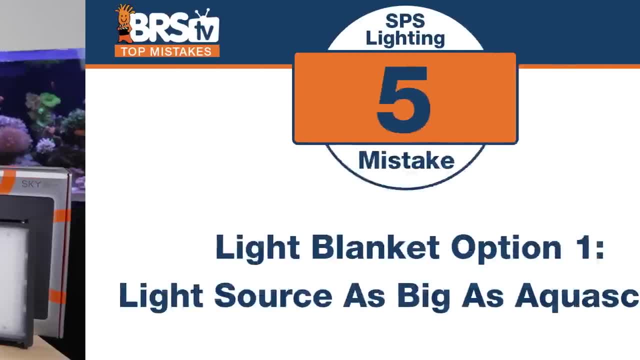 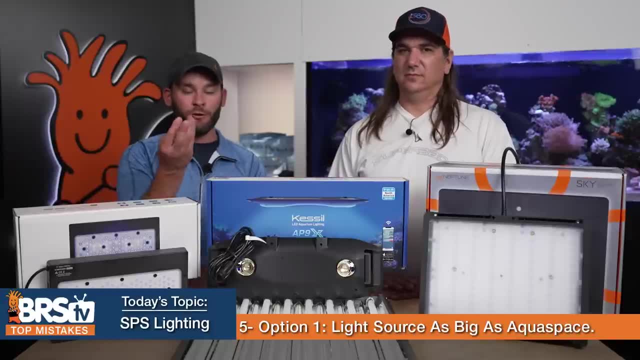 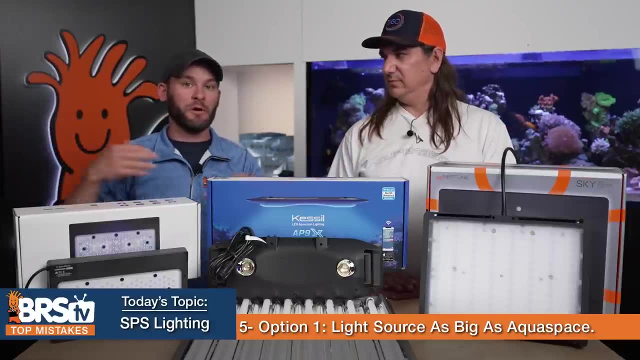 We'll lead to the same path. So the first option is making having a light source that's just as big as your aquascape or what you're trying, Bigger than what you're trying to illuminate. Illuminate meaning this: Corals, you know, only four inches by five inches, but my light source is twenty four or forty eight by 18 or what have you. 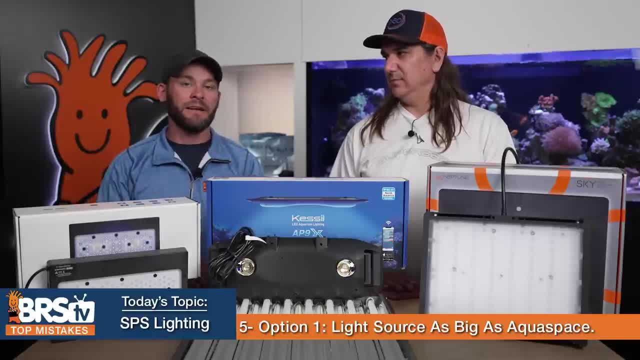 That means it's getting hit on all sides, from front, back, side, side. So one way to achieve this big, large blanket of light is to have a big, large blanket of light from a big, large tank. So one way to achieve this big, large blanket of light is to have a big, large blanket of light from a big, large tank. 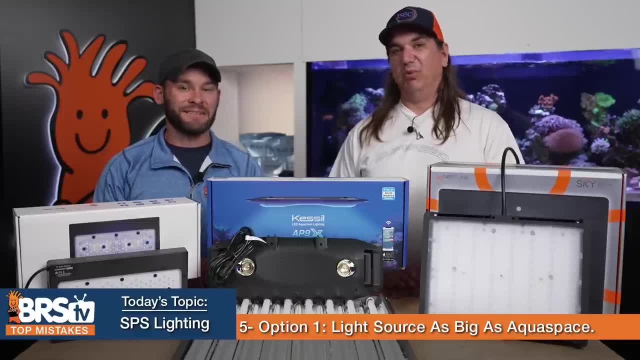 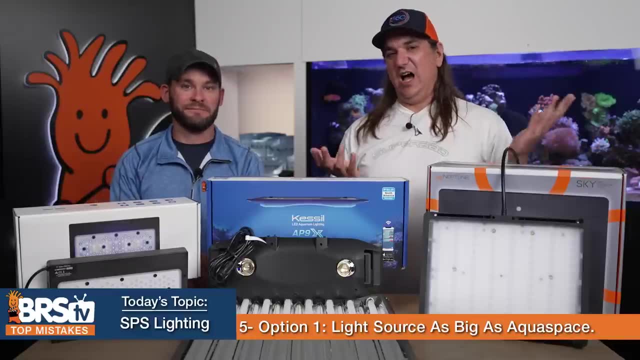 What is a large light source? We call it the blanket of light that wraps the object and light, By definition, it actually has to be bigger than the object you're trying to illuminate. Yeah, And so in this case, that bigger the tank, because I don't need to actually illuminate the glass, per say. 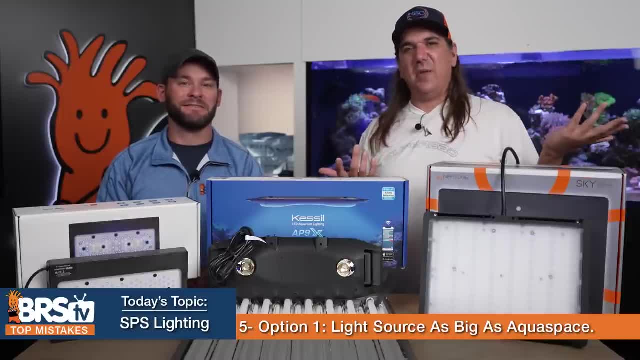 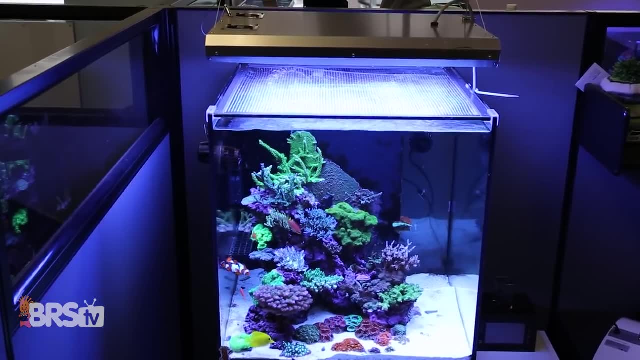 Right, It's bigger than the aquascape and the coral. So, like if imagine I had a two foot tank, this fixture right here of T5's is going to cover it. it's going to hit it from every angle. Plug it in, Done. 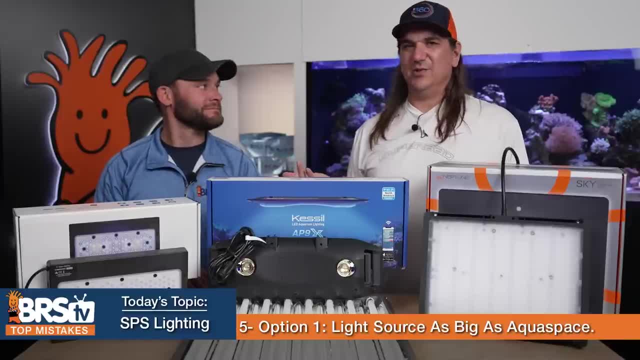 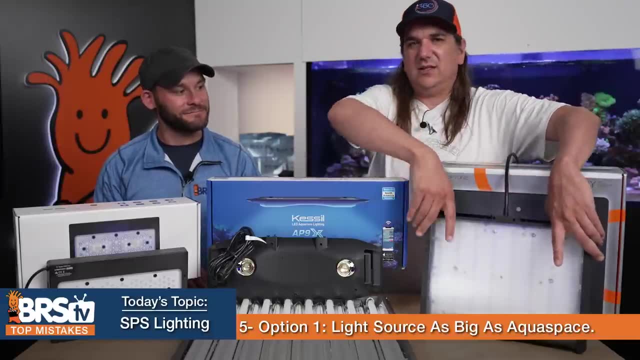 Now T5's lights are getting larger, Right, Right and less and less popular as time goes on, just because it's fluorescent lighting and you don't really use those in any applications anymore. But you can see something like the sky here actually does that as well. 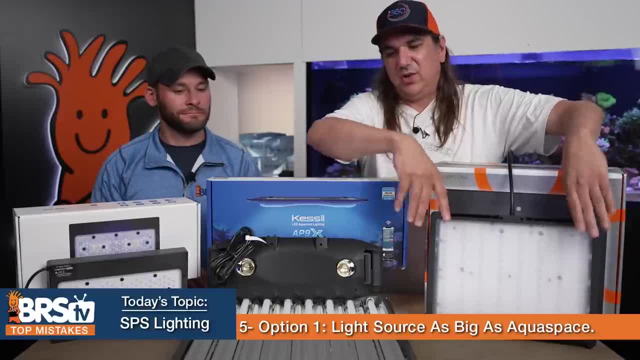 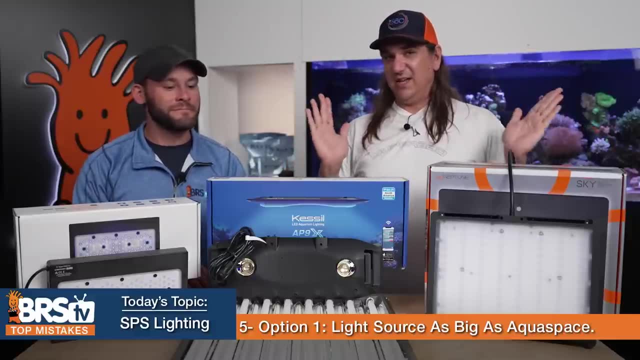 Like this is actually pretty darn close to the same coverage area as something bigger than that. You're gonna miss just a couple inches on the side, but it will actually reflect off the glass and be really, really close. So in some ways, kind of a balance. 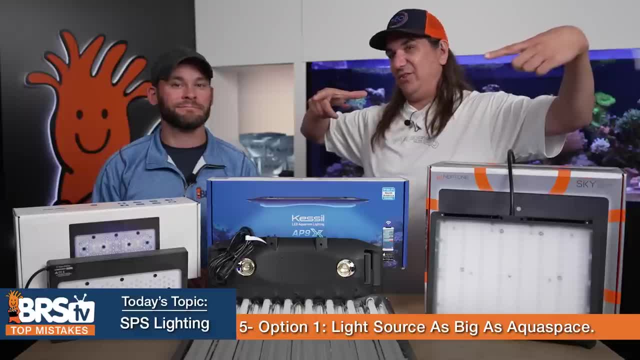 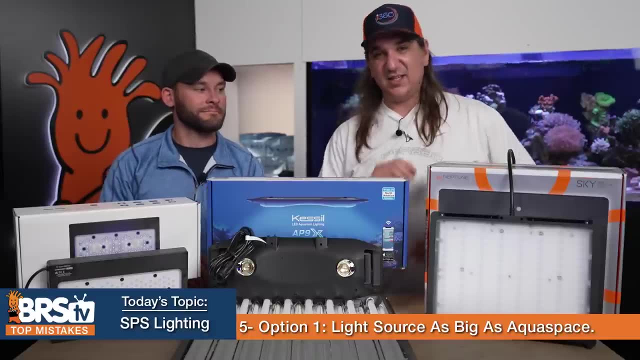 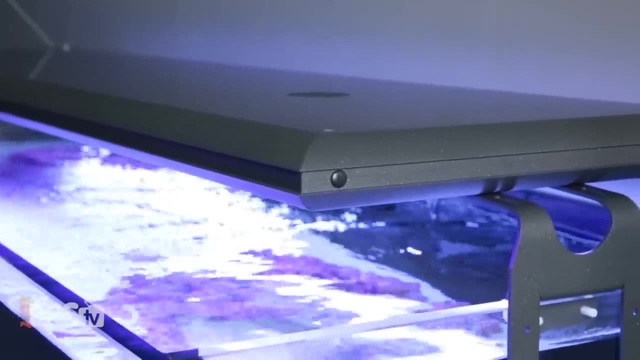 between getting something as big as the object but also a little tiny, smaller form factor that allows you to use it a little easier. So, yeah, you get something big that covers the whole thing. It could be a big giant LED fixture. It could be a big giant T5 fixture. 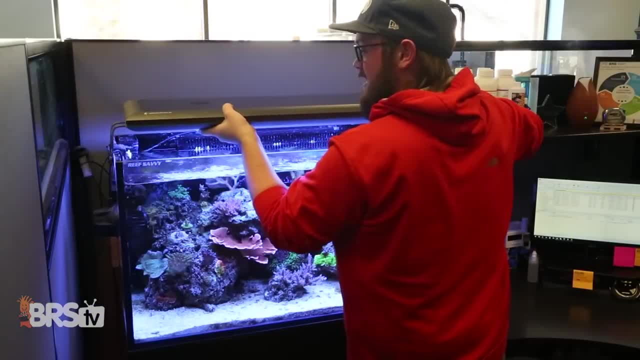 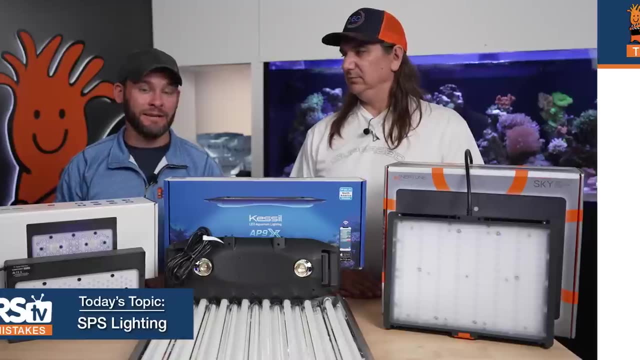 It could be halides, or it could even be just larger size modules and multiples. So number six, option two. Yeah, option two for making this big, large blanket of light is using a lot of different, smaller lights, So we just 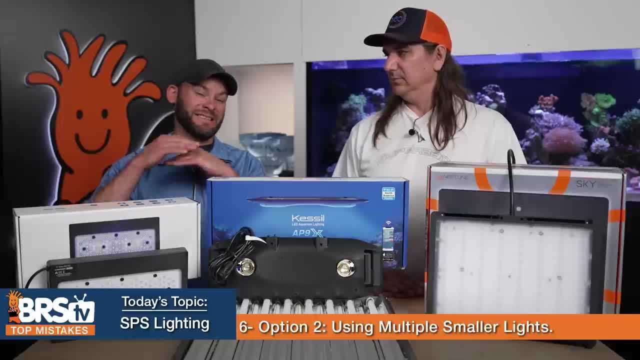 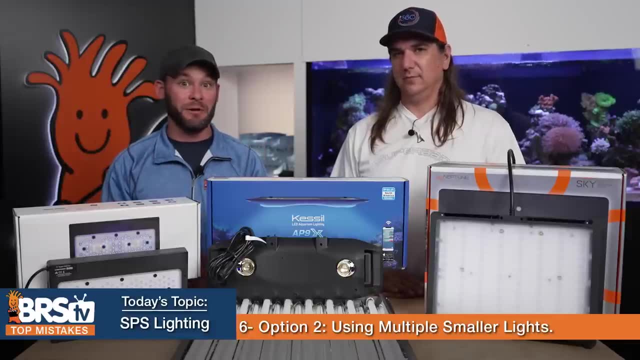 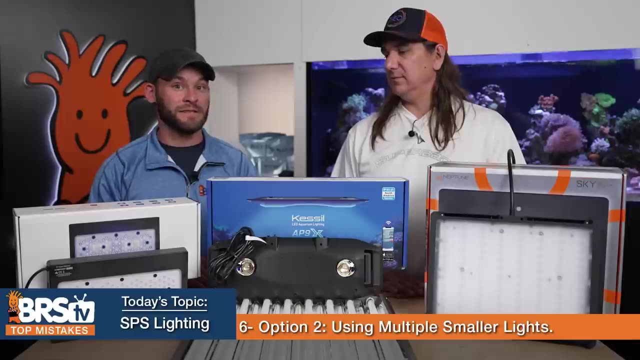 we've been on the AI prime and how eight of those we saw like this very even unique distribution of light. Light is definitely coming from all angles because we have eight AI primes, You can get this done with, you know, three or four of your other lights like XR-15s. 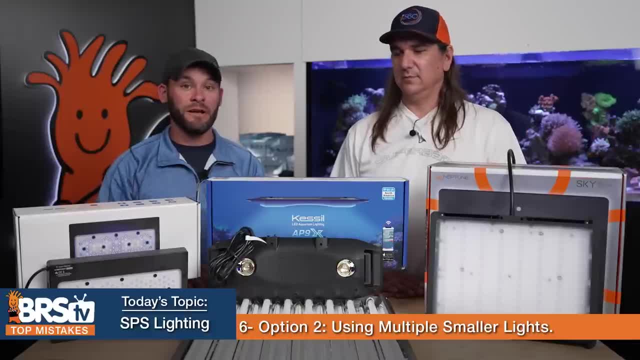 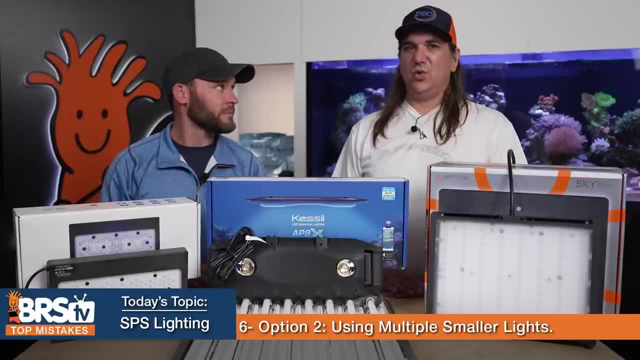 Maybe you wanna put four of those two rows of six or three, But essentially what you're doing is achieving that same big, large blanket of light but multiple small form factors. Yeah, so you know, think about it. There are wide angle lights now where the cones intersect. 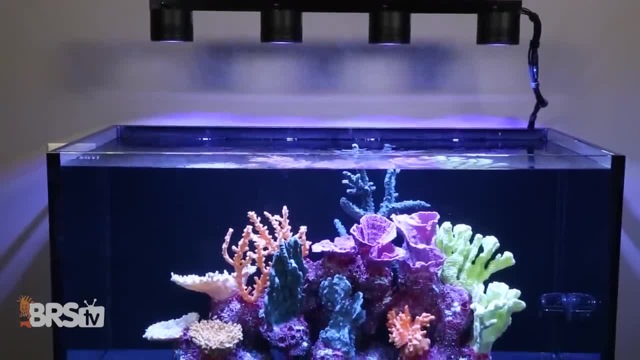 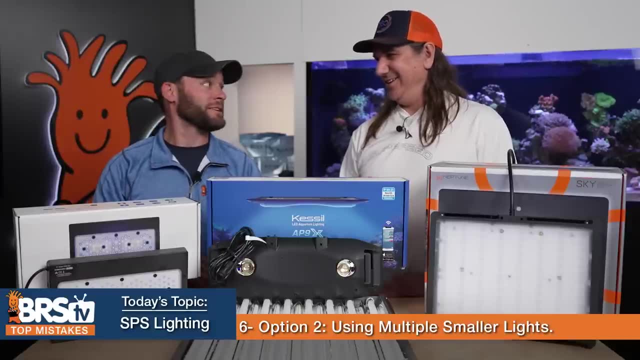 and you just need to have enough of them. And the important part here is to know what your goal is, Cause your goal is actually different than most people's. Yeah, If you're still watching this thing, You're SPS dominant. You're an SPS nut. 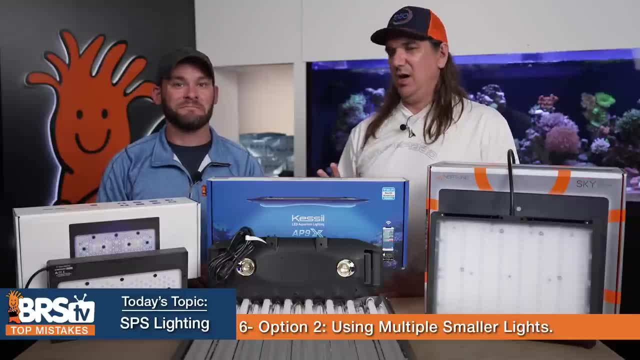 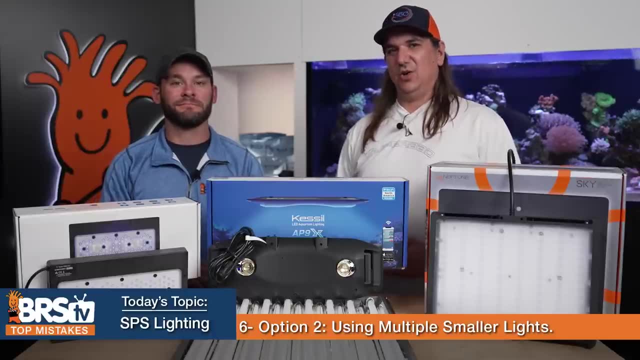 You're doing an SPS dominant tank wall to wall. It's gonna be awesome. Well, you know what? You're part of the upper echelon of like 5% of reefers trying to achieve something really unique, And so you know the two foot area. 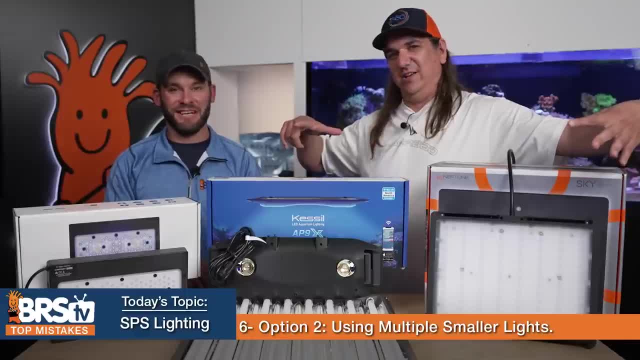 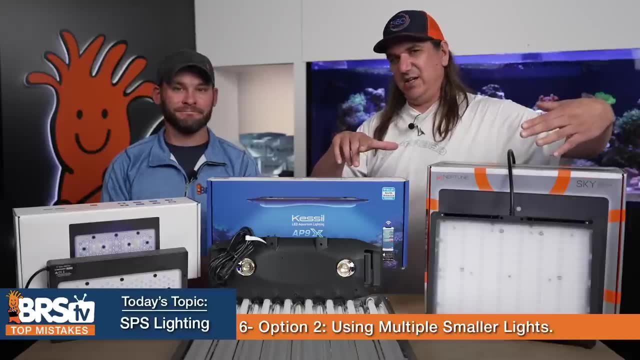 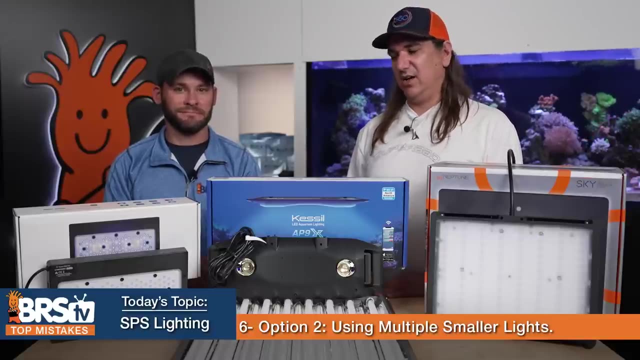 really doesn't apply to you. It applies to the other 95% right And in this case I need these intersecting cones of light. It's probably much closer to like an 18 inch area, depending on the light. I can tell you that, like on the 750XL up front. 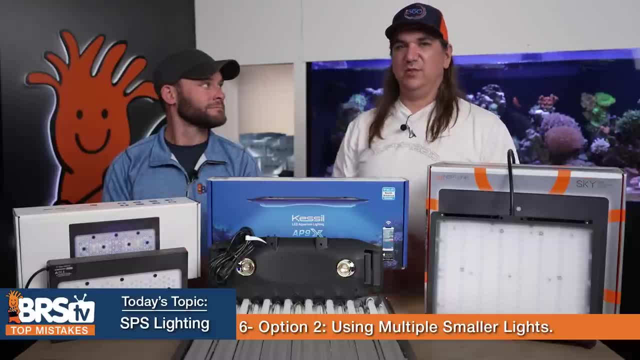 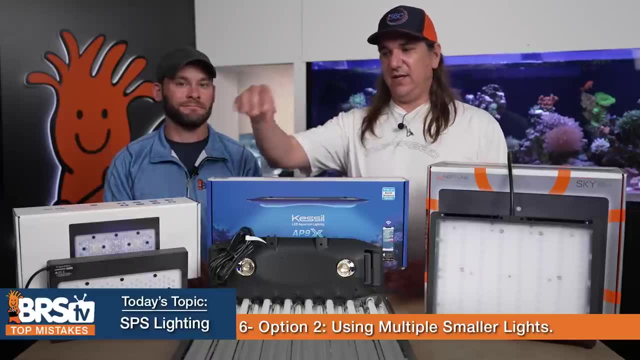 you know, it would normally call for a six foot tank for three of these, But in our case we used four, you know, and four seems to do the job Because, again, these XR15s, one of the cool or 30s here. 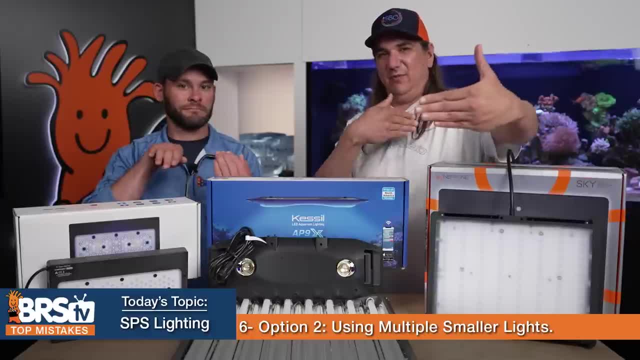 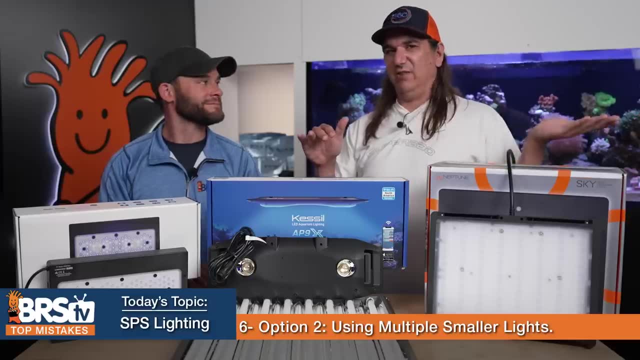 one of the coolest things is I can actually turn them sideways and have them front to back, So they actually cover pretty good front to back, And then I'm gonna space them in a way that I also understand that I don't necessarily have a lot of corals on the very ends. 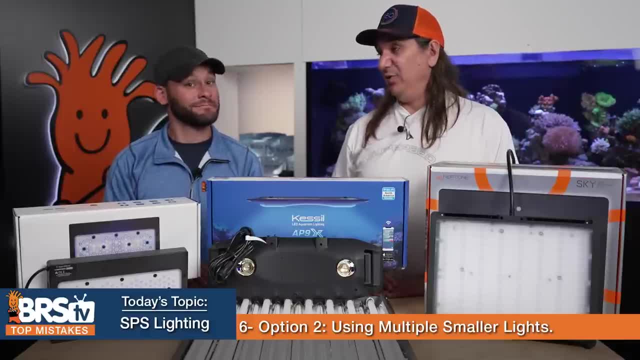 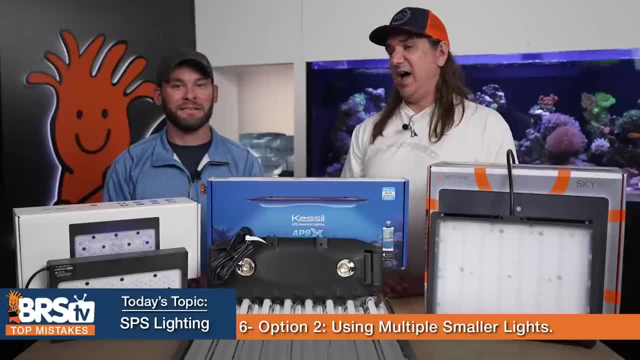 And I'm gonna light the tank. aluminum, You could do five. I will tell you, though, that we had 10 of the XR15s, and we went down to four of these, And we actually got the same or better coverage with changing them out. 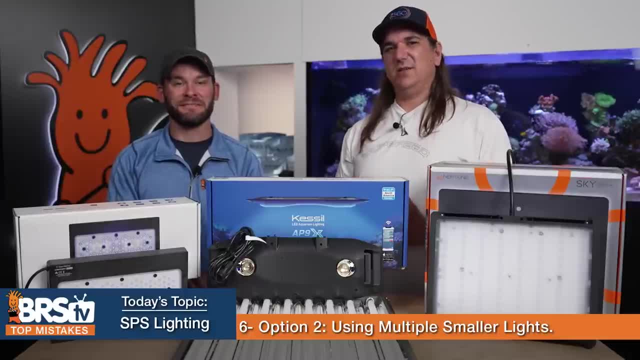 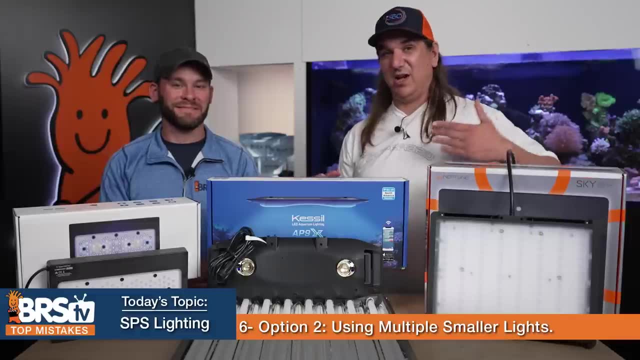 You're going from gen fours to gen fives in that case, But the message is still the same And you heard it again with the primes. The primes actually would be an even like lower cost method of achieving the same kind of coverage. We could put you know eight of those one inch. 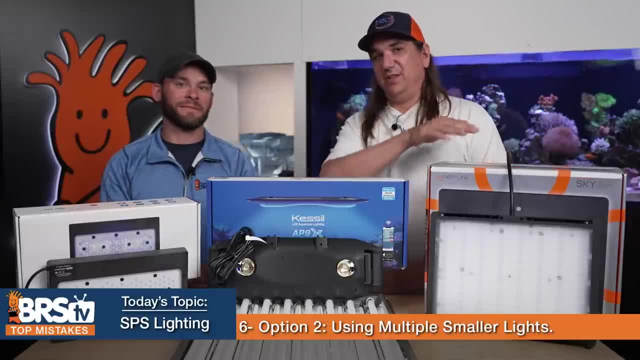 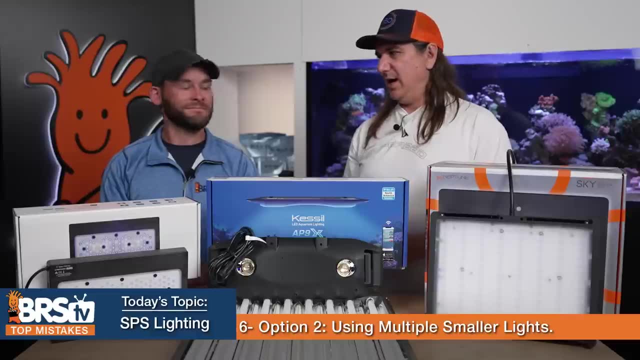 or small $200 pucks over the top of the tank and actually do it for less expensive money. You get really good coverage. So if you're gonna do the multiple light method, put some thought into. you know how wide angle is it. 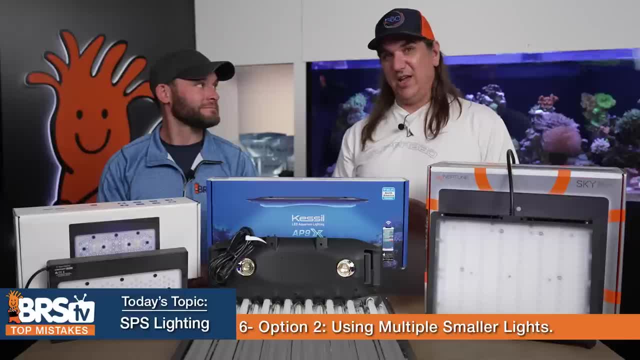 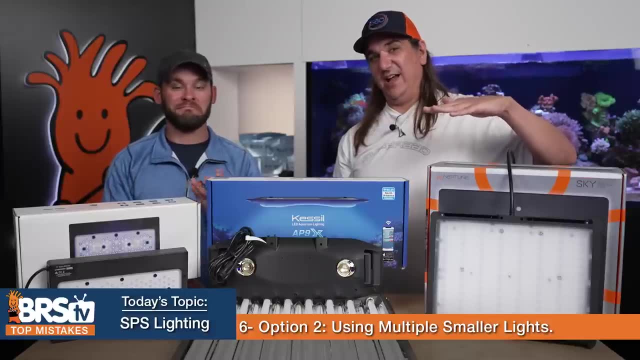 And I will give you a hint- that when you watch a lot of our videos, the wide angle means that we suggest a low mounting height. So the mounting height tends to be around eight or nine inches. the Kessil A360s are a good example of that. 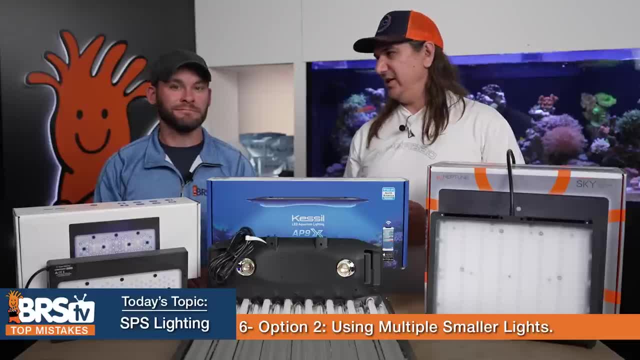 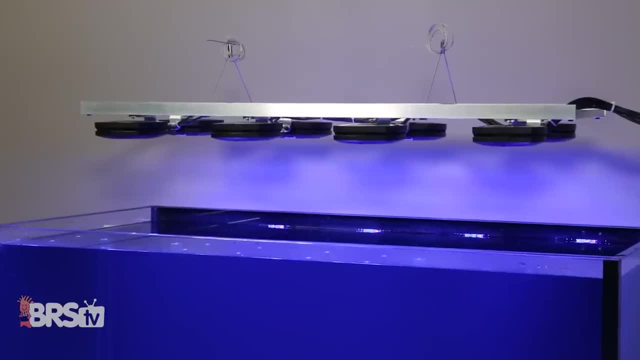 Even you know the 900, turning it sideways as well. All of these options you know are designed about eight or nine inches, means they're super duper wide, and great options to mix them together and get that blanket coverage of light. 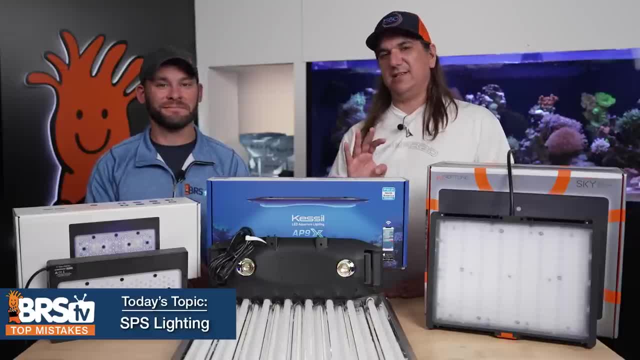 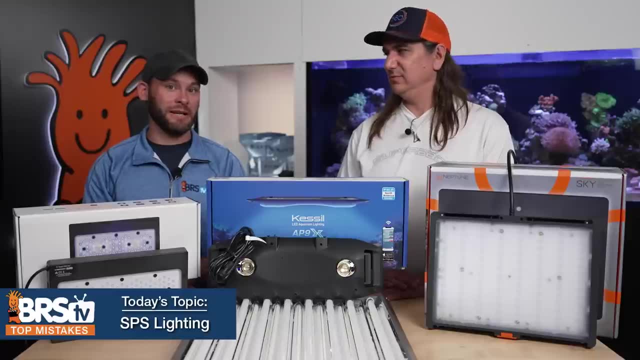 So number seven: we saved the best for option three here, because it's actually my personal favorite preference. Yeah, so this one option three- to create this big giant blanket of light is using fill light with a wide angle. So this is exactly what you think of. 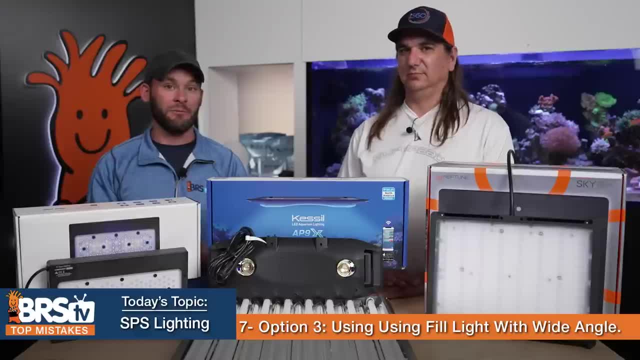 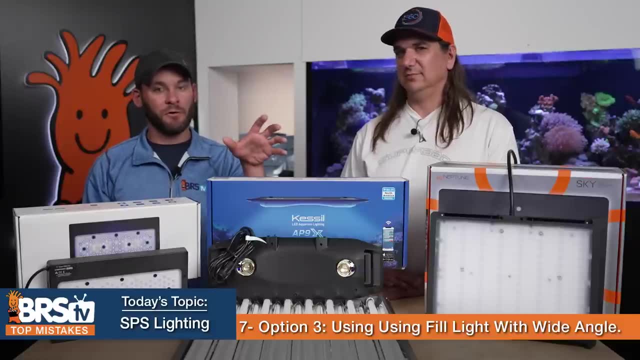 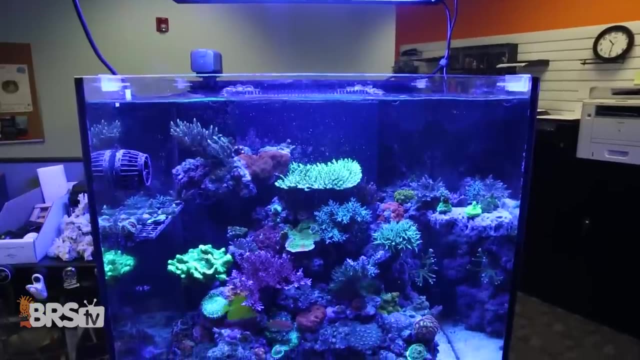 when you think of hybrid lights- So the T5 LED hybrid or the reef bright LED and XHO strip and LED hybrid- you're taking your smaller form factor, wider angle light and you're adding it to strips of extra light, which then creates all of these different spots. 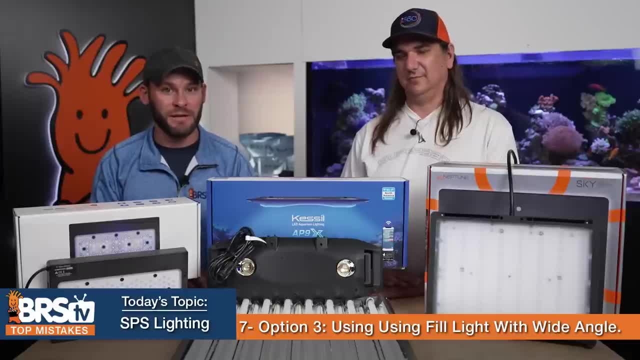 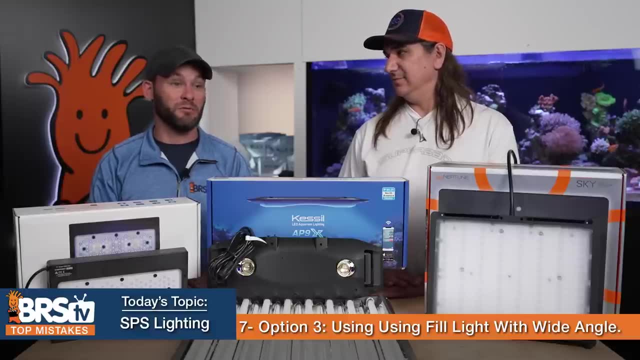 You've got lights from coming from all angles, You can hit these wall to wall SPS. The one BRS 160 is one of the prime examples of that and covers the whole tank in a really cool way. actually, I like it. 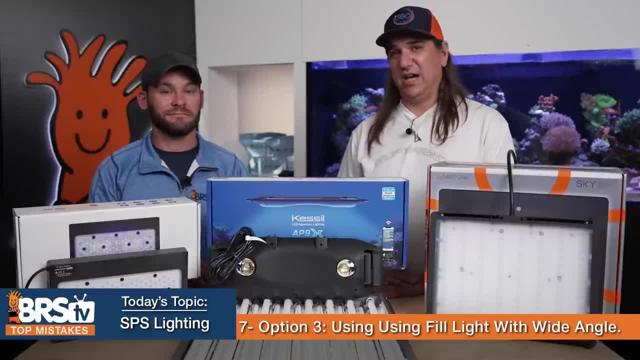 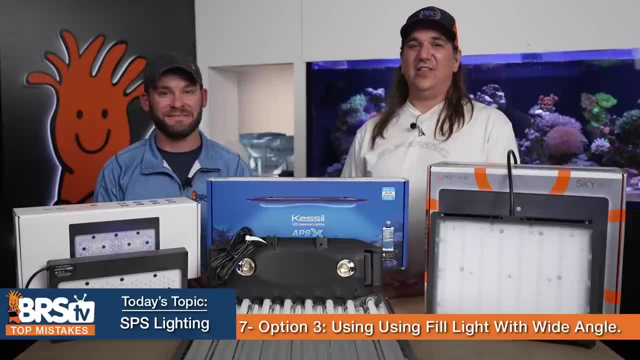 So I'm going to tell you this. there's three different examples of this hybrid lighting and why I like it so much. The first one is the sun in the sky, Yeah, And so there is the natural element, So in the ocean. 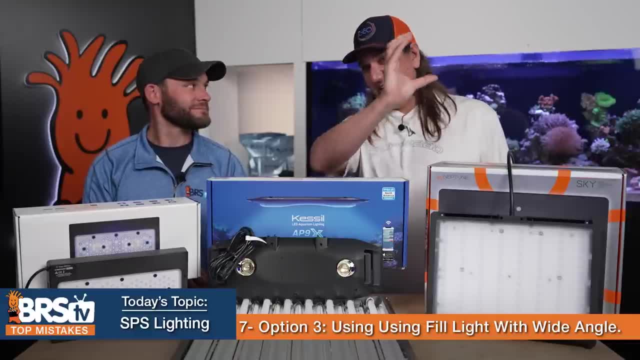 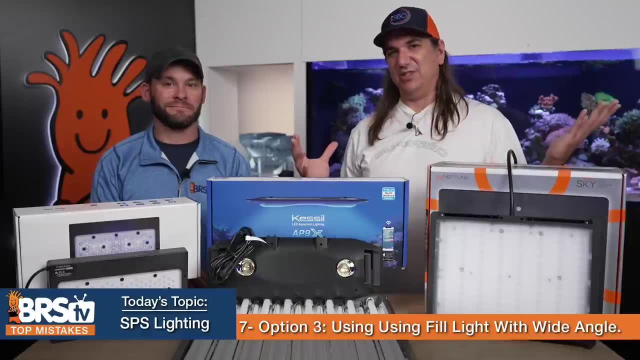 you'll have this really intense ball of light being the sun, hitting it from different angles throughout the day. But what's also happening is the sun is hitting the Earth's atmosphere and breaking up the light and turning the sky blue and illuminates the whole world. 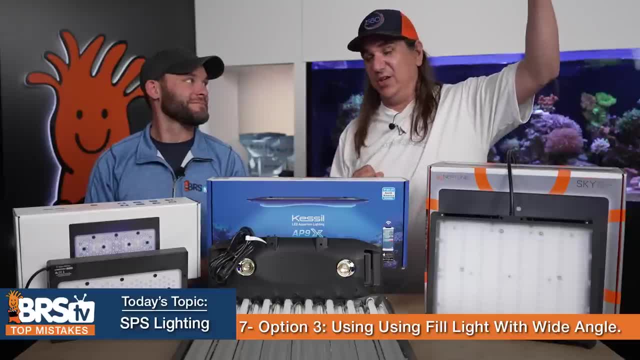 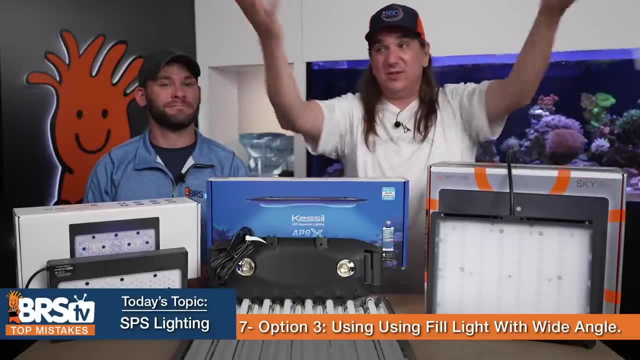 And if you doubt that, watch the sun, go behind the cloud and watch how super bright it still is. It still is, And so the sky is actually producing most of the light, and it's coming from here. It's coming from here, It's coating the whole thing. 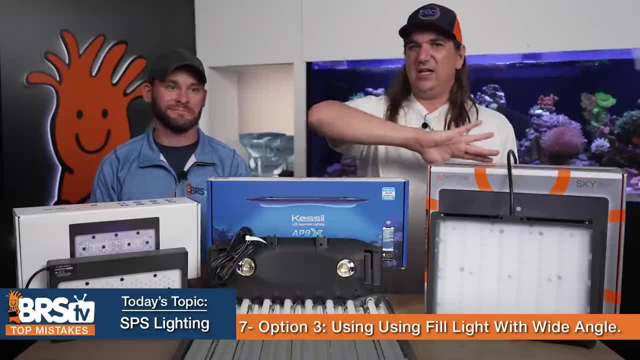 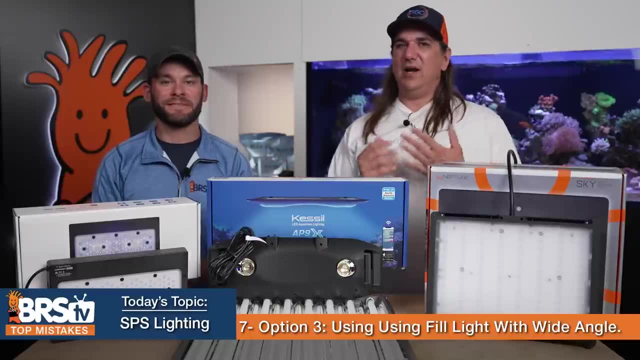 And that's why those corals actually don't die in the ocean is because they're getting it from all angles and they're able to build those like wall to wall colonies in the ocean as well. But it's a hybridized form. It's the sun really intense. 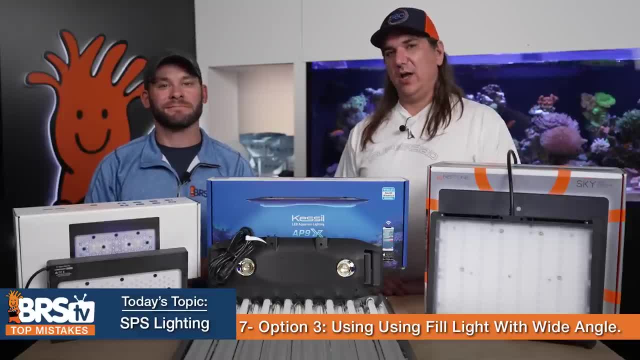 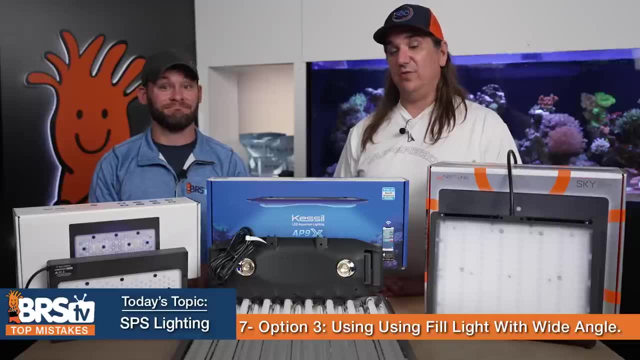 and then, right behind that, the fill light from the sky. All right, So the second one for all of the dinosaurs in the room is: is actually T5 or VHO with halides? Hello hall highs, Little halide bulb providing the sun. 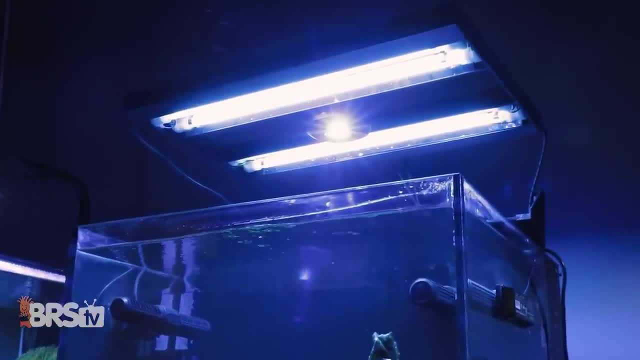 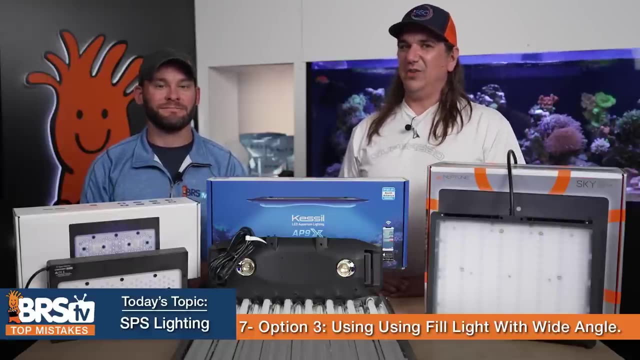 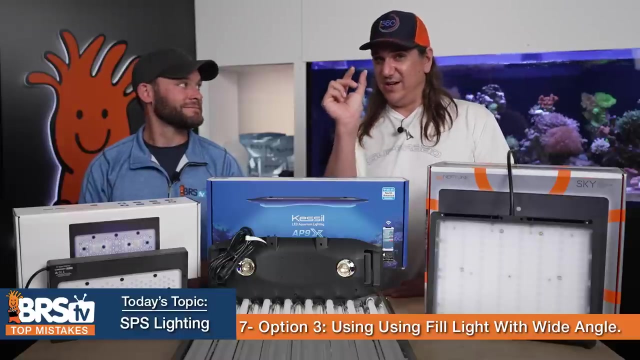 fill light coming from the T5 or VHOs, some of the most successful tanks known to man using that method. Also speaking of some of the most successful tanks out there, the BRS160, that tank is castles Tiny little light like a highlight or the sun. 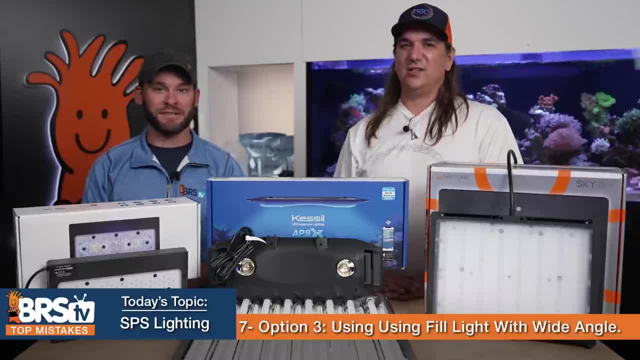 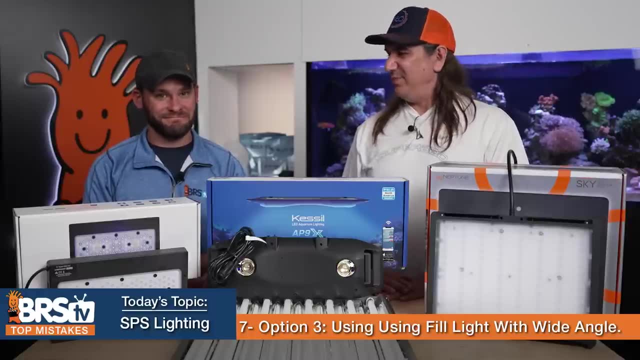 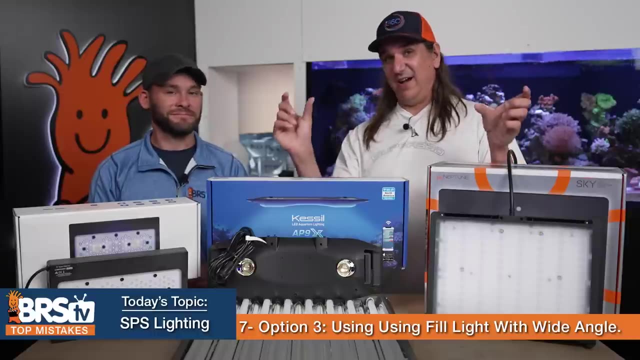 fill light using the T5.. Oh, yeah, Yeah, really, really awesome solution that has worked for I don't know, probably six or seven years now. also, another example of the hybrid lighting: the e170 in my office, the Kessel with the t5 fill lights again. so the beauty of this is you. 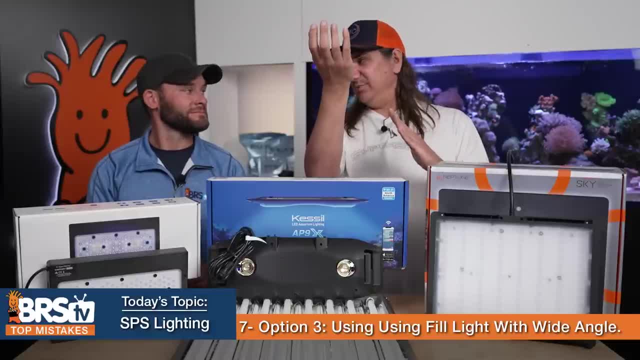 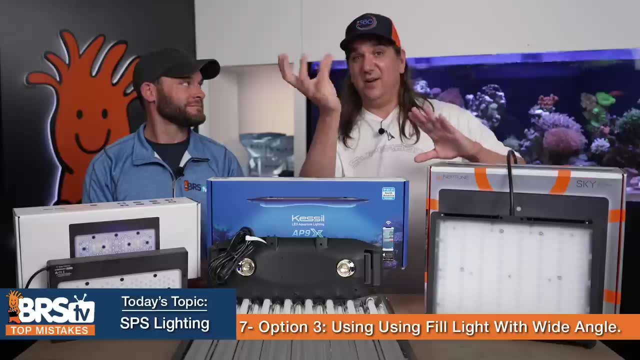 know, have the Kessel on its own, it would definitely shadow an SPS only tank. these are really great for mixed tanks and LPS and like 95% of the tanks out of there, but for an SPS wall-to-wall a like is going to shadow. but if I put these 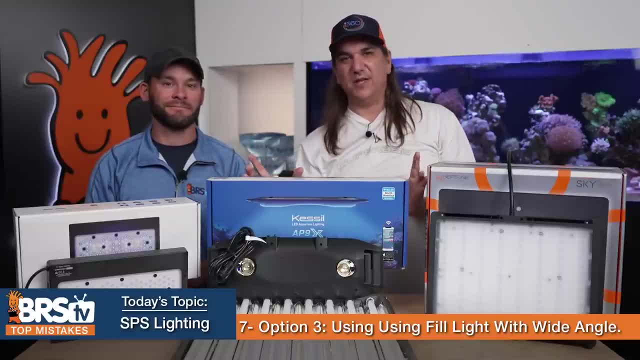 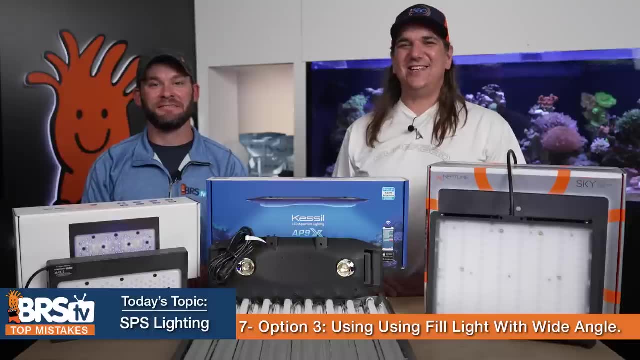 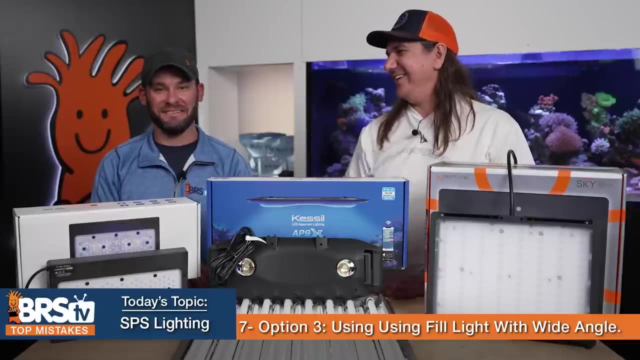 strips on the side, it fills all the light in from the sides. I no longer have this problem and the reason that I know this is because we've well documented 160, even 70. you've seen it in action over many years and most people would see those tanks and say, oh, I want me some of that. that's that thing right. 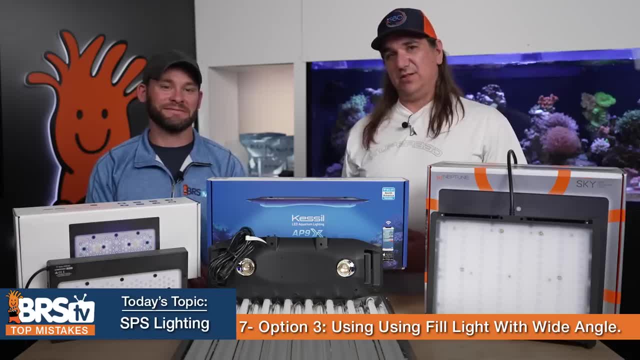 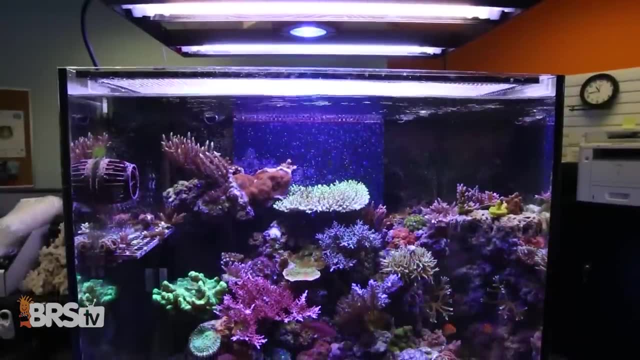 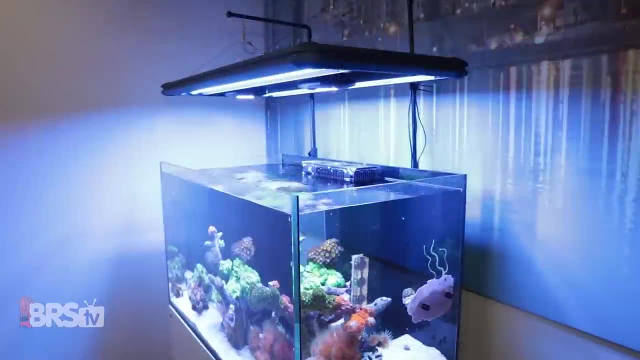 there. that's how you recreate it. yeah, so that is the third option, so we do have those three different options. you can get a big blanket of light from one that just covers sky-to-sky, all over the place. you can also get multiple points of light, like a bunch of AI primes, a bunch of 360 X's, a bunch of. 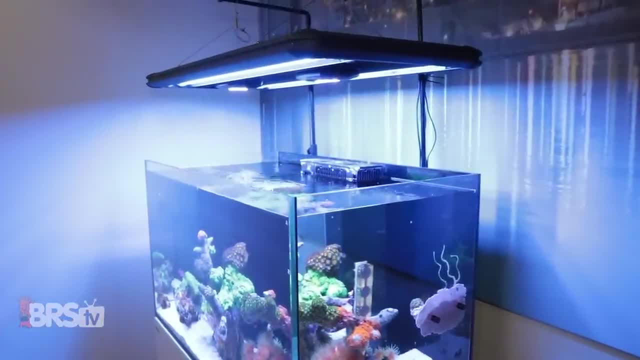 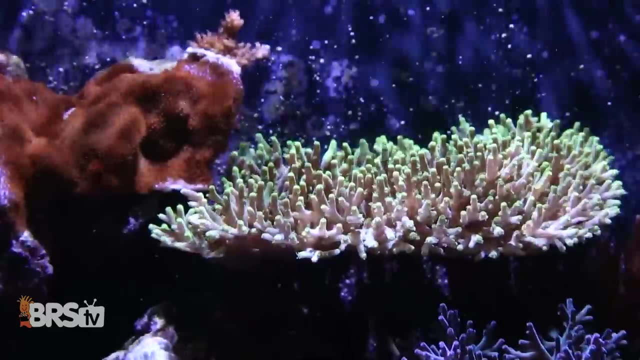 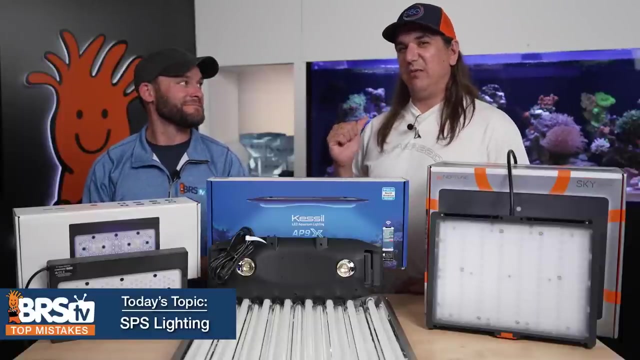 modules like the radians, and another option is to hybridize it all together and one of the benefits that hybridize is you get that really cool shimmer you in many cases. so bring it together and it softens it a little bit with the fill light. all right, number eight, one of those things we just mentioned, probably. 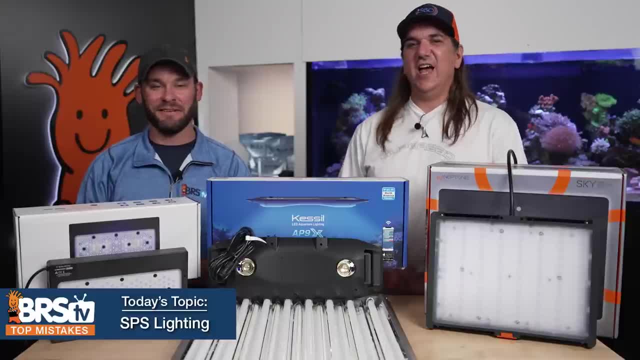 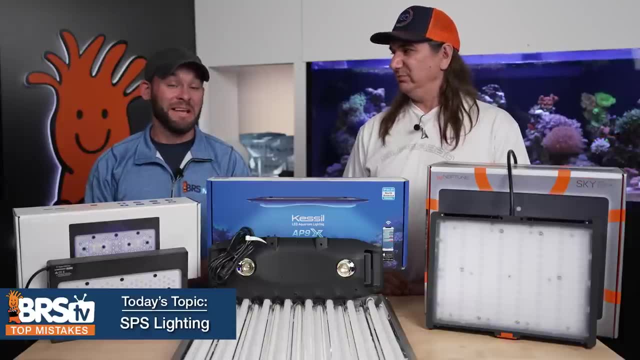 spoke to you and you said: oh, this is a really cool thing to do and I think it's just for me. I get it, yep, but also, you know, a lot of people are overlooking over older technology and maybe shouldn't. a mistake is overlooking t5s, or not. 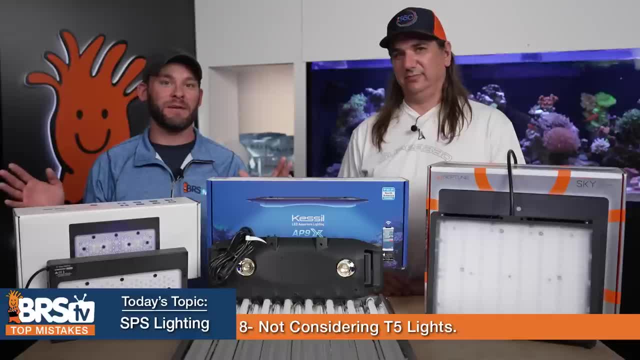 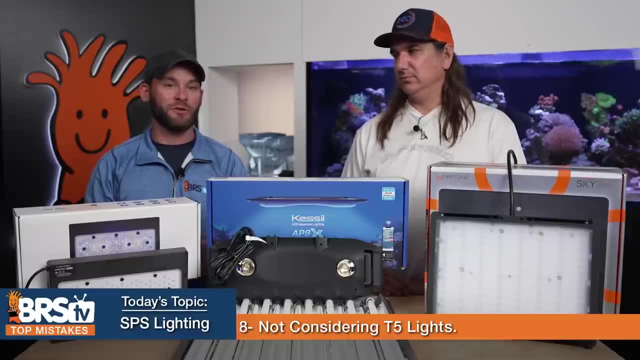 considering t5 lights for your wall-to-wall SPS dominated system. that was my goal. that's what I used and I loved it and I've seen it work. so many plays- this is one that you can point to- is like this works: plug-and-play almost. 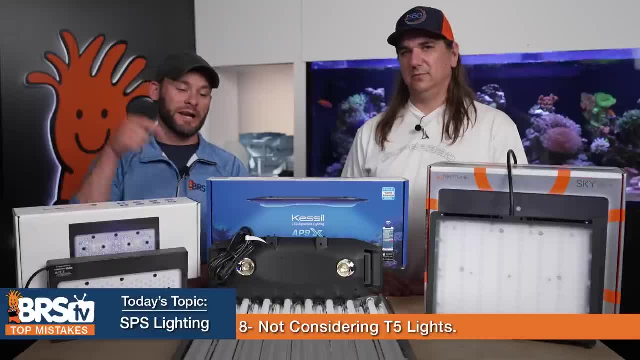 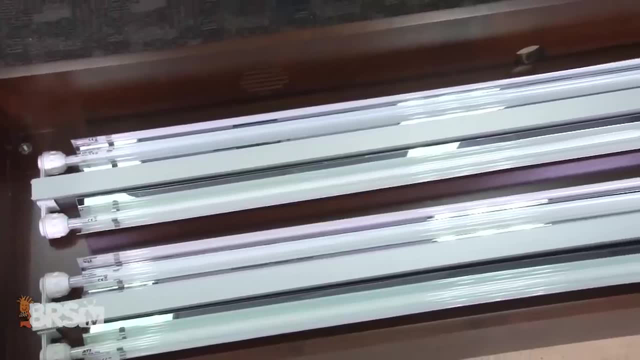 every time. if this is your goal, you're going to achieve it with the tried-and-true t5. okay, I mean, I don't know. you know it's really hard to hear that we should go use these ancient balls, but you know what? they just work. 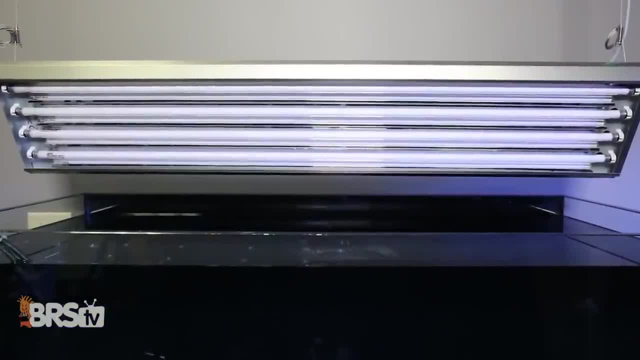 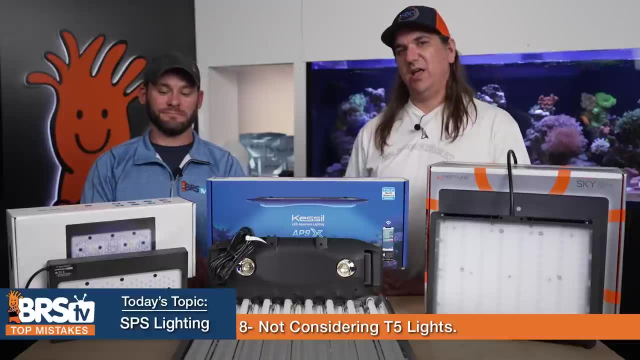 and so I know it's a little bit flat looking for me and there's a reasons that I wouldn't use it. I don't like changing out bulbs, I don't want to buy the bulbs, I don't want to go through all this stuff. but, honestly, if you put the 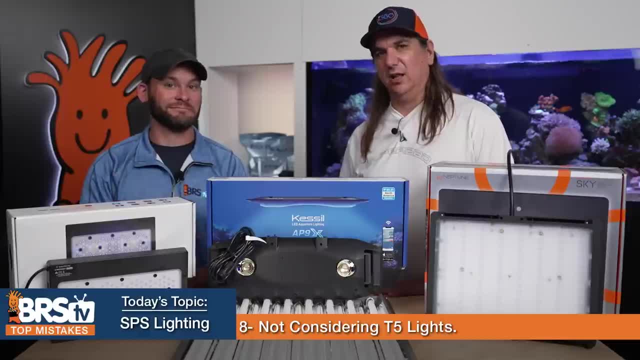 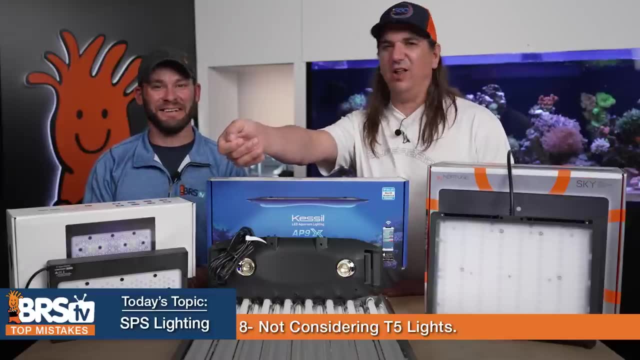 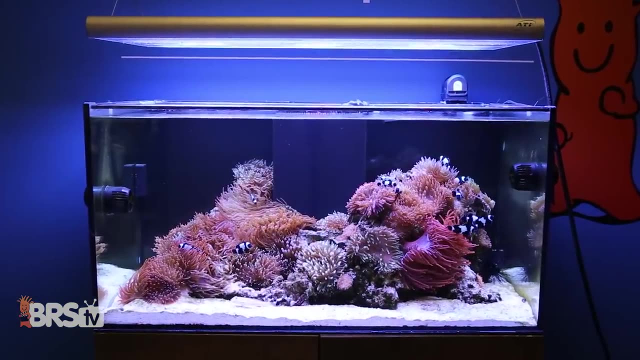 bulbs in it and hang the fixture over. you plug it in. lighting will never be your problem. there it is. you will have mastered lighting by plugging it into the wall. it's that simple and you'll have other things to think about with your reef tank. but you'll never know. if you wonder if you got this thing right. 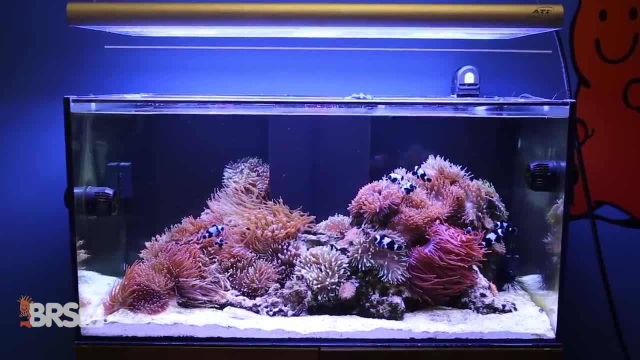 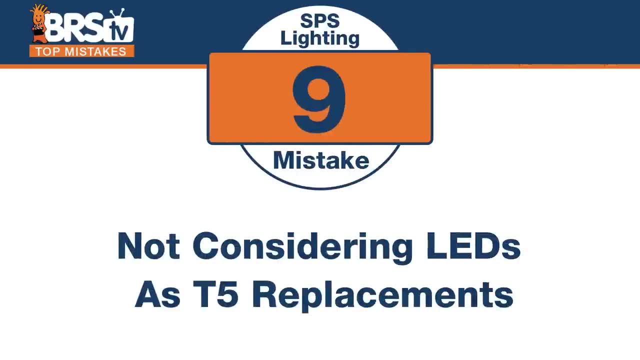 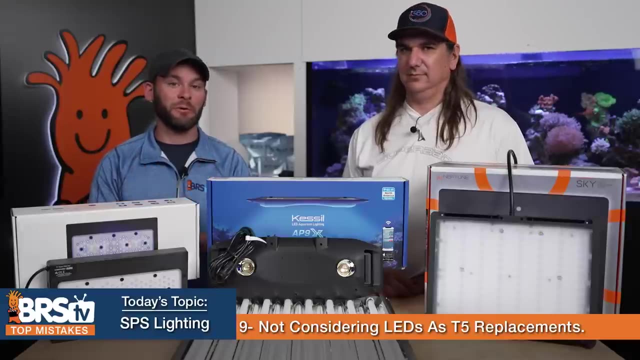 so t5s really still have a place and probably will for a long time. number nine: there's a caveat to that long time piece. yeah, so the mistake here is not considering LED strips as t5 replacements, not just as hybrid. you know fill light that we were just talking about. 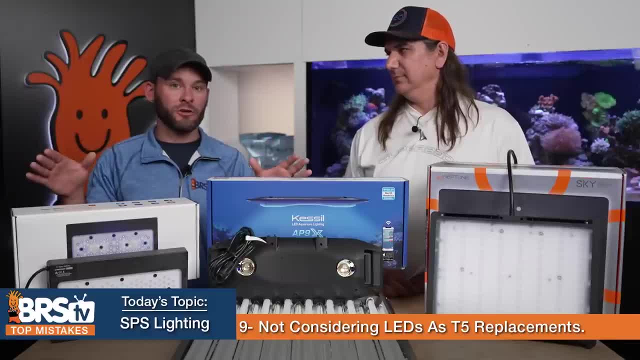 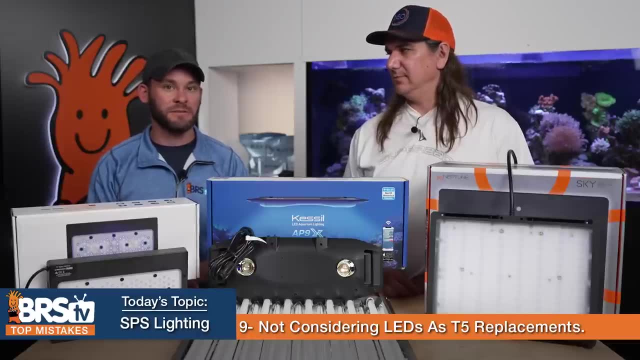 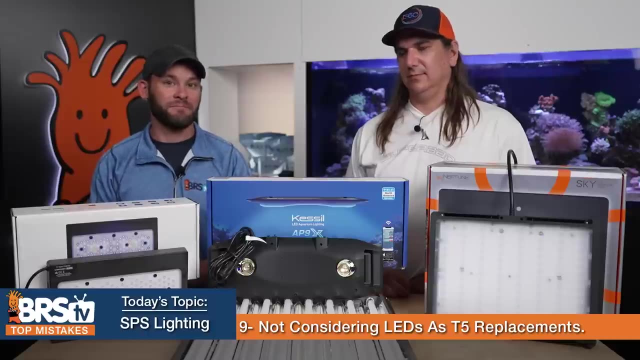 also, as you know, your big giant or your larger fuller fixture itself. I mean, this is something we just picked up in the investigates when we started testing reef bright strips and we found- you know, we tested- the difference between a single bulb, t5 bulb, versus a single LED strip. uh, you know, bump and par same. 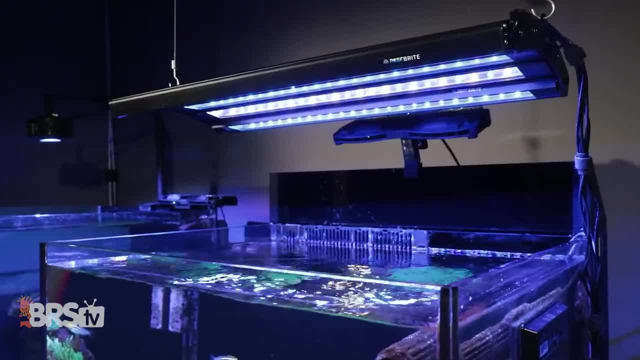 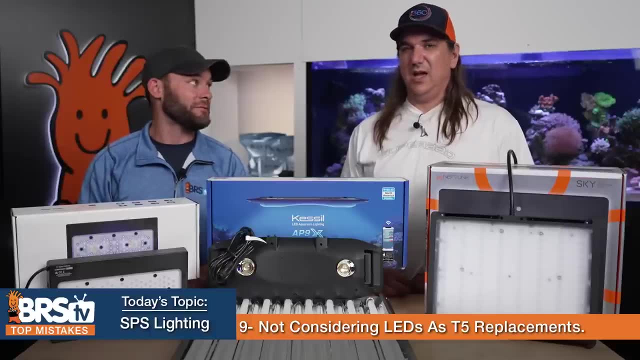 distribution, if not better district better distribution. and then, when we added all of those LED strips together, we found as good, if not a better difference than an eight bulb t5. yeah. so this is where this really matters, because there's probably only like five percent or less reefers that are actually 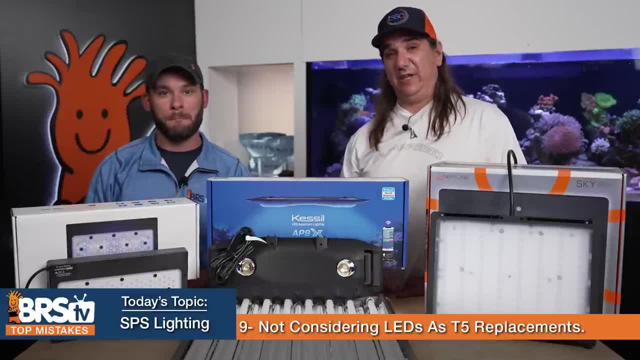 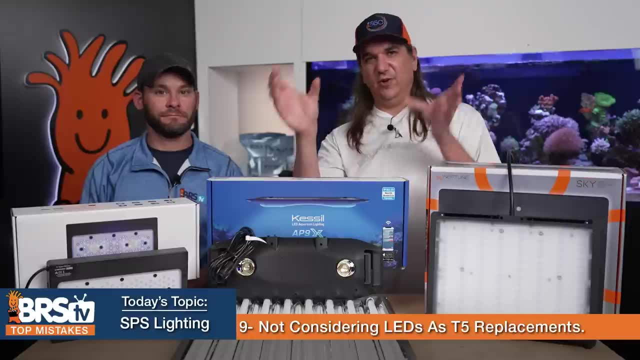 buying big panels of t5s now. but there's a lot of people that are doing that hybridized option, where you know, I got a castle in the middle or a Radion in the middle and I got some fill light bars on the side of t5s. okay, it isn't magic. 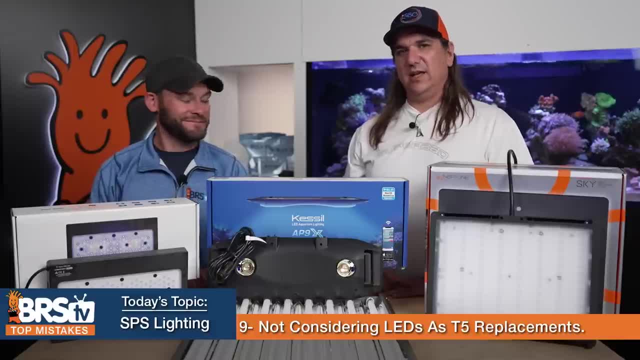 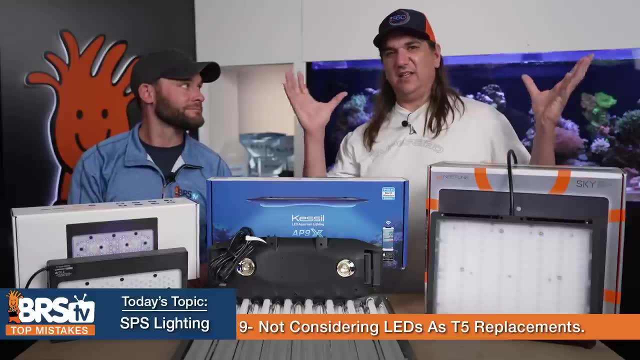 that's inside the t5 ball right. the reason that the t5s work so well is: isn't this magic, uh, like photon that's coming out of it? it's the fact that it's blanketing the entire lie, or uh, tank in the in light and there probably was a. 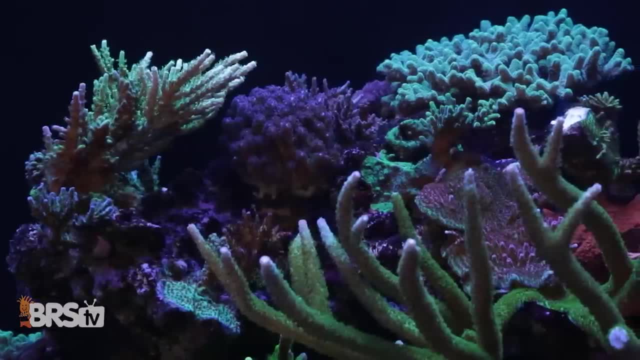 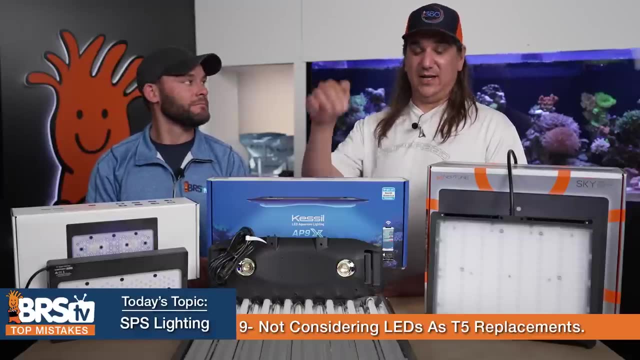 time. you know, uh, eight years ago, where LED spectrum wasn't wide enough, yeah, you know, we didn't know the intensity. all that stuff doesn't exist anymore. no, we're not matching the light to the same intensity of these. the spectrums now well blended in most cases, and it's the right spectrum. the difference is: 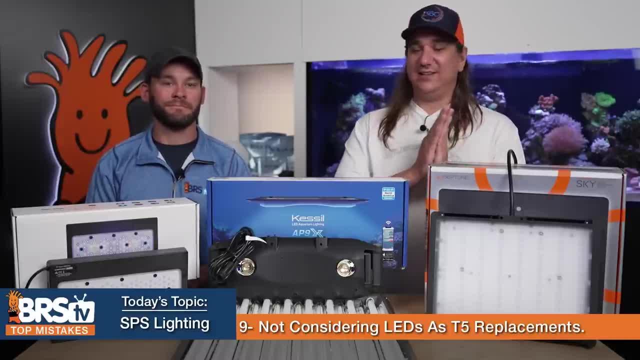 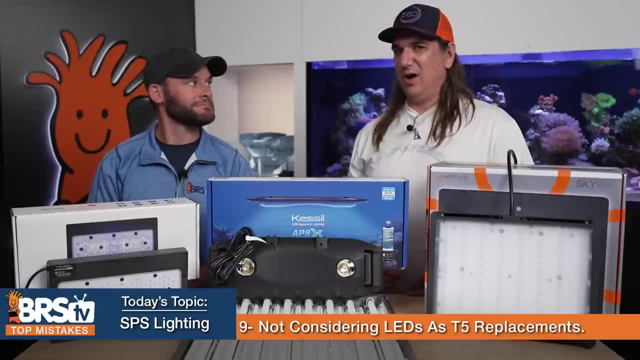 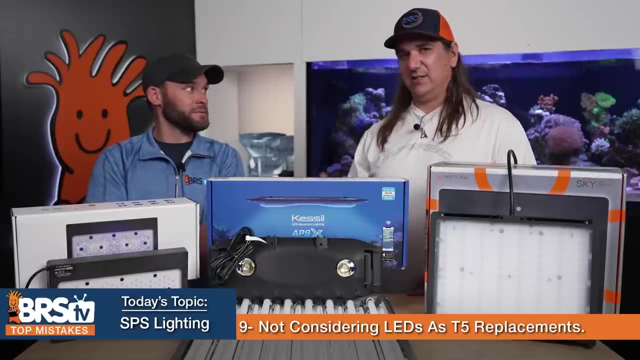 actually the distribution of light. so how do we get light to the way that these coals grow? and it's definitely blanking it in that way. so why not swap out the t5 bulbs with these LED strips, the reef bright ones, or I think aquatic life, you know, has strips or orific. so in 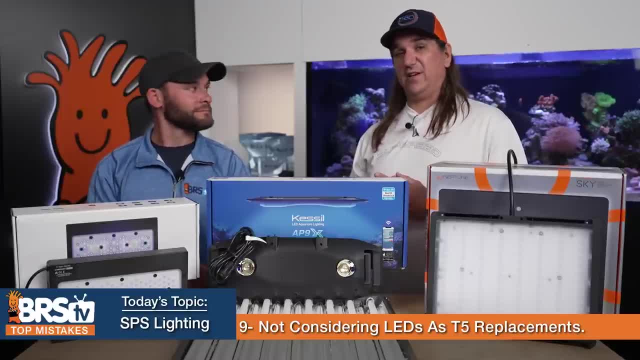 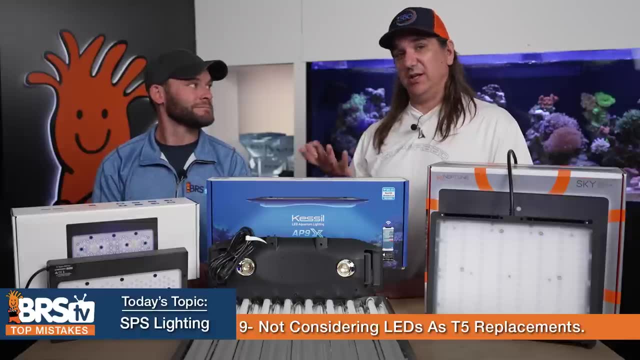 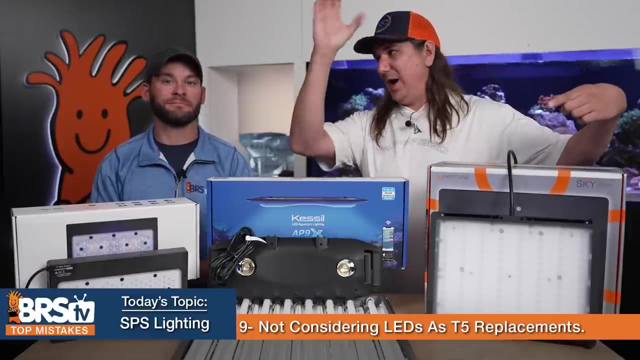 those cases like you're seeing it now. there's like the aquatic life fixture. I mean, an enormous amount of people have picked those things up and probably because you see what that specific picture did, our fixture did to the e170- oh yeah, super easy way to get that hybridized version- drop a. 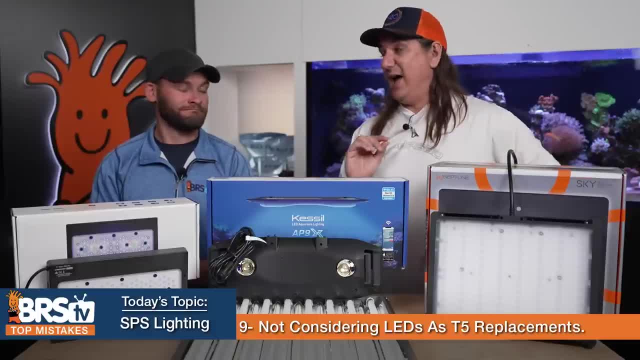 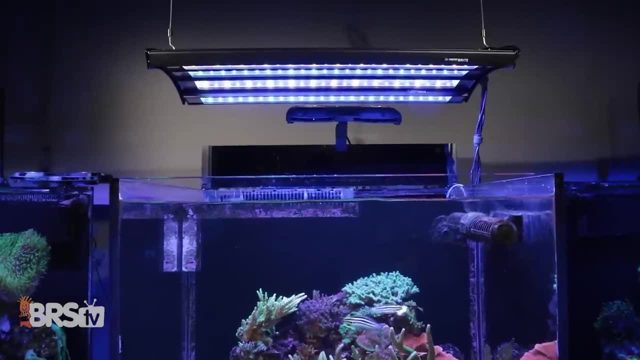 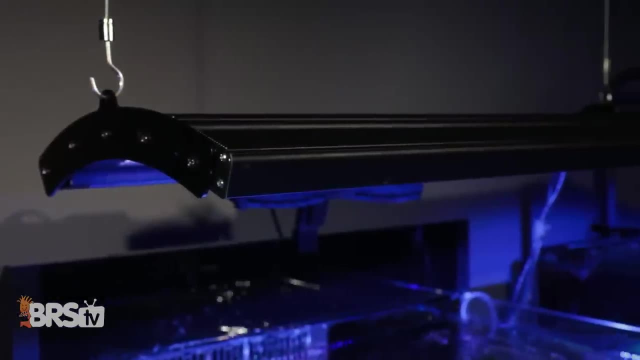 Kessel in. drop a radion in. you got the fill light in there. but now you can get options without the t5 bulbs. you can get it with the the LED strips. specifically we tested the xho ones, where you actually get wider distribution and more par than you get out of a t5 bulb. that's a win-win. all right. so there are. 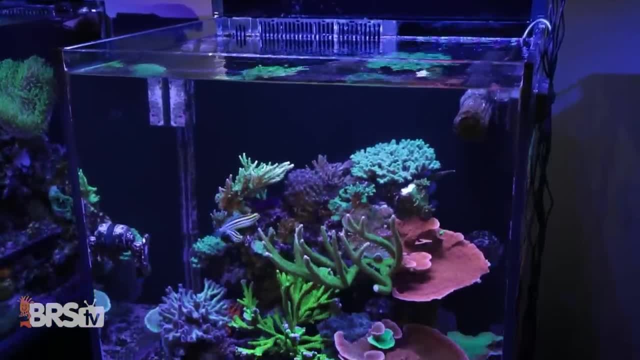 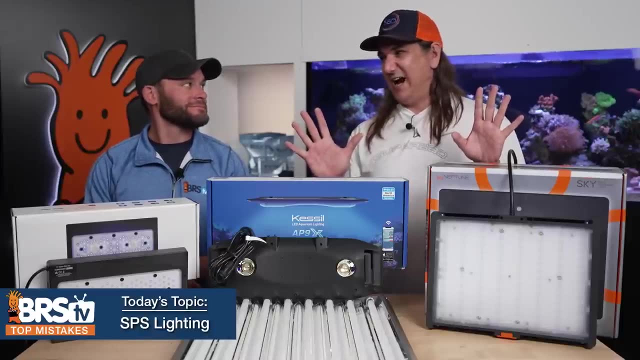 alternatives here where you can get this uh like hybridized combo and step into today's technology. number 10: this is one of those areas where the conversation, when we talk about General corals, actually gets lost when you're actually talking about the five percent. yeah, so the mistake is not considering. 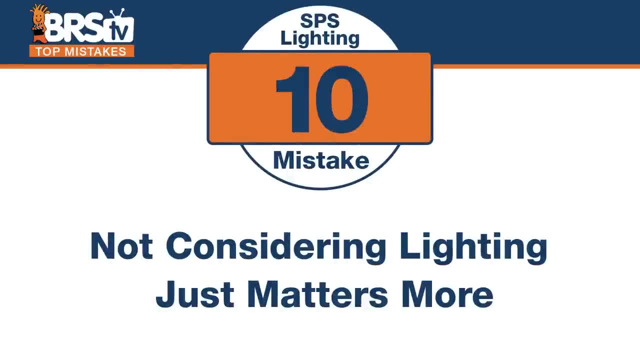 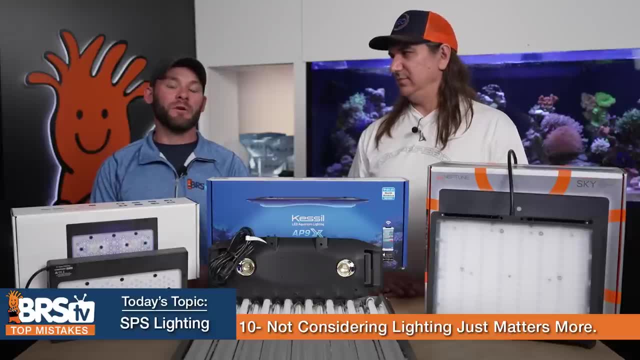 that lighting specifically. if this is your tank path- the SPS dominated wall to wall system- you're trying to do this to the best of your abilities. lighting is one of the most important conversations for creating that type of tank, which is why we harp on the, you know. 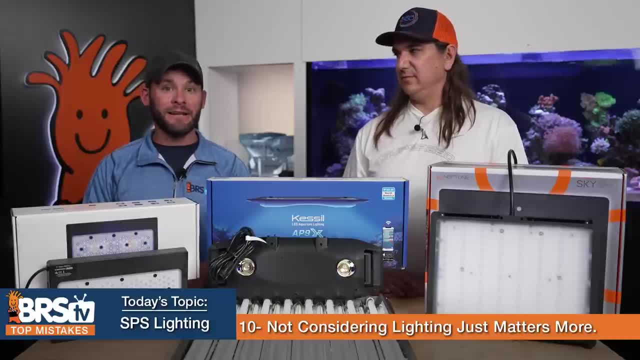 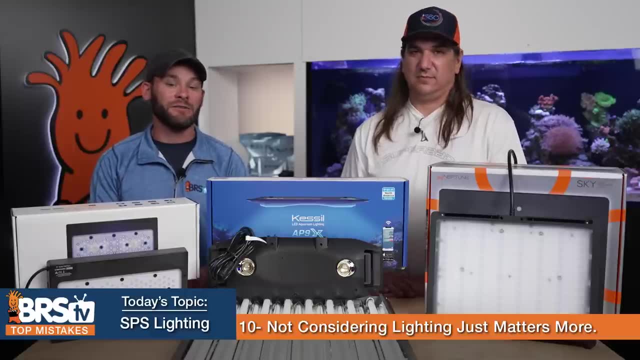 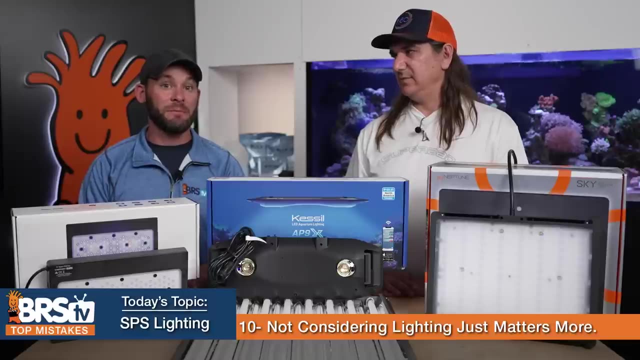 lighting topics so many times. we have so many videos about lighting and lighting properly what lighting means and how the how it works and what intensities and Spectrums and pars. uh, you, we hit on this so big because, when it comes to that big giant wall-to-wall SPS tank, this might be the number one factor to get you there. 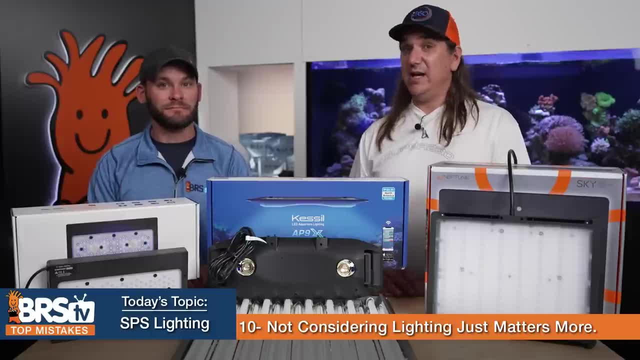 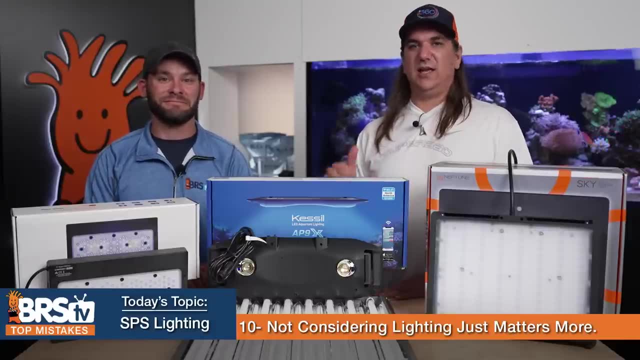 I think that's the point is you'll see a lot of people- maybe even 90, to the community saying: I don't know, I just throw some light on it works. yeah, you know, like I don't work for me. uh, the part of it is there's two things. 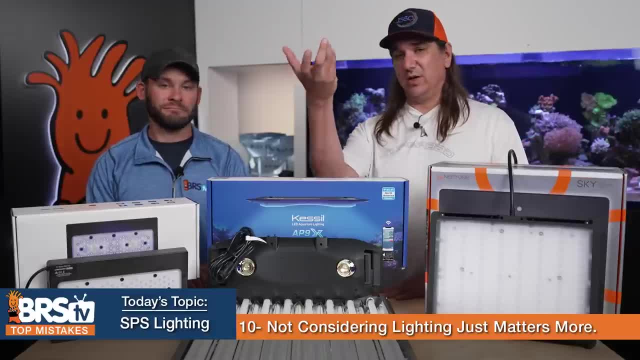 A, they're trying to do something different, because if I'm just trying to grow a bunch of euphyllia, I throw a single Kessel wide angle light on the top. man, I'm done, done. you know, I got all kinds of corals and tank styles. they'll. 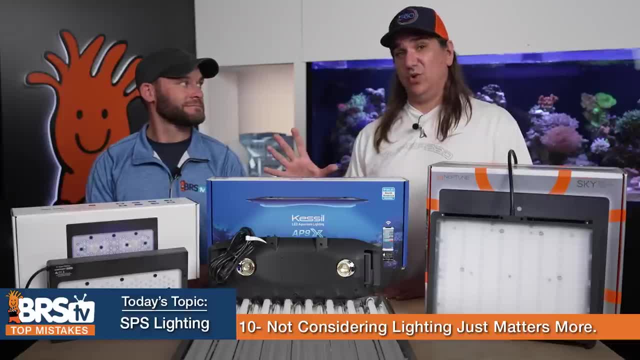 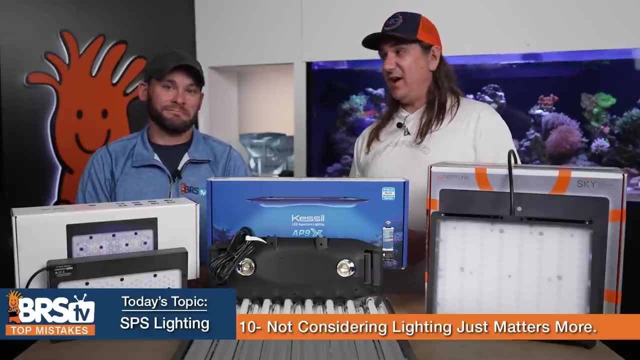 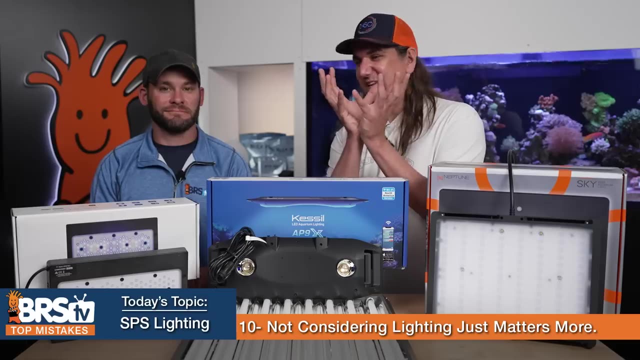 do, if I'm trying to achieve this one specific thing, which is wall-to-wall epic tank. it's different, and one of the things that we discussed earlier is a lot of people say, oh, I do, it's just fine, but they actually have colonies that are this big, not this big, uh, and so you know, and they may never actually get here and 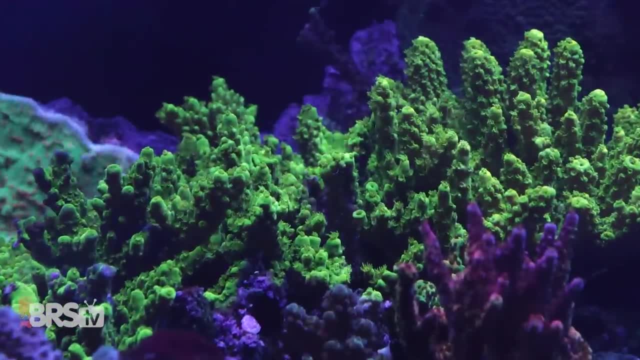 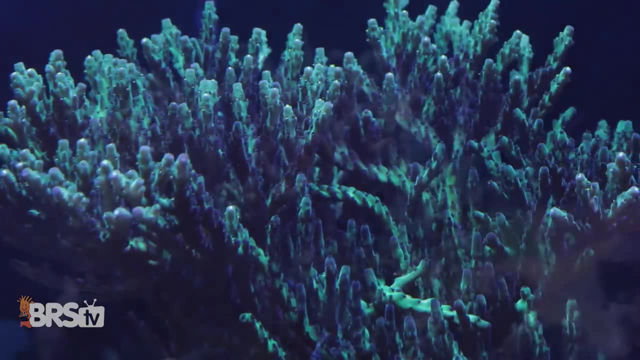 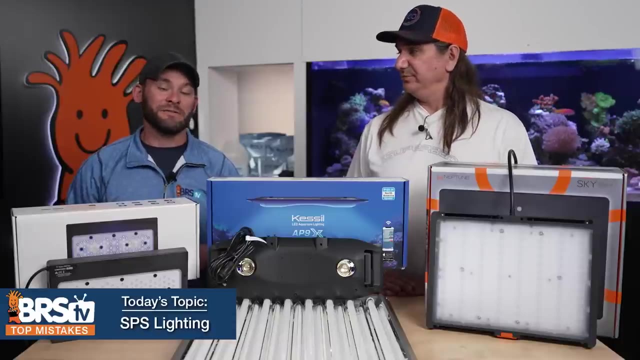 they probably won't tell you why they didn't get there along the way, because they won't even know, maybe in many cases. so, uh, in this case, uh, the failure here or mistake is just not understanding. with this tank style, lighting just matters more so number 11 in that spirit spectrum matters, yeah so. 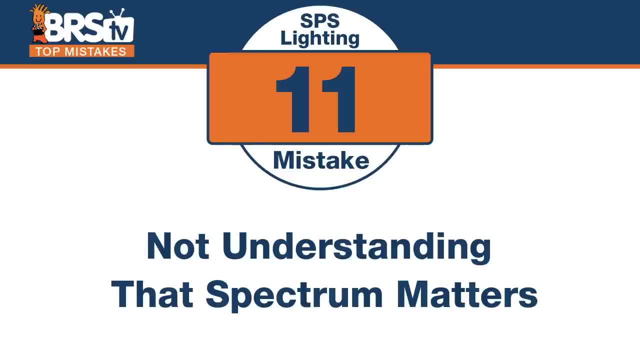 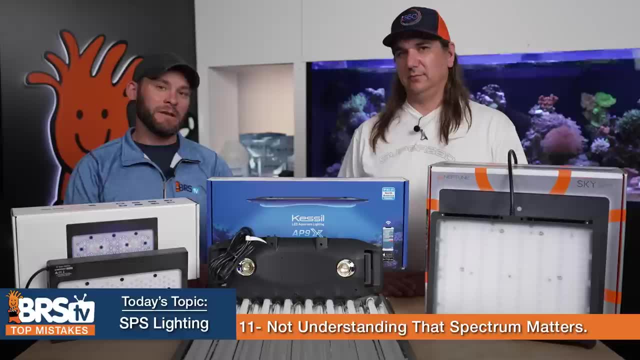 mistake is not considering the proper spectrum or understanding that proper spectrum matters- and you know this goes back to T5s and metal halides, but one in particular wavelength of that of uh spectrum that has time and time proven uh to work on every application that you throw a T5 in. 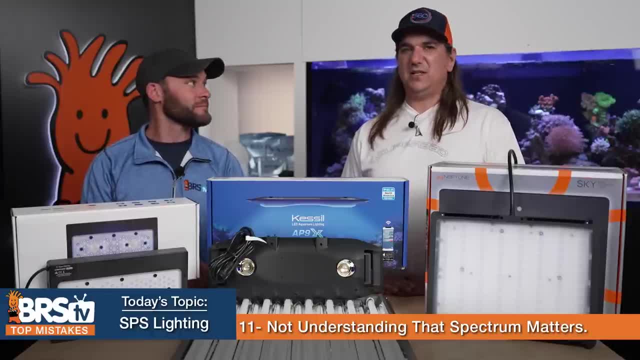 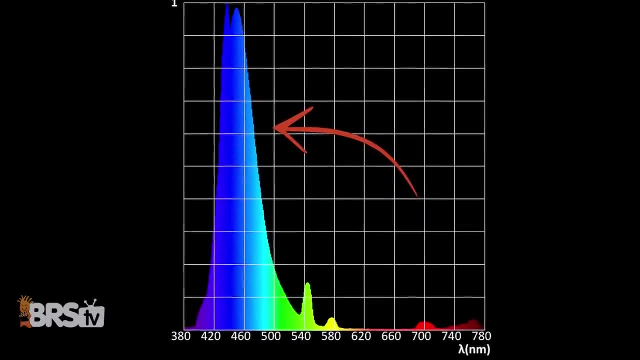 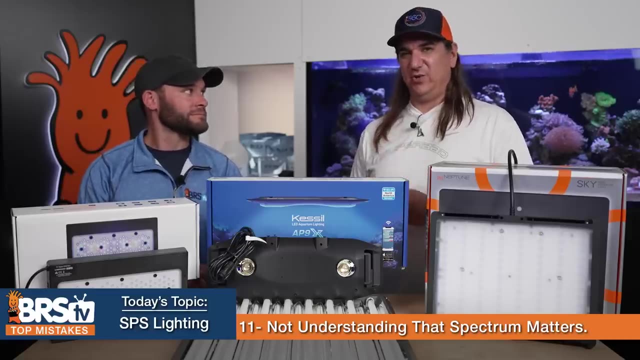 that's the uh, the B plus bulb. basically, what that is is just a wide, uh breath of blue that you know, really hits all of the different areas of chlorophyll and carotenoids, and we get to better understand that, and so most of these lights now do that and most of them also have leaped into. 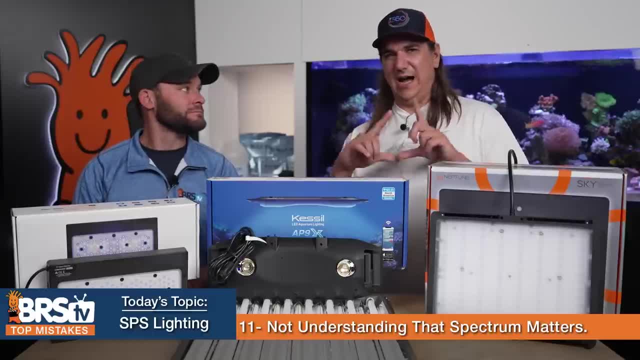 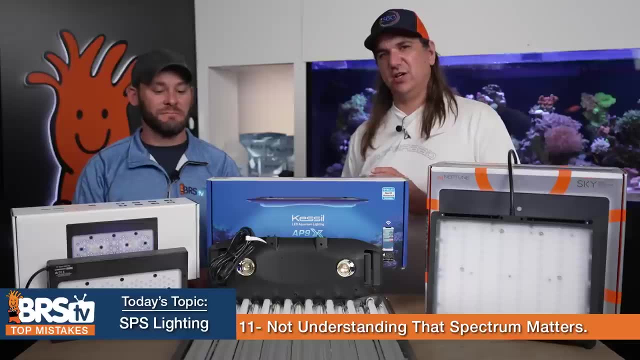 the future and actually give you like a preset option that already hits that area, right, right, uh, there's no more willy-nilly, just flip switches until I think it looks good now, optimized to the health of the animal you're trying to take care of. uh, and so? 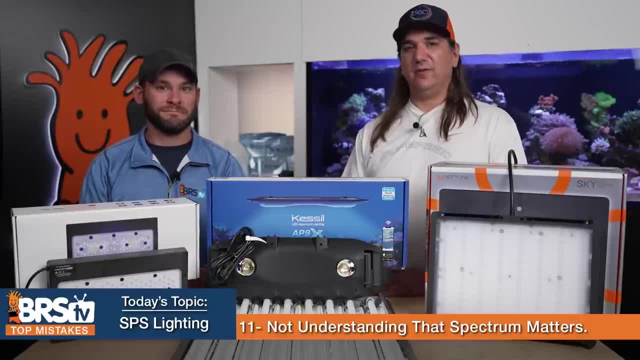 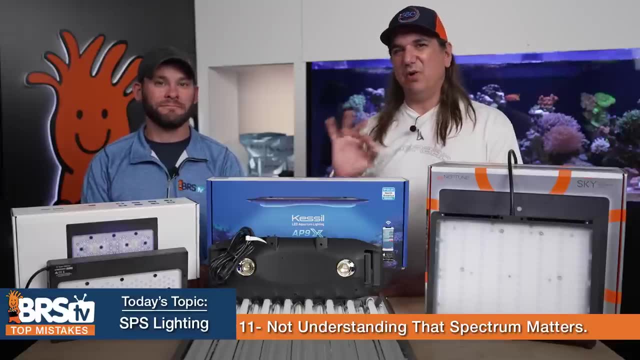 when I say spectrum matters, not only is it that the light's capable of the? uh, the right spectrum, which is like almost any good option out there, will do a various degree of that, some a little bit better than others, but all of them will support life, uh. the difference here now becomes: 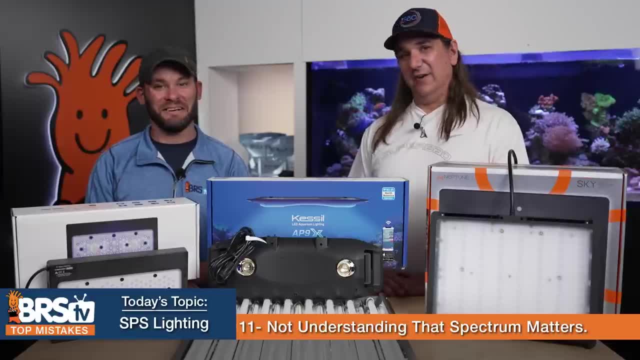 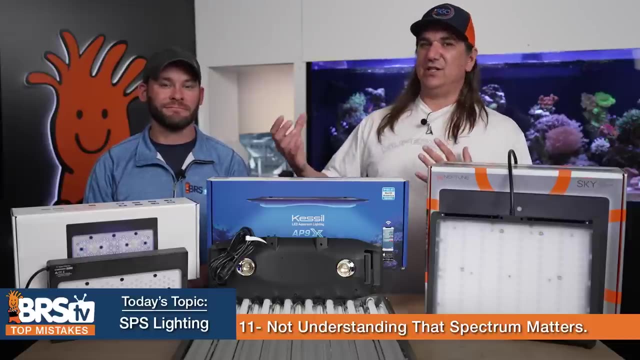 like: all right, stop messing with it first off, if you're, you know, tweaking it all the time and changing it, the animal will never be able to adapt to that. so it's changing, you know, the different pigments and concentrations of chlorophyll and different things in it to adapt to the light that you're providing. but if you keep switching it back, 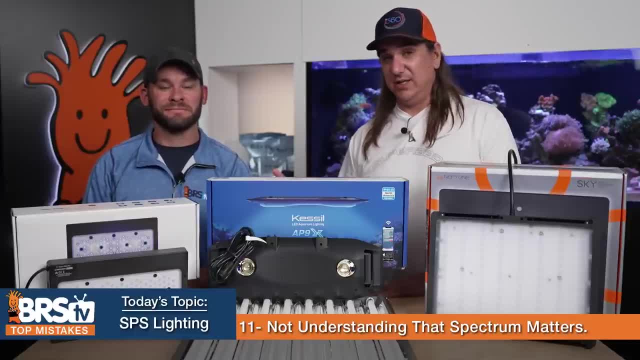 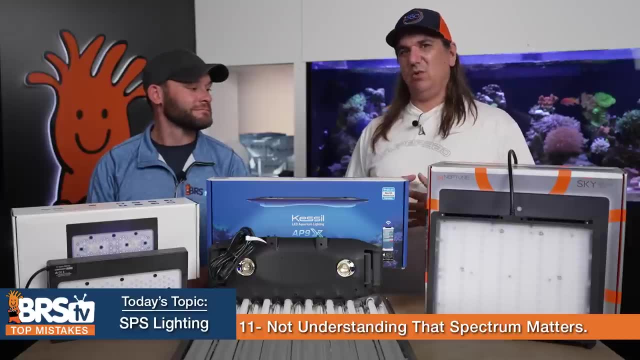 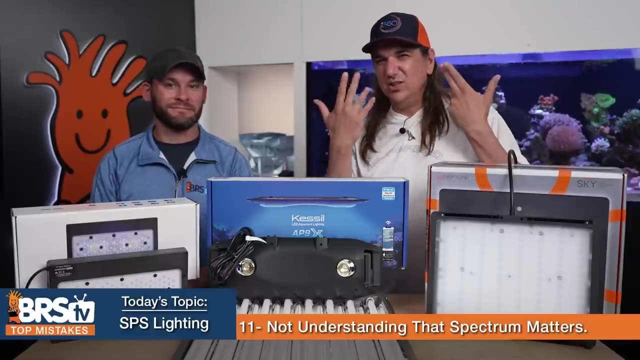 and forth. they will never be able to do that. so pick something and leave it there. a spectrum is number one but number two. you know, we're learning that, like you know, basically what we were doing before was taking all these individual lights- uh uh LED lights- and they come out in a cone and we overlap them enough and we visually looks blended. 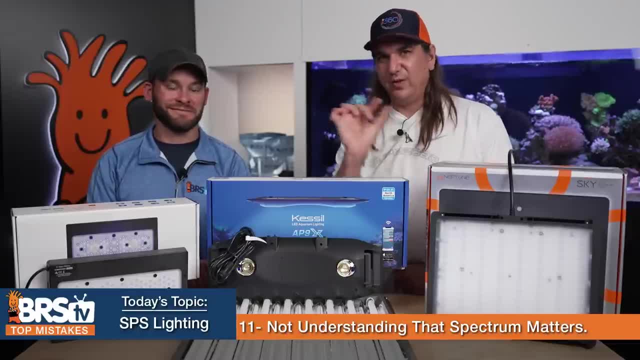 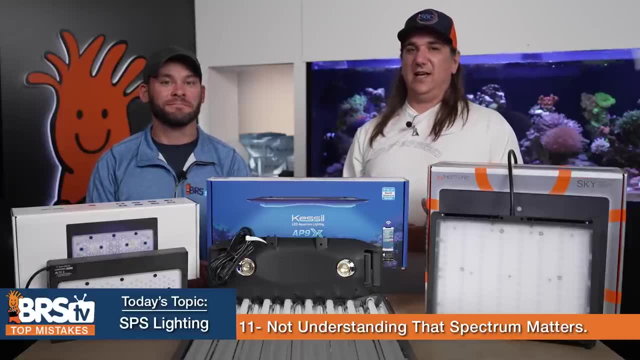 yeah, but I can look in the tank and see the little greens and red shooting all over the place, which means it's basically getting hit with little laser beams of- uh, different Spectrums. and so now we're finding that, you know, diffused approaches or similar types. like Castle puts all the LEDs under. 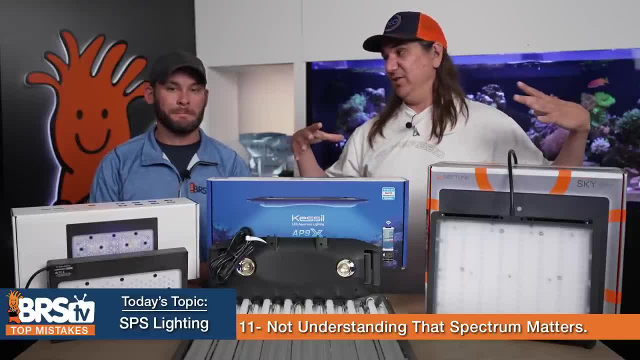 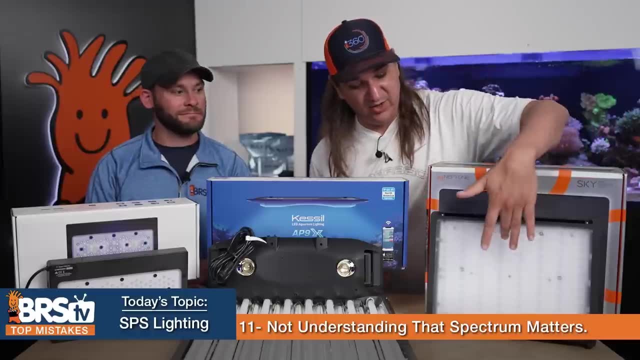 a single lens, which actually does blend them pretty well, like, in fact, better than any other LED we've seen, but also the diffused approach, where you put all a grid of LEDs, like the sky here, under a big giant diffuser. same thing with the frosted approach from. 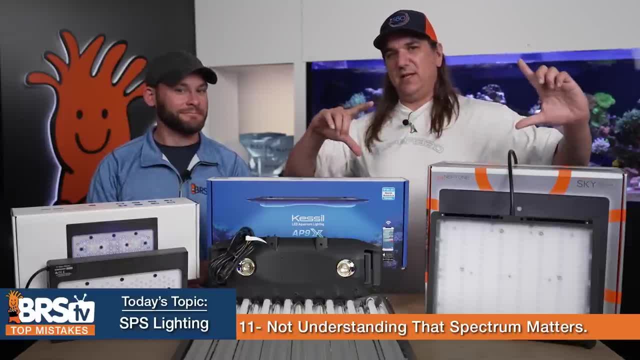 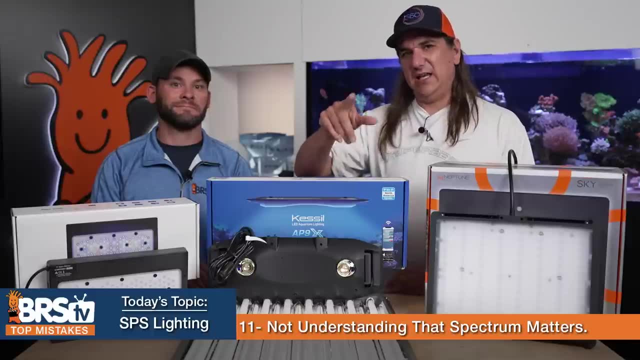 the Radeon G5 and they have a diffuser. but diffusing it now blends all those individual Spectrums uh, eliminates all the little Spectrum laser beams and I'm not hitting that animal with the wrong Spectrum, especially at top. yeah, so that is definitely one of the things that we've seen. 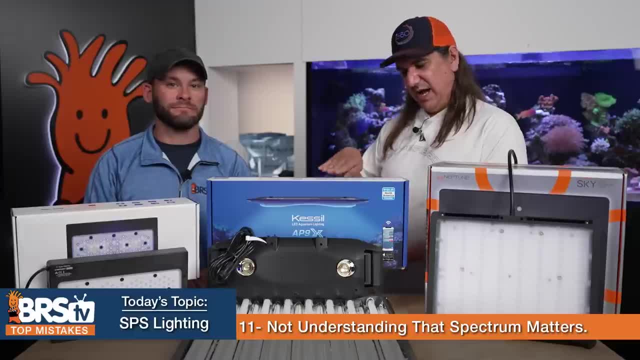 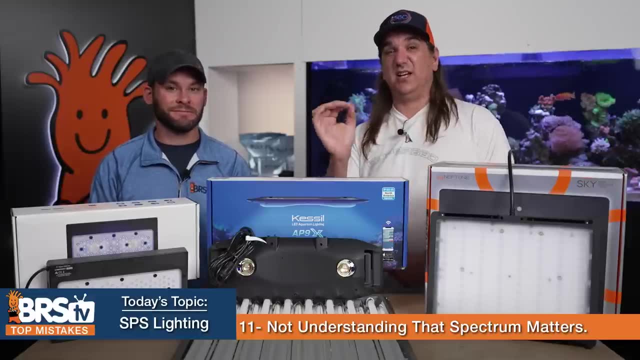 over the years is that, you know, down in the bottom half the tank it really didn't matter as much, but a lot of the corals that grew to the top would grow up there and then they would start to have challenges and it's because they're getting hit with the totally wrong Spectrum mix in. really, 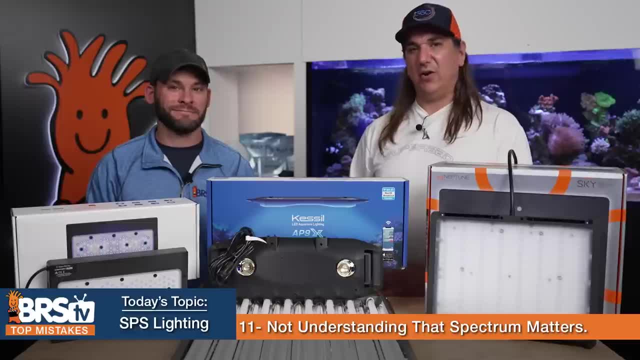 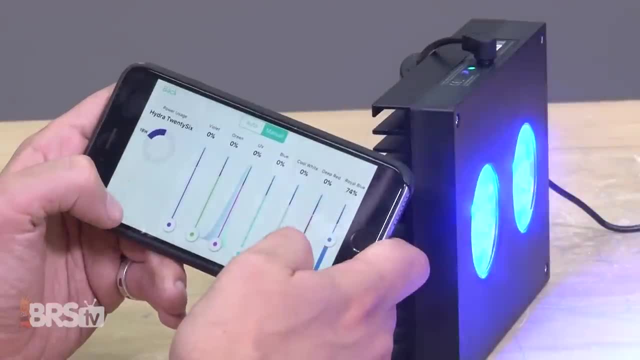 big intensity. so you know, Spectrum does matter and we're getting better and better at it. you're seeing, the manufacturers are doing the right mix of LEDs. they're giving you help on a set, a setting for them. they're blending it properly, all of these things, and finally we're stopping to flip the. 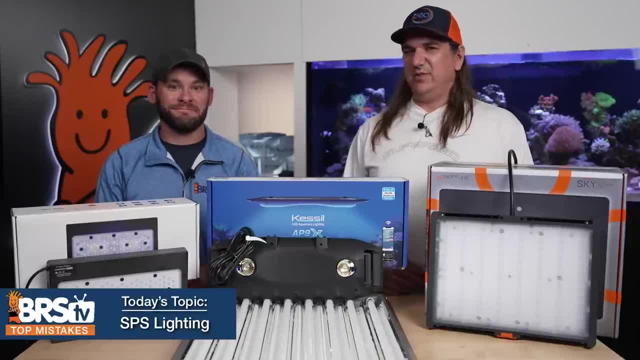 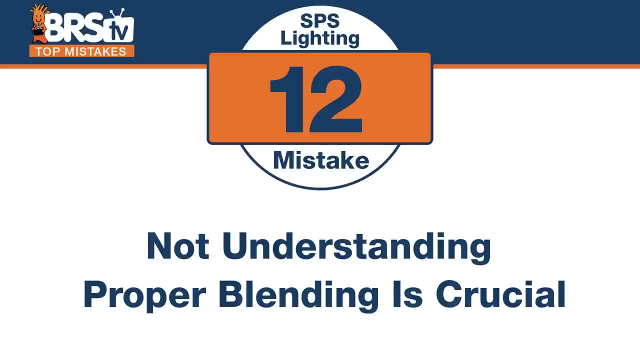 switches and treating the apps like their toys. all right, number 12. sometimes I uh steal a mistake. uh, mistake is not understanding the proper blending is crucial. uh, just like you were saying, um, if I get think of, if I was outside and the sun wasn't blended very well or the atmosphere wasn't 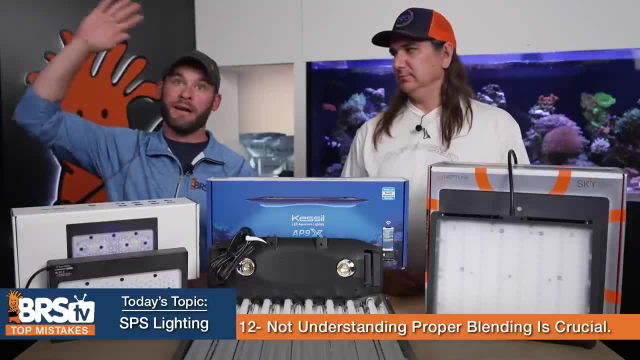 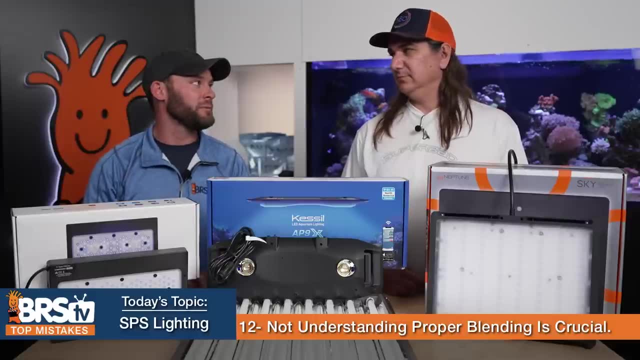 blended very well, and thousands of times a day I've got bright red coming across me and then every once in a while I get bright green, and it's just doing that hundreds of thousands of times a day. I wouldn't be happy outside either. this is such a great analogy, all right, but you know what? what if? 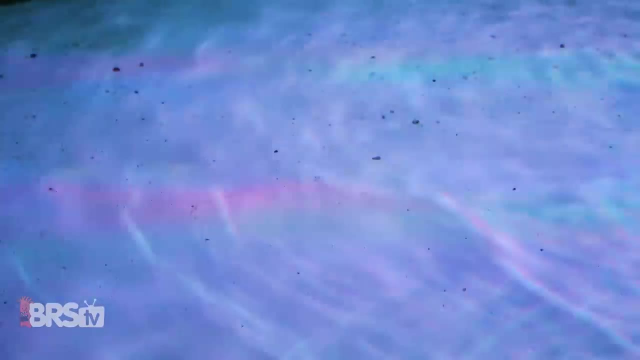 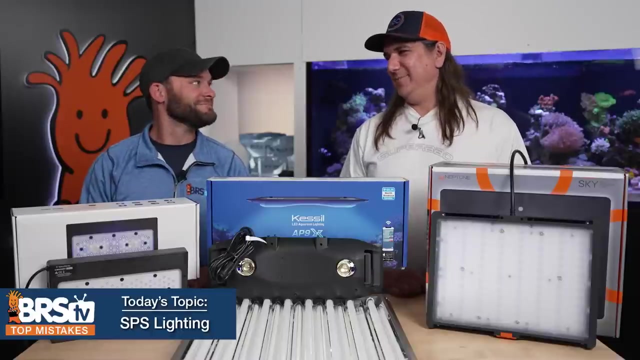 a big stripe or focus beam of UV hits you, I'd probably be toast instantly. you can understand why this is bad, yeah, so uh, yeah, it's, it is blending them and this is definitely one of the evolutionary steps in LED lighting and achieving our goals 13.. oh man, another Thunder Steel. the mistake is not understanding that stability. 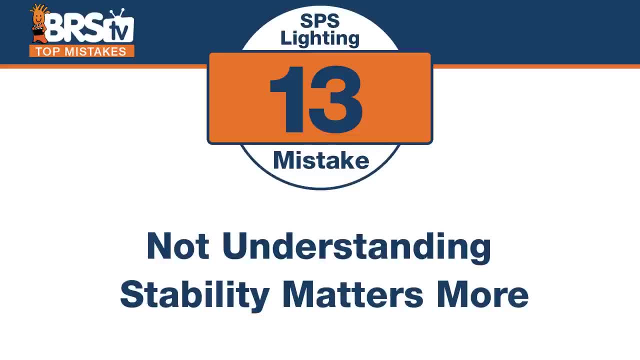 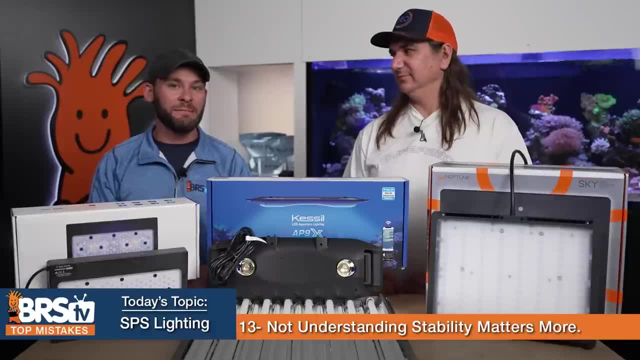 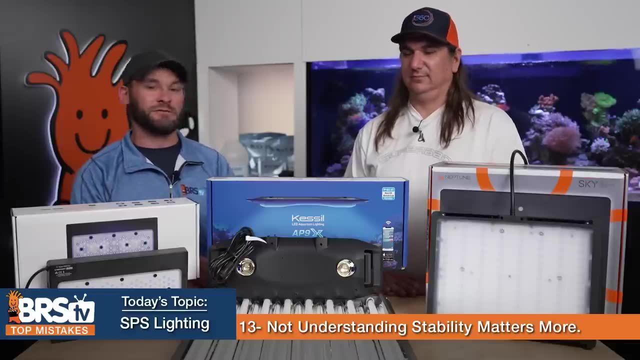 matters more so. that is not only the Spectrum blending, where I have a steady, stable Spectrum hitting me just like I'm outside in the sun. adapt to that. and on top of that is- you know you were talking about flipping switches and whatnot- and this is one thing that WWC Vic you know turned us on to when we were making the BRS WWC hybrid is. 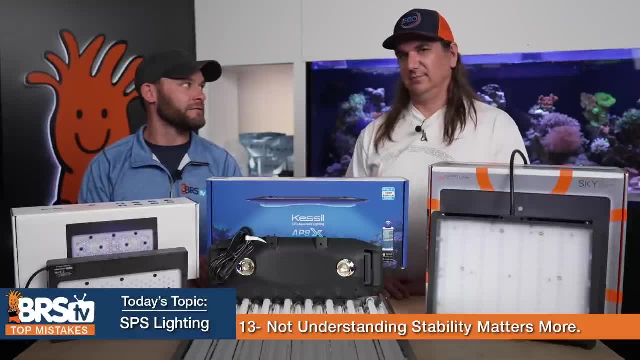 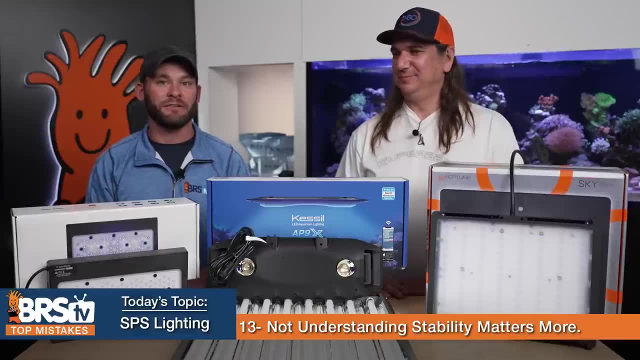 set your lights and don't ever touch them, forget they're there. they set them once and do not ever touch them once again. I mean, that's what's one thing about the T5 technology- metal halide technology- is you set your T5 bulbs, you got your your mix that you like. it looked good to you and 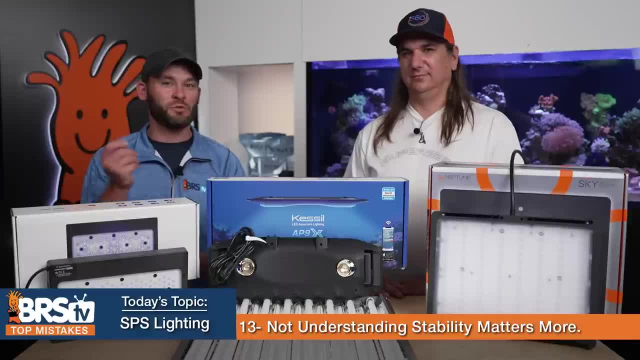 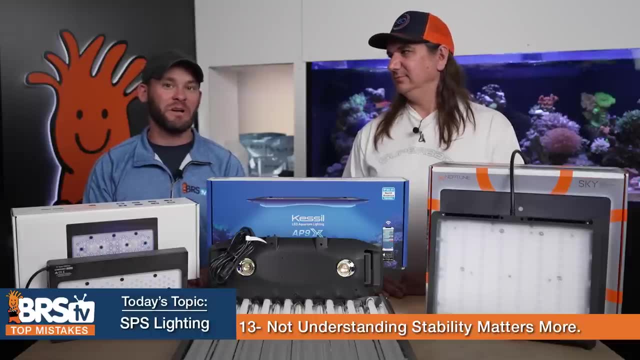 you just wouldn't touch it for months. you change out the same bulbs that you had. you were swapping out all different colors of bulbs and playing around with it. your metal halide, you know, you know, you know whether 14k bulb or 20k bulb didn't change at all. all right, so I'm gonna 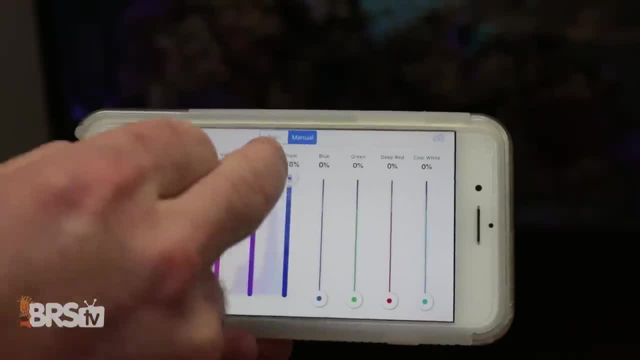 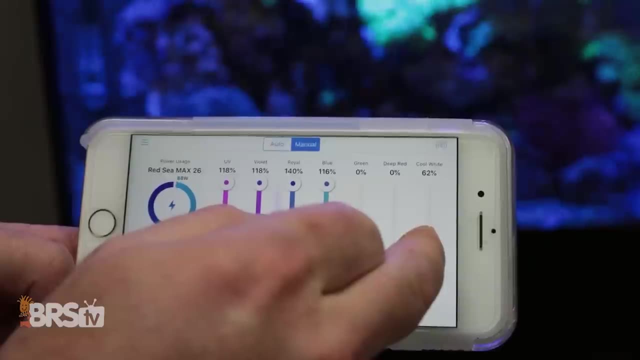 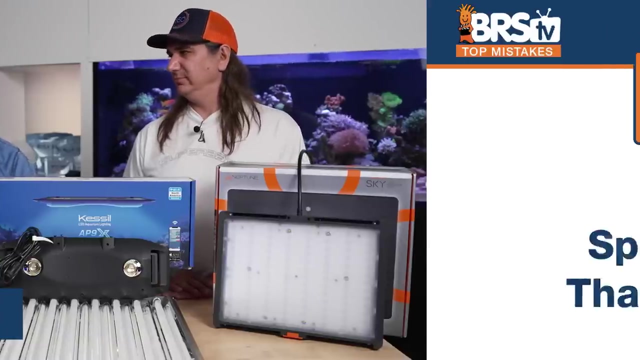 say it again: if there's one thing that you heard today like, you're like I really want to have a successful tank and I'm looking for one tip that says uh will help me the most, it's set it up to something good and leave it alone. all right, number 14, there's dollars involved, yeah, so the mistake is. 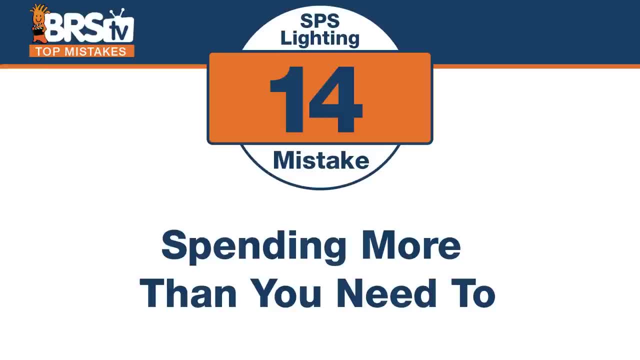 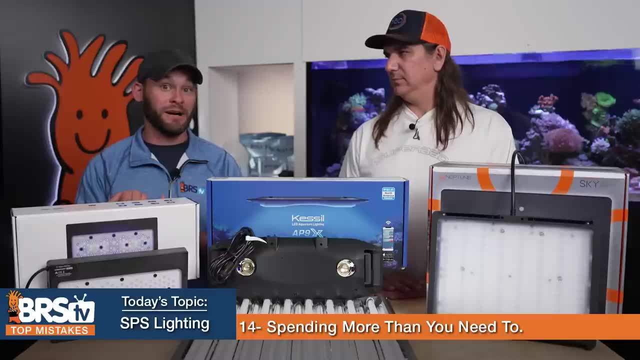 spending more money than you need to achieve this. there's multiple ways to do this. on the lighter side of the wallet: T5 fixtures- older technology like that is, uh, pretty cost effective and easy to get a hold of. um, you know even multiple small lights like the AI Primes. you know these things. 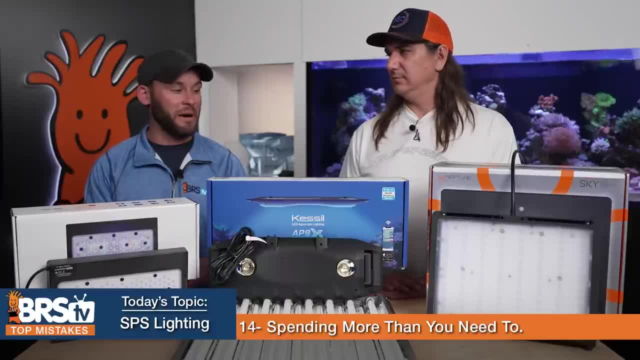 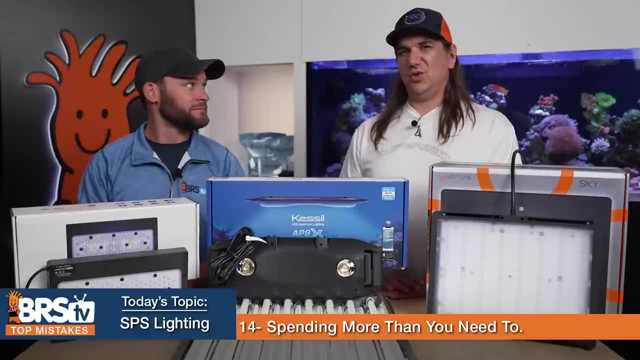 are like 200 bucks a pop. so get four, six of them and you're about the, about the price of a single fixture of one of these larger ones. but you're actually doing better at spreading the light out. um, think about your goals. uh, not like one light is better than another light, because that's not. 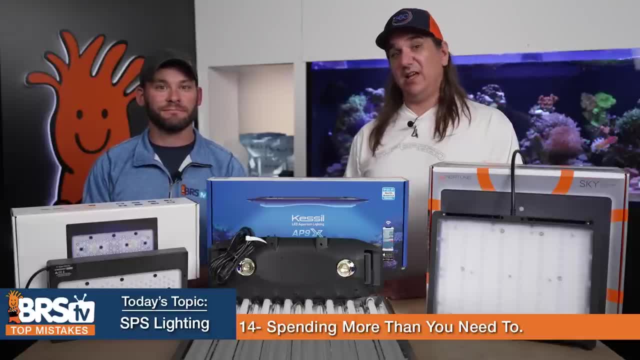 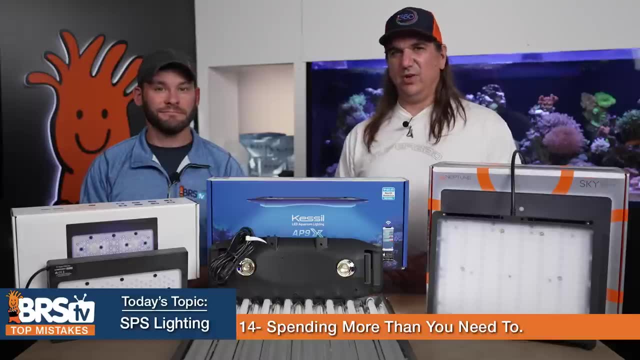 necessarily true. uh, it's how you use the light and how many you need. and then, uh, what do you achieve when you buy these things together? so, uh, you know, not getting tied down to one light or another, but, like you know, some of the ways that I've found have actually been the cheapest of all the things. 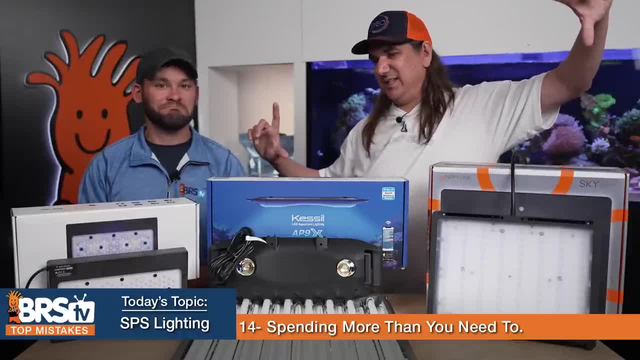 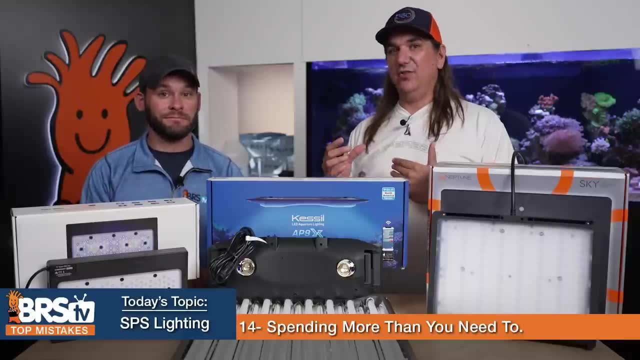 that we've talked about is actually the big form factor lights like the T5 and probably even in the sky. well, the price point of the sky is high for the application. if I look at other things that are going to achieve that same kind of big form factor light, 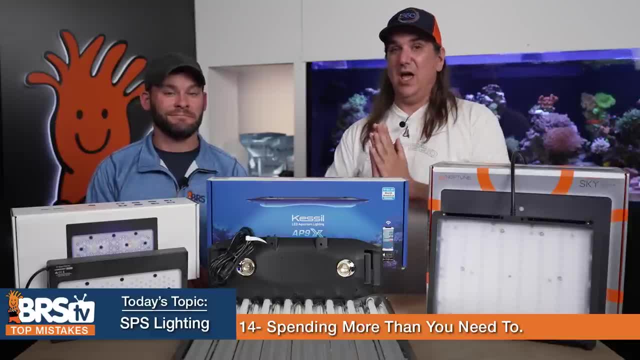 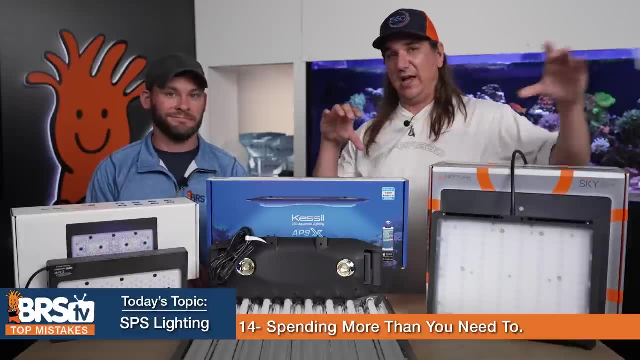 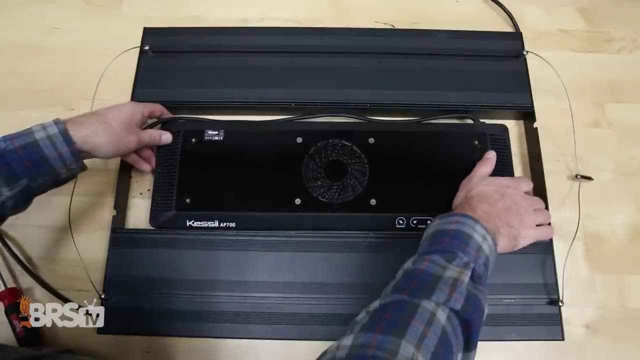 in the power range they're probably going to add up to something more. in my case, in a similar price range, is actually the Kessel a360 and then with the fill light, adding in either some LED bars, but more specifically inexpensive would be the aquatic light fixture like the one on the e170. so in that, 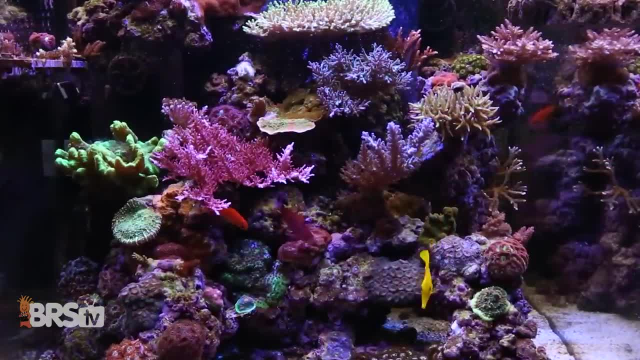 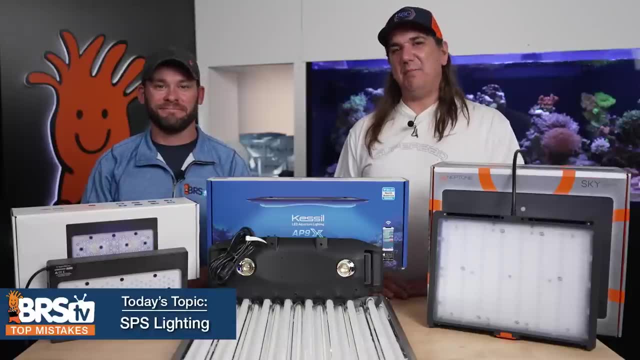 case, my goal is: not only do I want it to, uh even light that covers from all angles. watch it look awesome, and shimmer is part of that for me. number 15: if you're not buying T5s, do this. the mistake is not using a par meter, and well we. 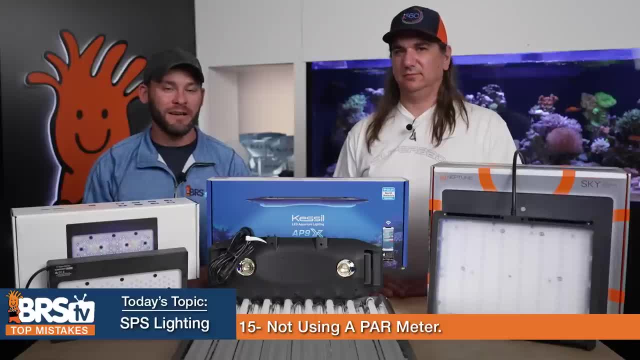 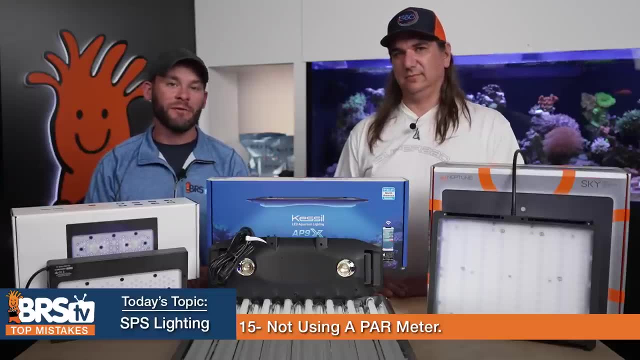 have goals. we'll be talking about them here in the next couple mistakes. but the par meter is the way that you set all of these up, other than the T5s, which we already know mounted eight or nine inches, plug in and go. the rest of them have the capability, a bunch of them have the capability to go way. 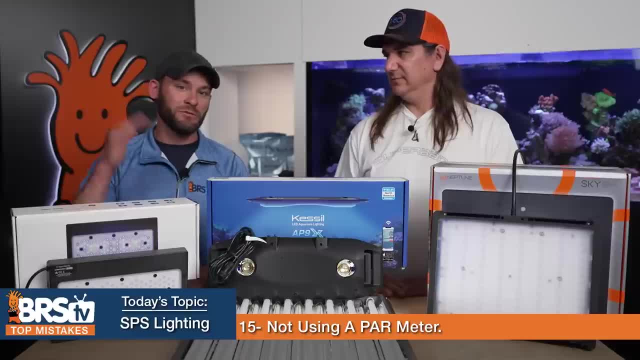 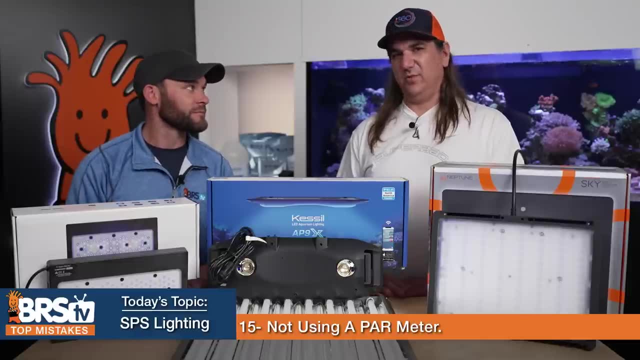 higher than what our corals need- uh, and you don't want to be too- or lower than what your corals need, so there are some sweet spot ranges in there. just make sure you're testing it so you know where you are. there's a tip with hidden within. 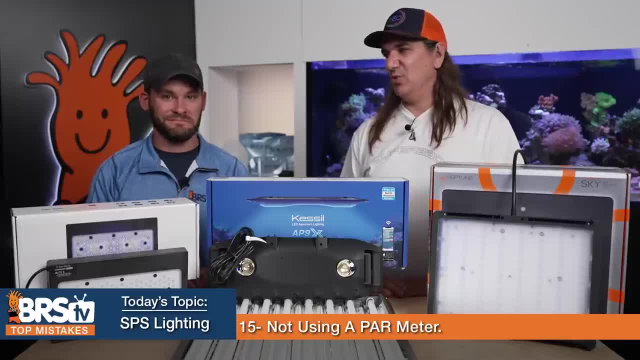 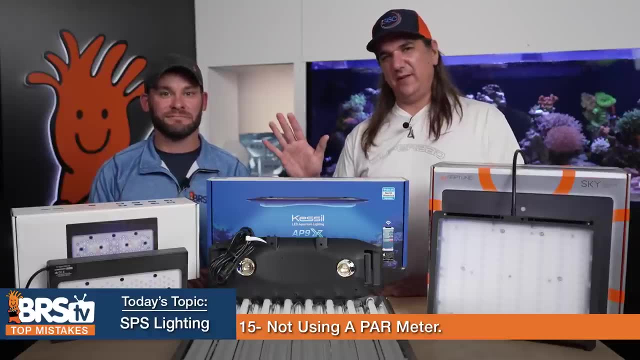 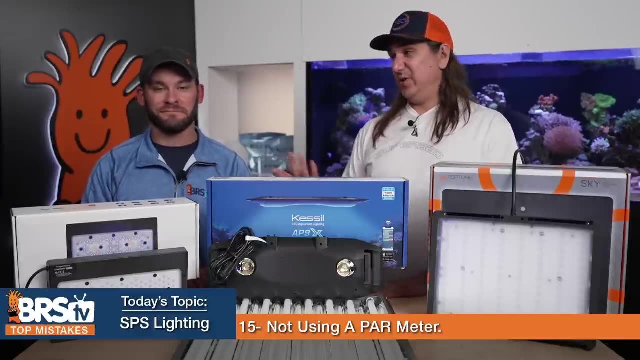 the tip here, which is, uh, going too high is a hundred times more likely to kill the coral than going too low and rapidly, uh and so, uh, it's at 200 to 350 par range, and so, if you're asking how to set this thing up, it isn't just like willy-nilly. uh, you can emulate. we, we share some power data in a 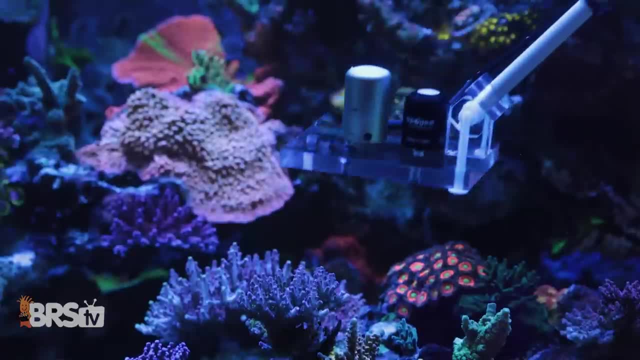 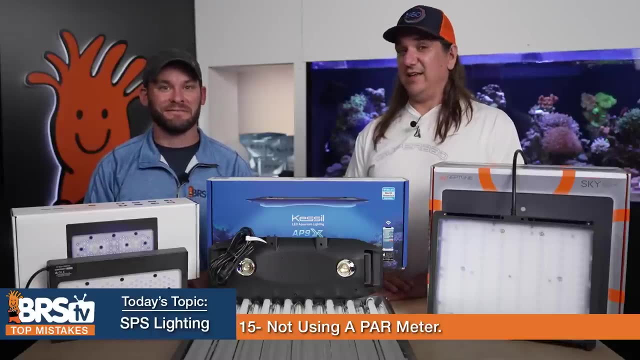 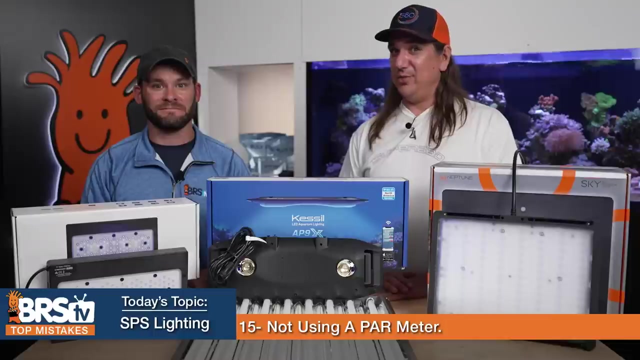 lot of ways so you can try to emulate, but you know, picking up a par meter is actually one of the easiest ways to do it. and hot tip here actually is: uh, at BRS, at least currently. hopefully you guys will use this and it won't change in the future, but uh, we actually allow you to return them used. 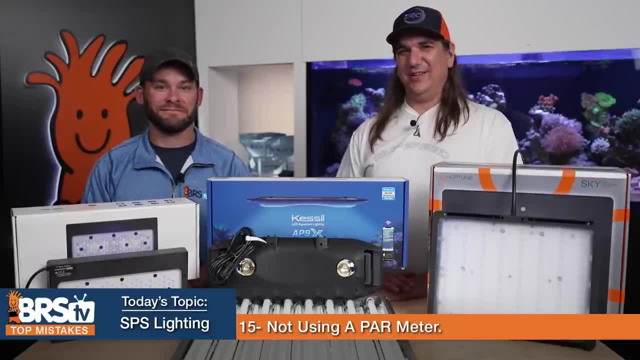 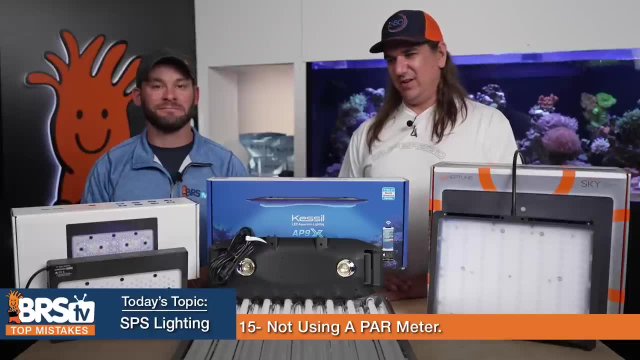 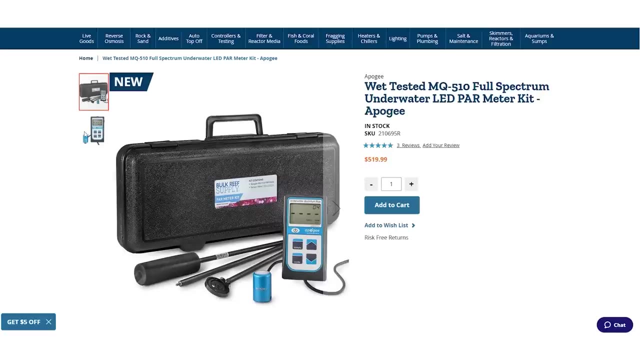 uh, yeah. so uh, they're called wet tested at the moment. we'll see if that name sticks, but uh, yeah, it will. I think it has like a 20 percent restocking fee, but you know you're going to invest a thousand bucks in the lighting. uh, you know what, spending 40 bucks, uh, on the par meter. I think that lets you. 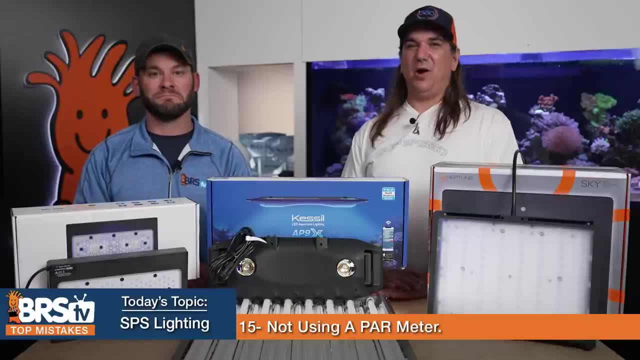 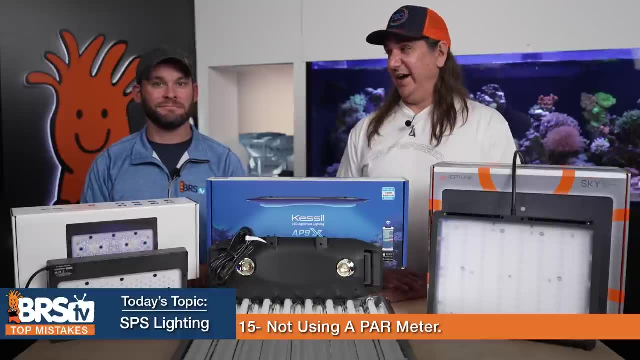 return it for up to like a couple of months. so we used to have a part rental service and you had to return it in two weeks, uh, and it's to cost like about the same amount of money in this case. now you can just buy it and uh return it whenever you feel like it, uh, or within a couple of months at. 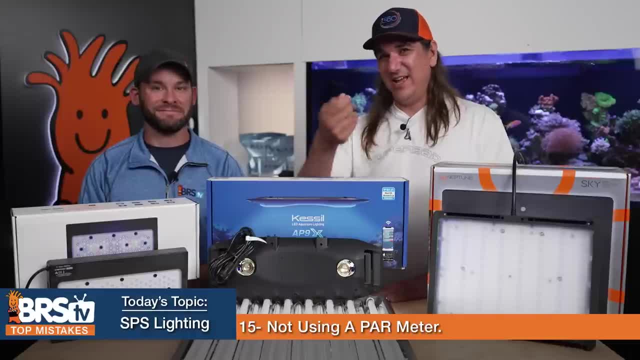 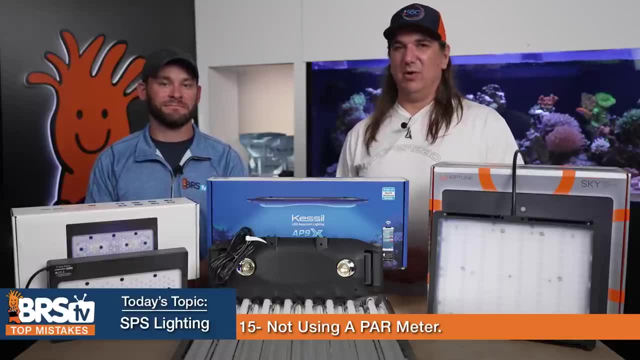 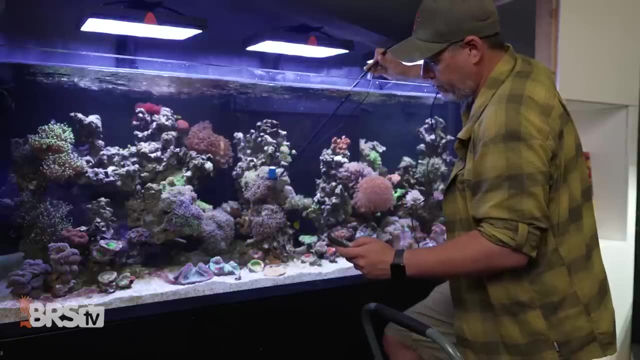 least and uh, you know what- have- be able to measure it, uh, and get these things tuned into the right way. uh, and for us, you know, I know a lot of people don't want to buy a 500 par meter and it's a barrier to success. yeah, so that's why we're trying to find unique ways. maybe the return service won't. 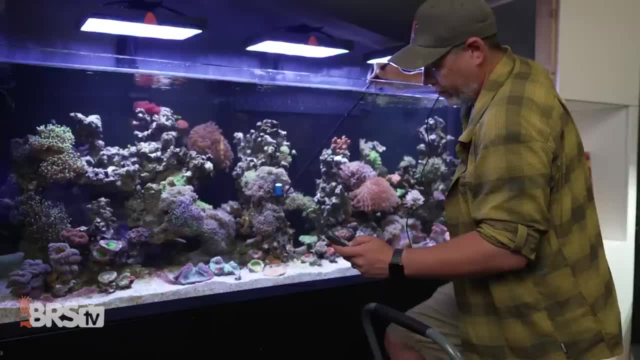 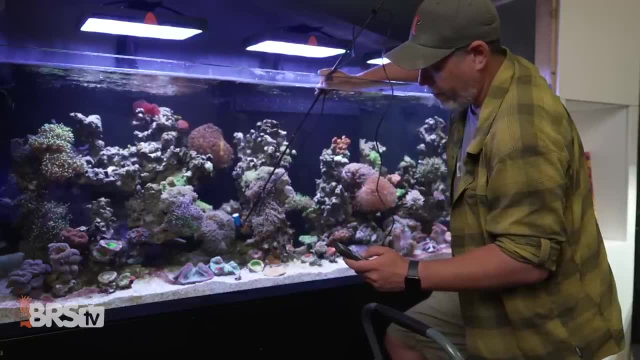 stick around, because this video will probably stick around for a long time. but come and look and see what we're doing, because we're actively trying to find ways to help you set up these tools right and do it affordably as well. number 16: the Thunder gets stolen again and again, and so the 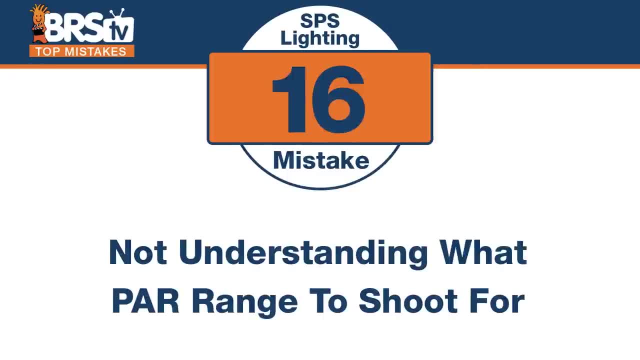 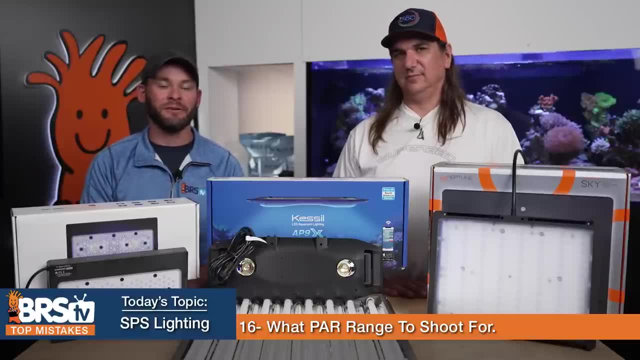 mistake is not understanding what range you're shooting for in your contaminated system and you know, after testing WWC tanks by hand a whole bunch of times, testing our own tanks, that are successful here. 200 to 350 par is that pocket range that we're aiming for. but 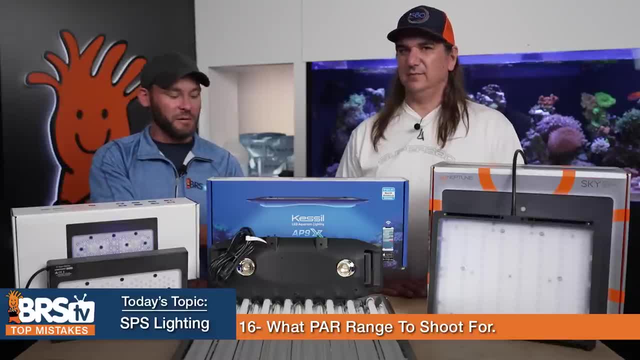 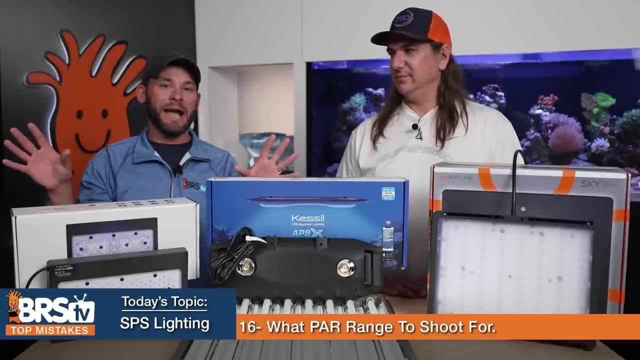 you might have spots at 500, 400, 450, and then spots down in the corner where you're at 75 or 50 or what have you. but the goal is as many points as possible, on average between 200 to 350.. so if you 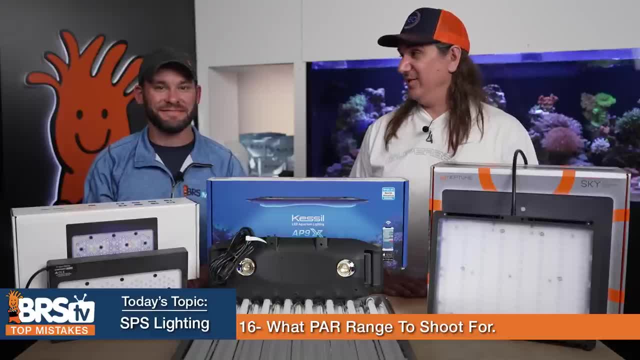 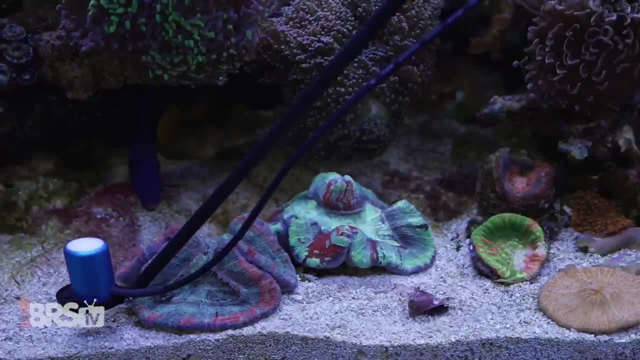 heard that range you're like: ah, all right, I know I gotta go get 350.. everywhere in there, because that sounds like the best, most horsepower possible. uh a, it's kind of hard, but also it. we're talking about the range that does well in. so if you're gonna shoot for 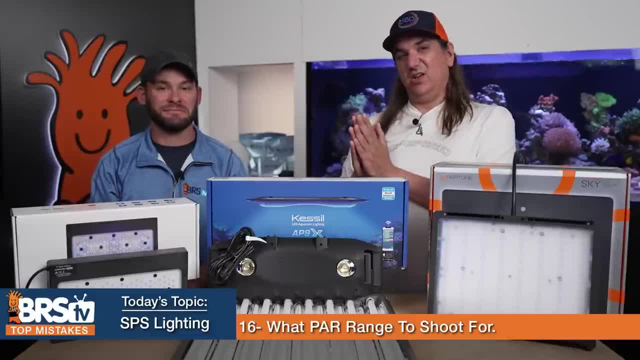 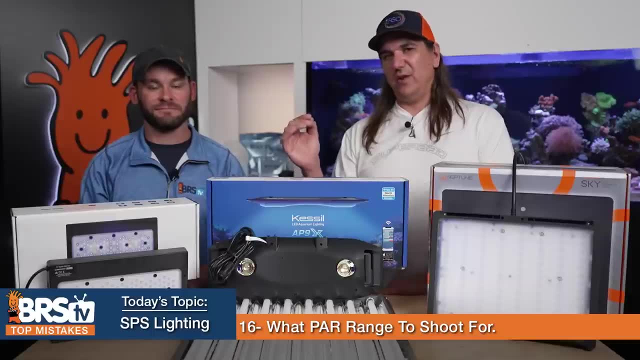 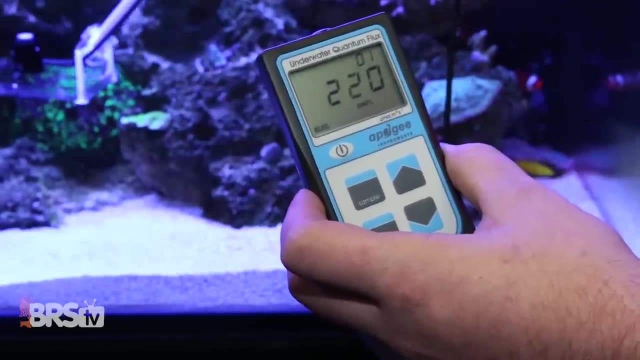 a goal, shoot for the middle actually. so you know, somewhere around 275 is probably that range, and each one of these corals will do better in different areas. so shooting for that range, like the 8020 where they'll do the best, is the goal. if you shot for 275 everywhere, it's probably better. 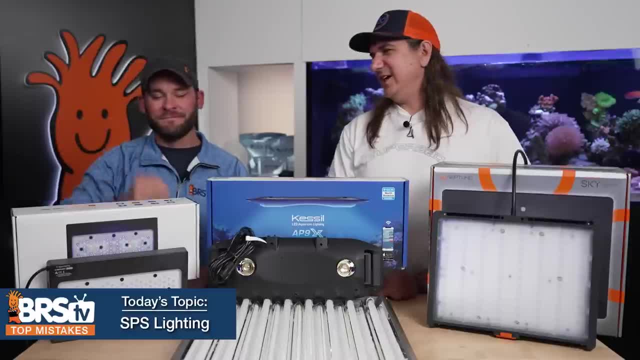 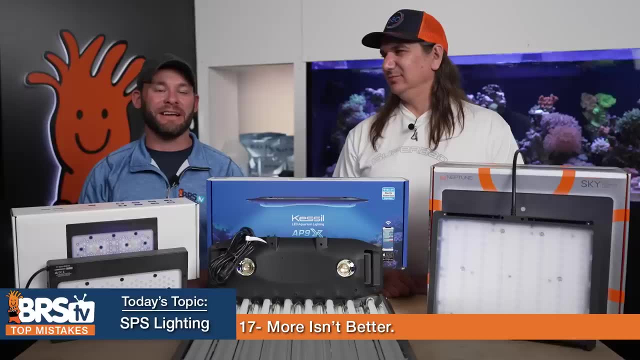 than 350.. more is not all right, always better, all right. number 17: I've got a problem: more isn't better, so more par isn't better. and you know that was when LEDs- it was all about LEDs first coming out- uh, par Wars, I can this thing. 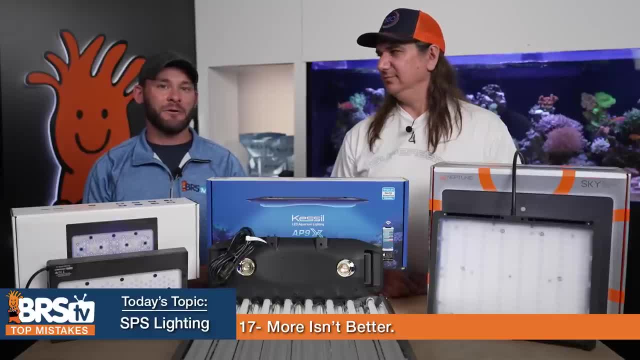 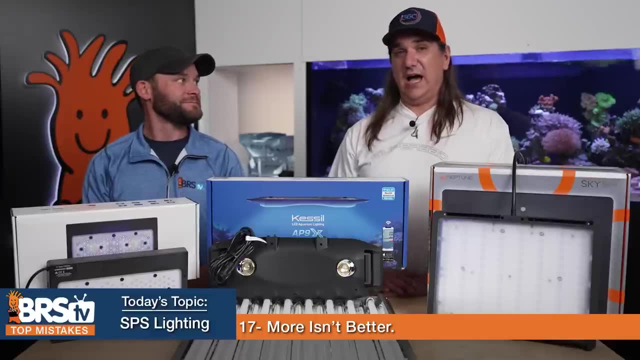 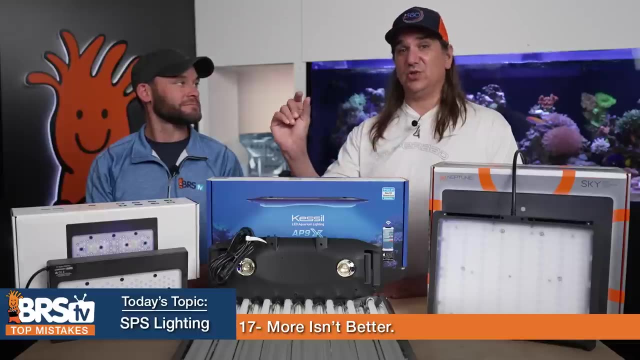 can push. you know, 1200 par, 1500 par, and now we're back to. now. we need to be in that range and let's make the tool right for the purpose. so, uh, I will tell you that the guys over at Worldwide Josh is really good in 200, but they don't do good at 350, and the reason that they know that is they. 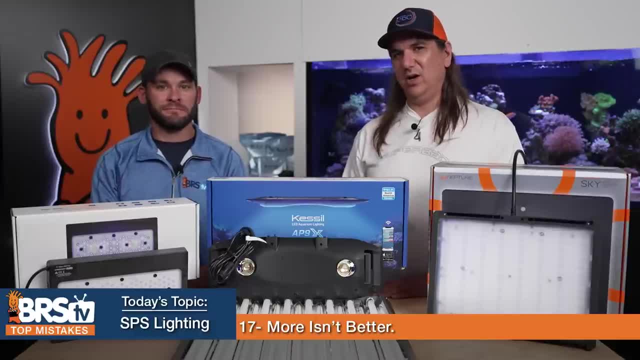 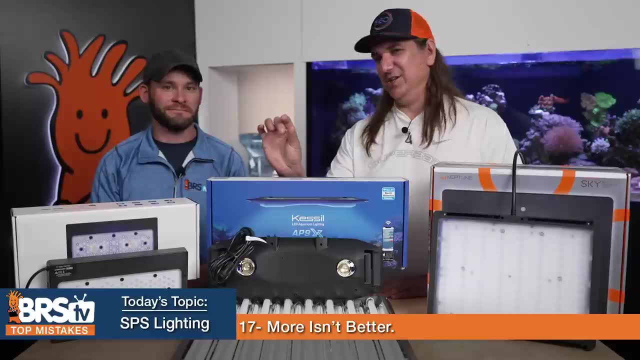 move them around, you know, and not like all the time. you know, like you know what this one just isn't really doing really well over the course of a year, let's spend the next year in a different location, a year not moving around by every month, and so one of the things you can do here is: 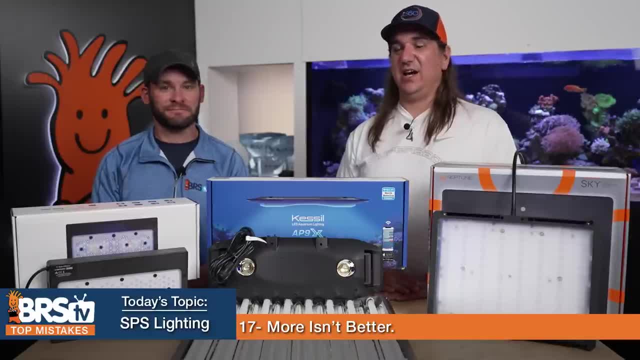 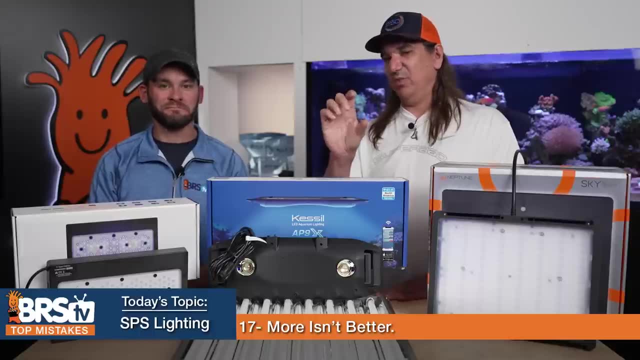 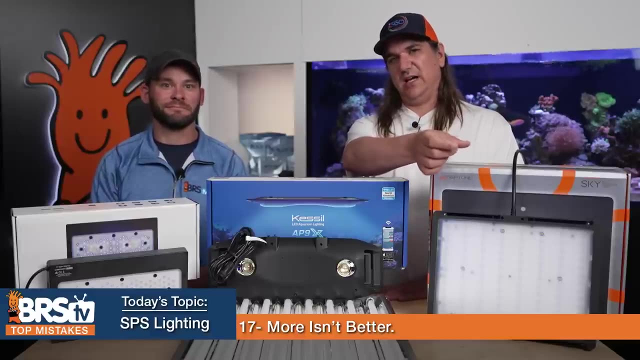 actually when we talked about in a different video, uh, the frag plugs. so instead of using a frag plug like the re, like a frag mounts from Marco, if you have a reef saver rock already, I can glue that piece of rock, you know, to the uh other rock and it looks seamless. and if I ever wanted to move. 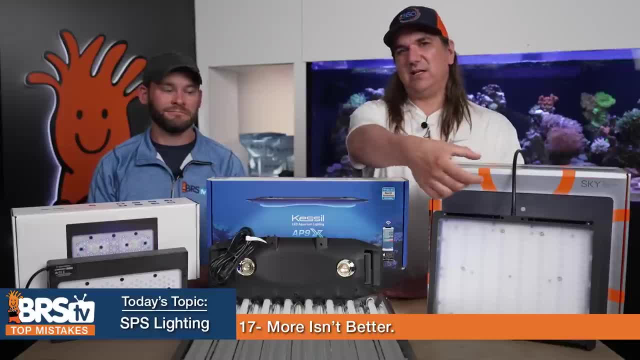 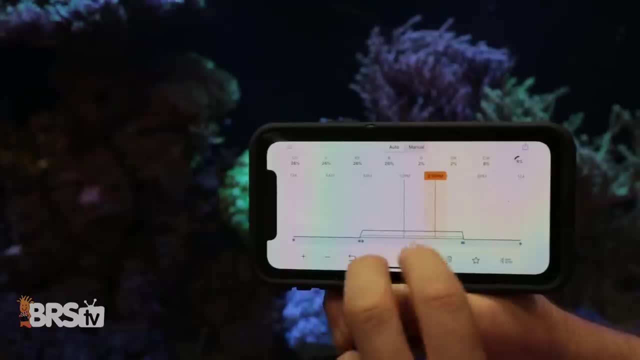 it now. instead of breaking the coral off of the rock work, I can just pop that piece of rubble off and move it to where I want, so it makes it a lot easier. so more is not always better. the right amount is better, and you know if you're going to experiment. experiment slow and long number. 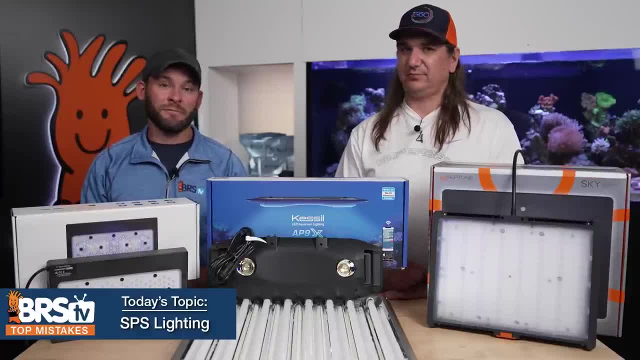 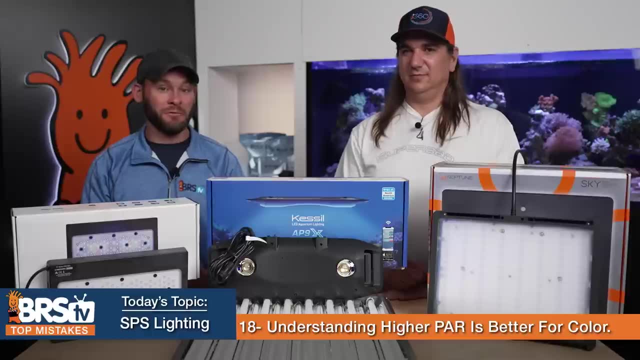 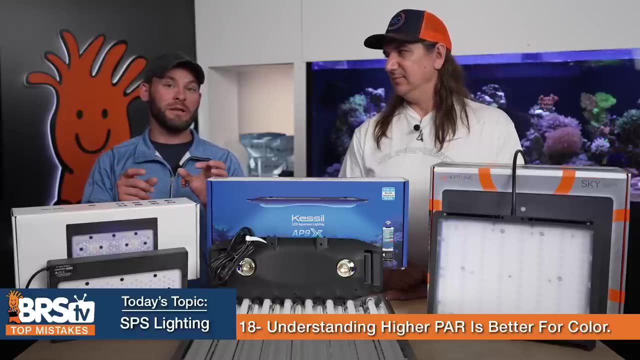 18.. one of the reasons that they move this stuff, yeah, so the mistake is not considering that higher par might actually bring you more color or differences in color and, if we've all know, we've seen wwc's stock and some of their corals. they're amazing colors and that could be from tweaking putting. 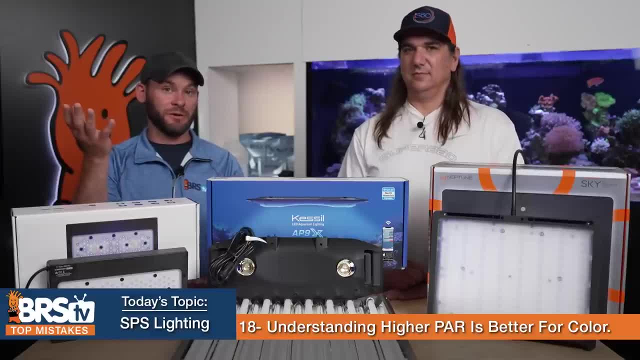 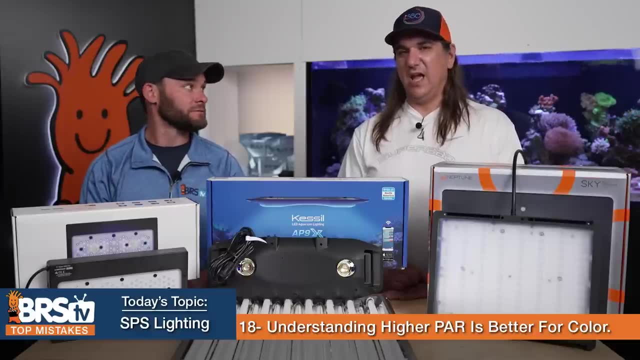 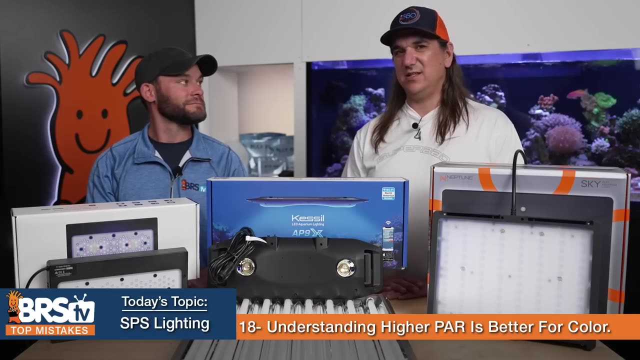 a little higher par and letting it sit for a year and find out what the colors and the morphs and what what fluorescence and stuff comes through, uh, or moving it a little further away from it if it starts bleaching out. so the general thought process or theory has not been proven out here, but what the common thought process is is: 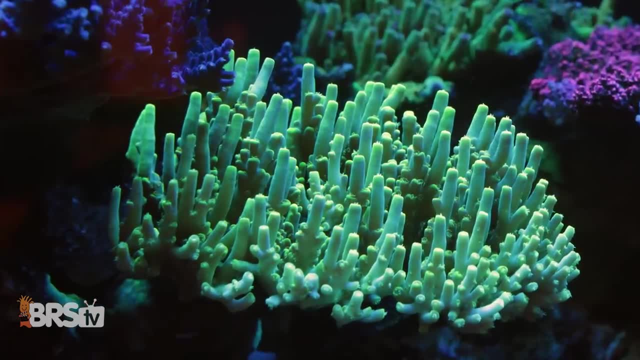 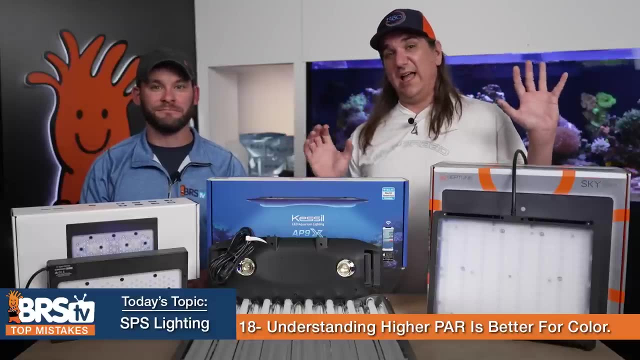 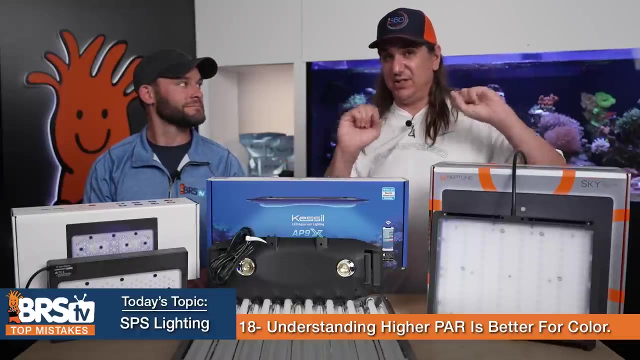 basically, you're going to exceed more color pigment and fluorescence because the coral is going to produce those fluorescent pigments essentially as sunscreen from really really high par. it's using those things to protect itself from too high light and if it's protecting itself and getting bouncing those rays of light back, what it's actually going to do is receive less of that. 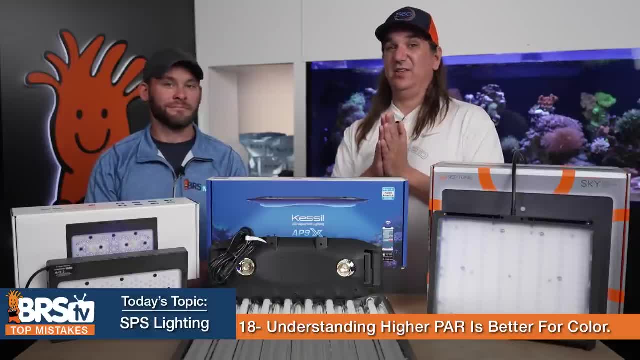 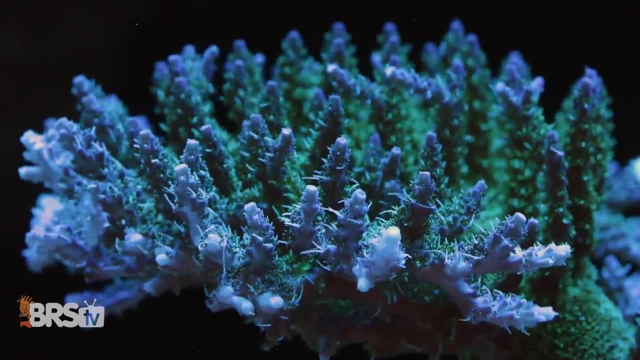 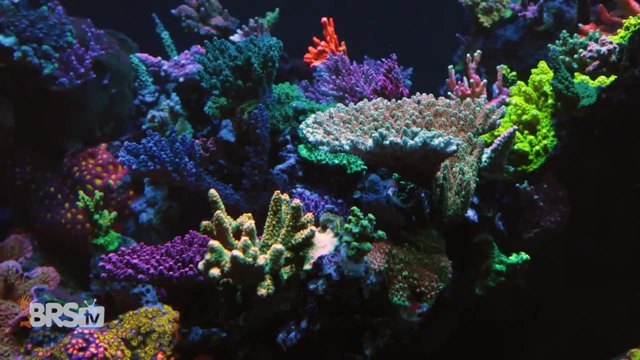 light and, uh, it will be able to photosynthesize better other than just getting bleached and burned out. so there are some cases where you know increasing the par will actually get better coloration and better fluorescence. but you need to know that you're riding the like razor's Edge here, and the reason 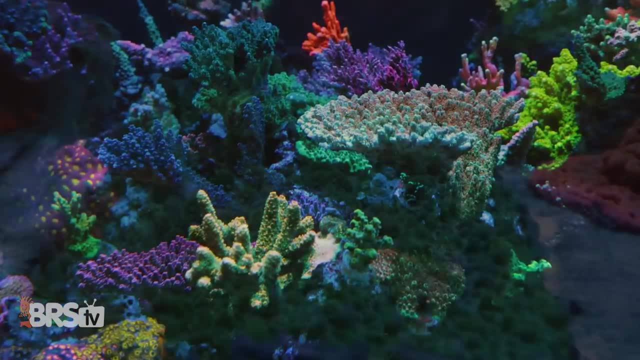 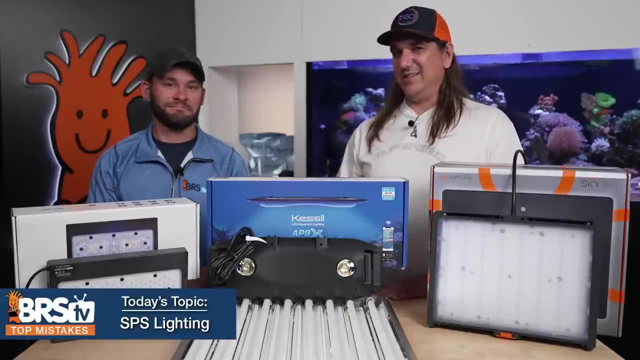 you're getting the color is because the coral is actively protecting itself from what you are doing to it, or at least that's what's currently believed, number 19.. there's a flip side to this. actually there, and making the mistake of not considering lower part for, uh, faster growth instead of 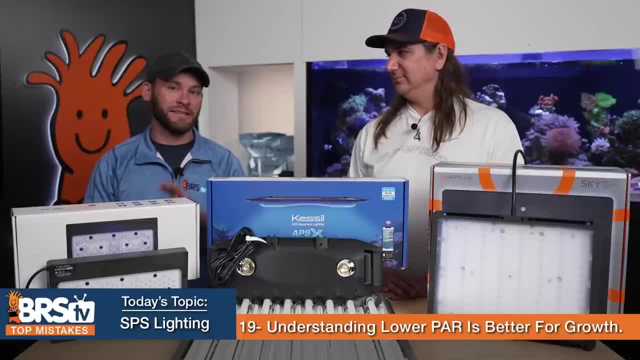 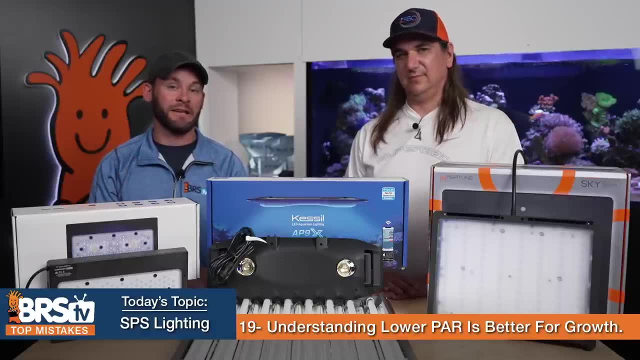 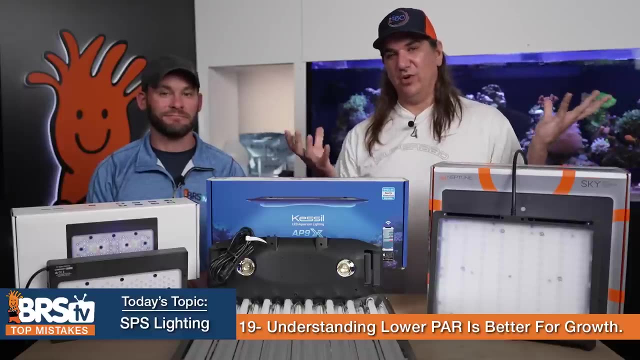 coloration. that might be a ticket. uh, you know, instead of protecting itself constantly from this bright light, uh, it's actually more adjusted to a lower amount of light and it can actually grow faster. yeah, so maybe closer to 200, it's actually able to absorb a lot more of the energy. 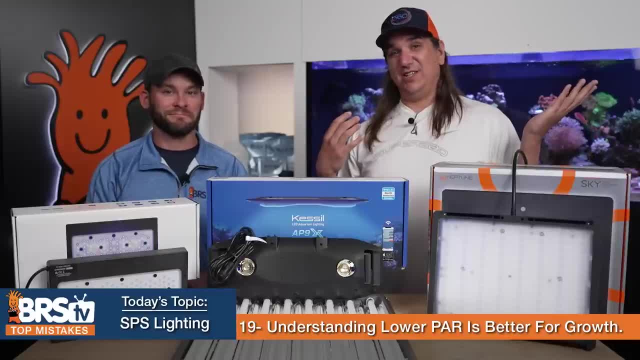 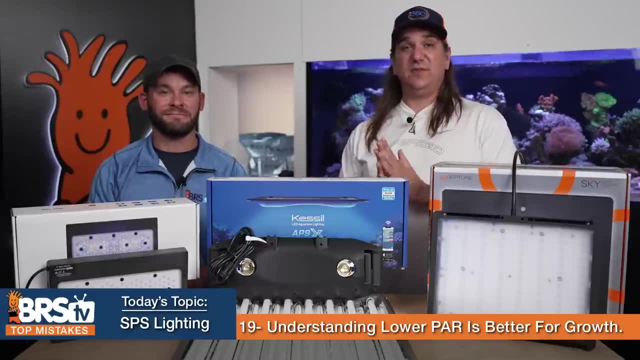 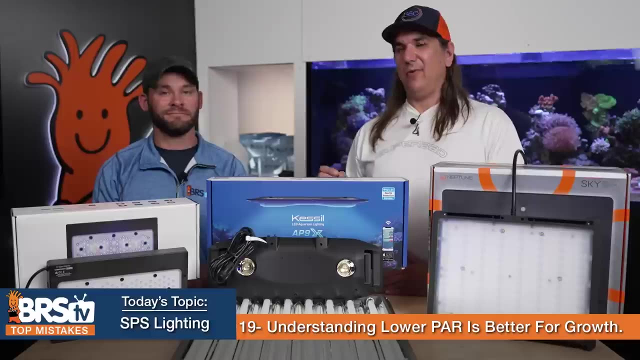 and reflect less of it away, and it's not producing these like suntan pigments. okay and uh, it's actually able to grow faster and so we've seen that in many corals at the lower range it'll actually glow, grow faster and you know you're not riding a like laser, a razor's. 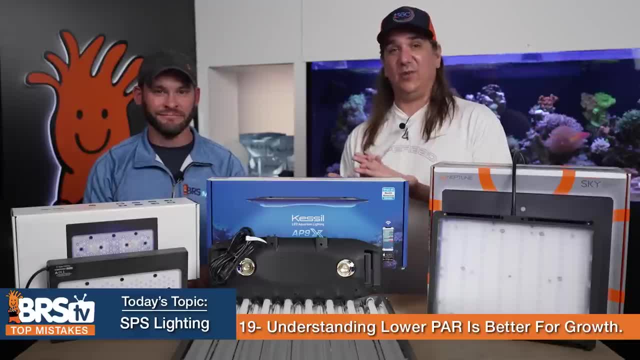 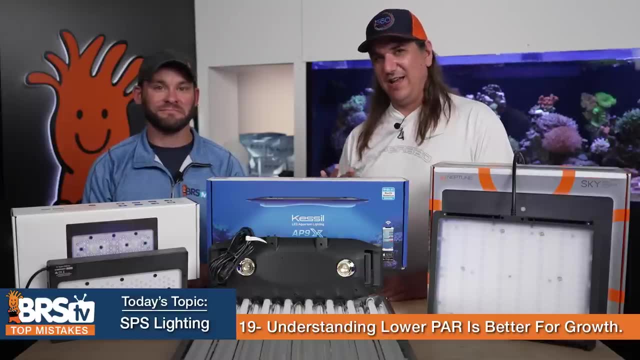 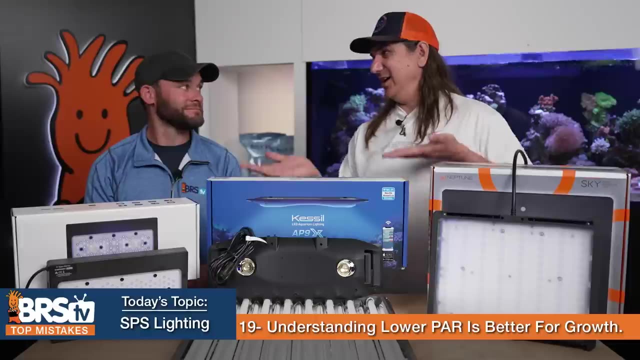 Edge there. as long as the coral looks healthy and it's growing, you're providing adequate energy to it. so you know, looks healthy, visually growing means you're providing enough. maybe you can get more color out of changing it, but what I wouldn't do is raise the whole lights all the way up and expect every coral in here to benefit from it, because it 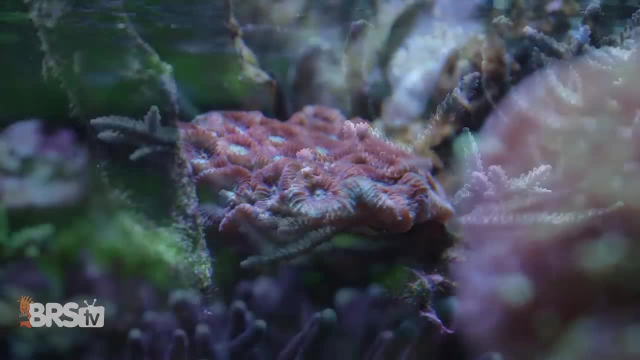 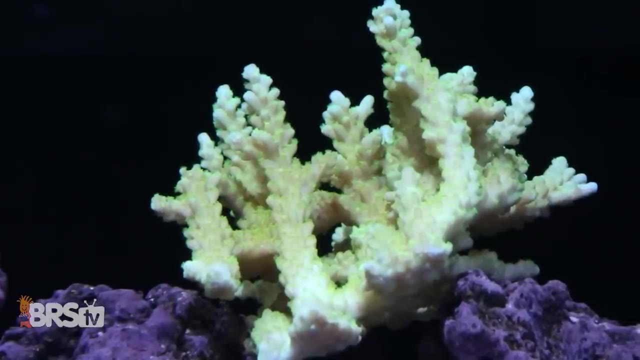 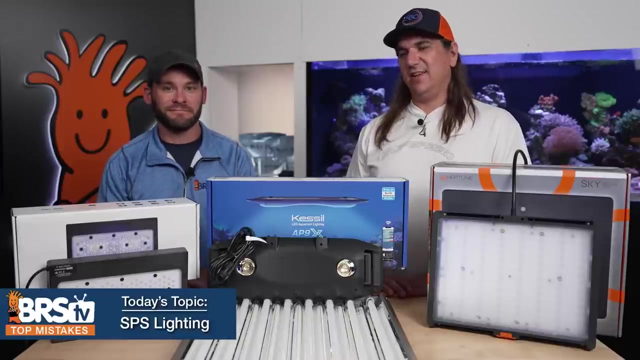 wouldn't. what you can do is move those coals around or, you know, if you have one of those Matrixes of like eight AI Primes in the top, yeah, you could actually start Zone lighting and creating areas that are higher par than others. all right, number 20- this is actually another one. if you 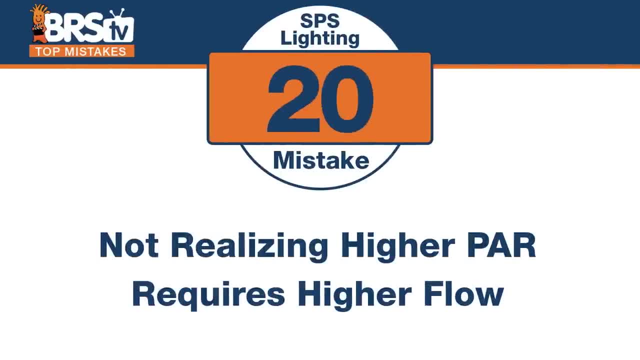 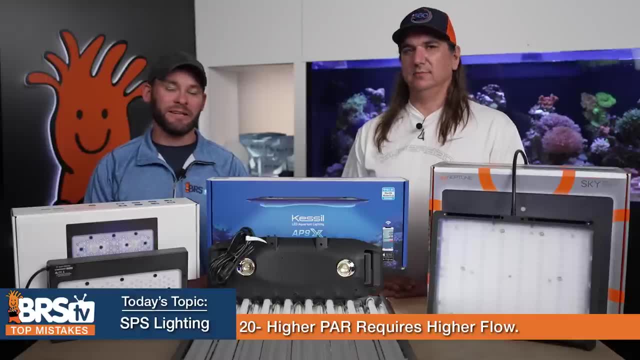 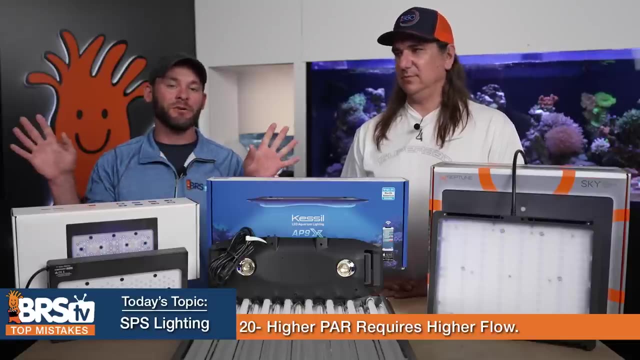 only heard one thing today. uh, let it be this. uh mistake is not realizing that higher par needs higher flow, and this is specifically wrapped around. the corals grow as they grow and then they develop the toxins and byproducts of photosynthesis, flushing it away from them. so 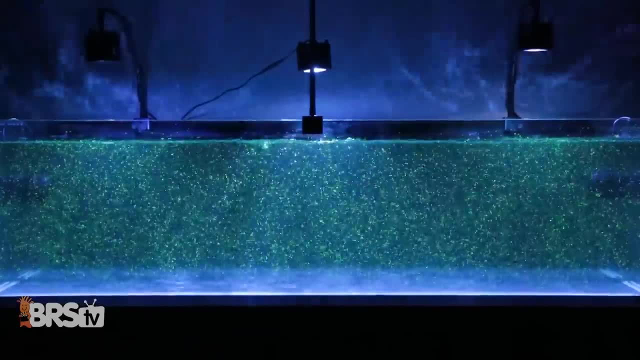 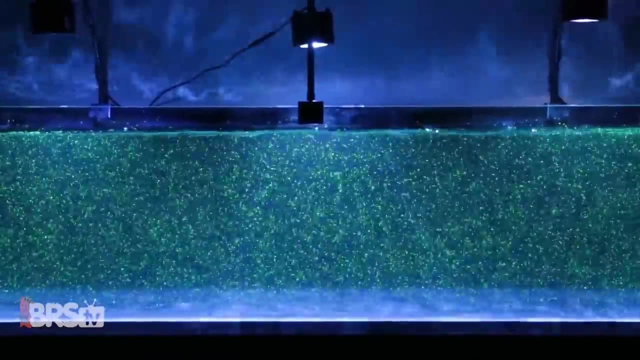 that they can get rid of it. yeah, basically, the more energy you're putting into the coral and the more it has to protect itself basically needs to get rid of all those byproducts. the oxidants are actually poisoning the coral and if you don't, it has no choice but to release it. 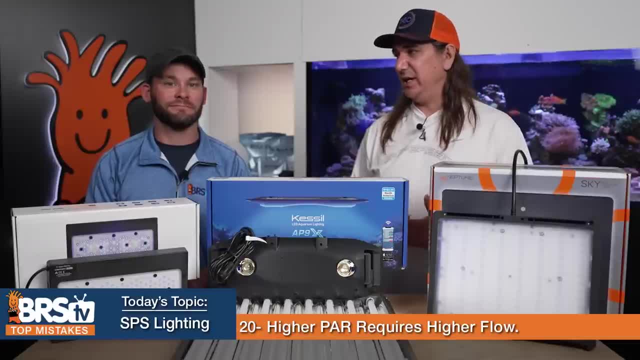 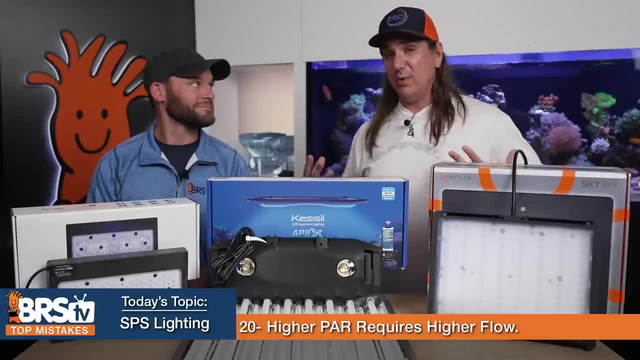 really into the water and it'll probably die after that. sometimes you can get it back, uh, nurse it back to health, but basically when it bleaches, what it's doing is saying I'm producing too much energy, I'm not able to get rid of the negative byproducts and oxidants of that, and, just as a desperate 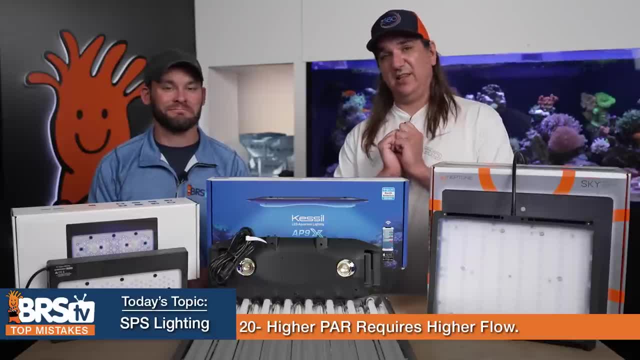 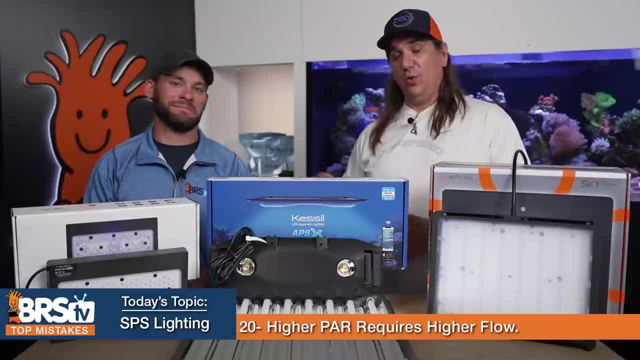 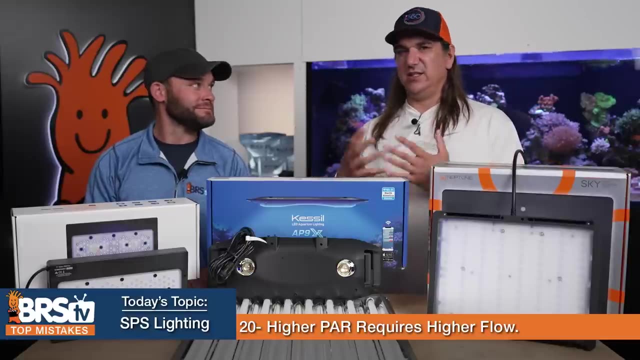 attempt to survive, I get rid of the zooxanthellae that is actually producing that energy. so the way that you can solve for that is actually high flow, and so high flow will actually allow uh, the coral to get rid of those oxidants easier. it increases the gas and water exchange in the 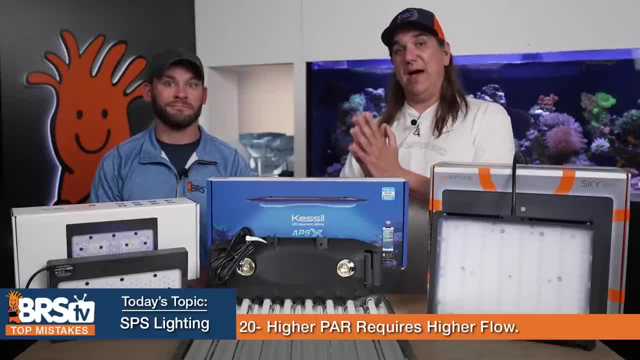 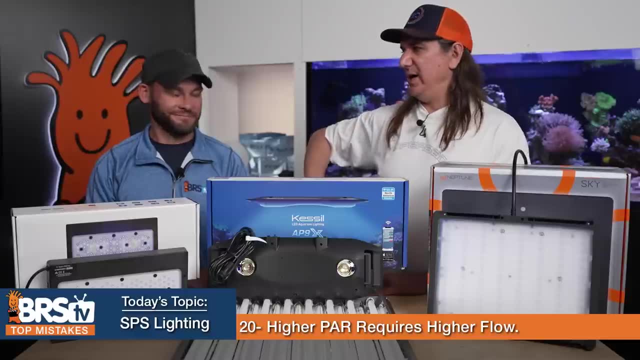 surface of the coral and the more flow you have, the better the corals will do in high par. so if you're gonna rise, ride that like razor's Edge of high par, ride the razor's Edge of high flow. and I'm going to tell you one more tip on the flow in that case, because it's super important, it doesn't. 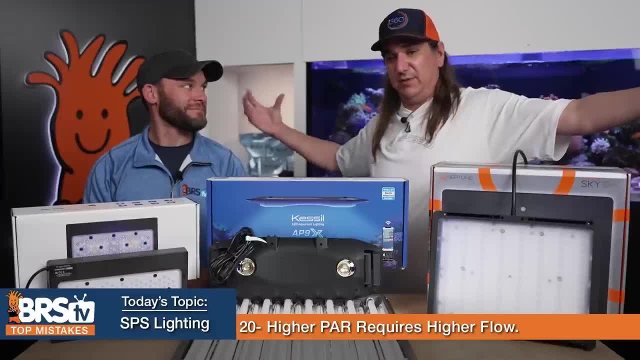 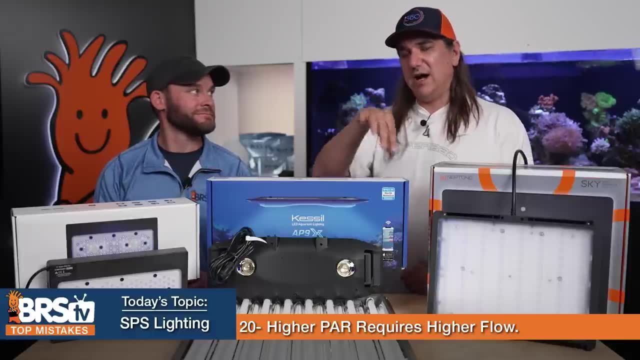 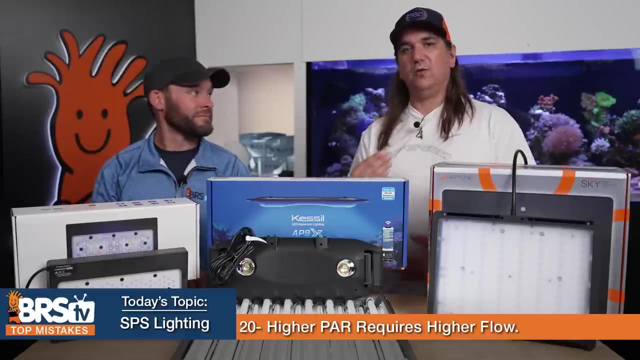 mean just put two ten thousand a gallon hour pumps on both sides, because when you look in the middle of your rock work you'll see that there's very little flow hidden by the aquascape. so what high flow actually means is go look for the dead spots or slow spots all over the tank and then solve for. 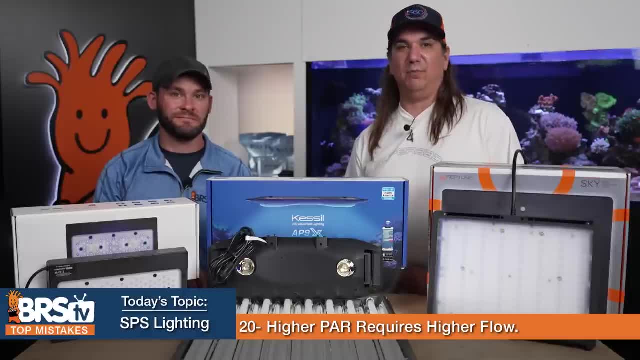 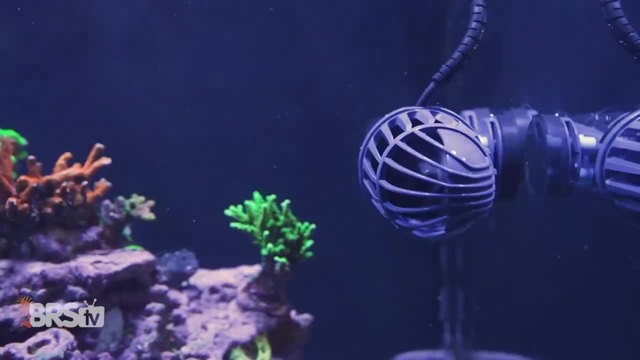 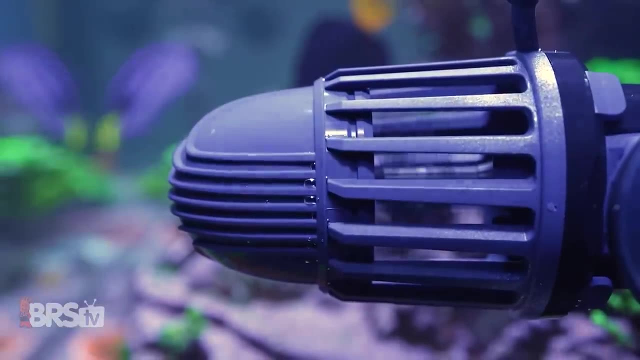 that flow don't get tied to a specific brand of pump, like I need to have all tunes, all Ecotech, all gyres and stay true to a brand. now look for the problem and the type of flow that actually solves it and you'll have better results: getting flow where it needs to be and kind of riding that. 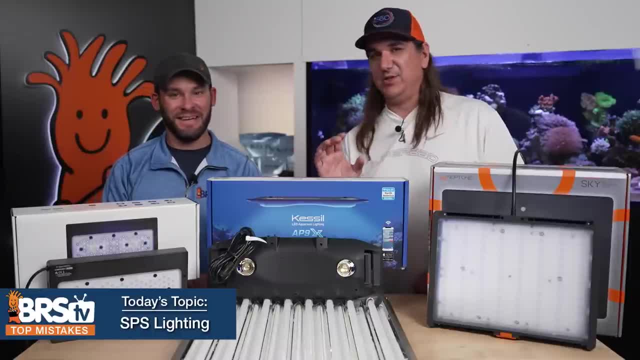 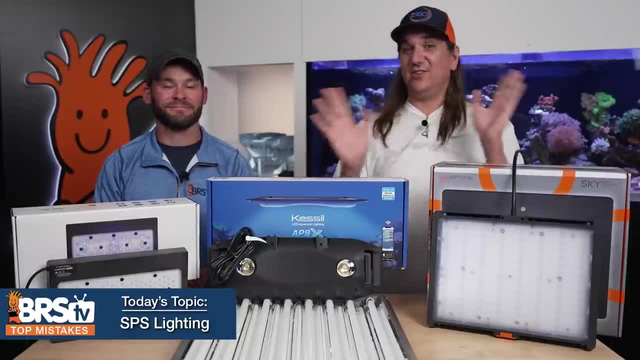 razor edge. all right, so hopefully you grasp the difference between little Frank big colony as well. as I'm part of the five percent trying to achieve something very unique versus the other 95, I need the information to apply as to my goals. you can find all this stuff here at the bulk Reef site. 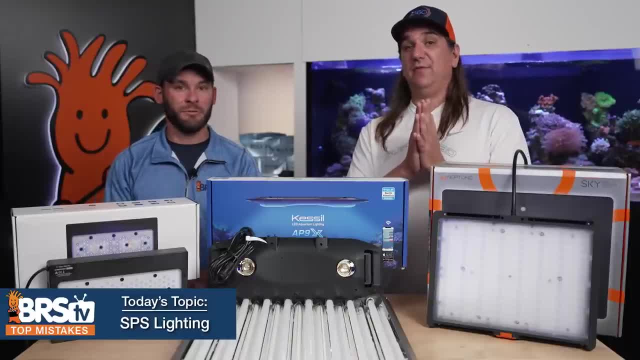 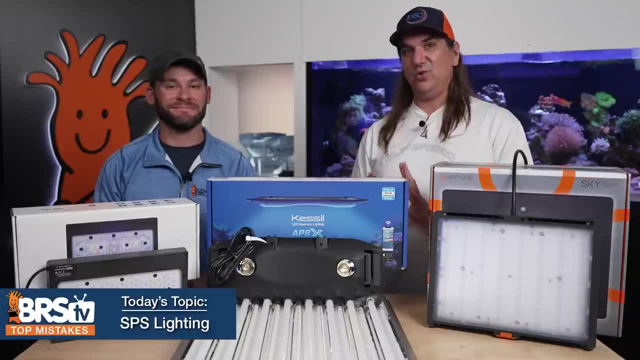 that you're looking for. but also we talked about flow. a lot of people believe that flow for SPS is actually more important- for the reasons that we just described, uh, than lighting. lighting, you nail it. flow is one of these constant tweaks you're always looking for.